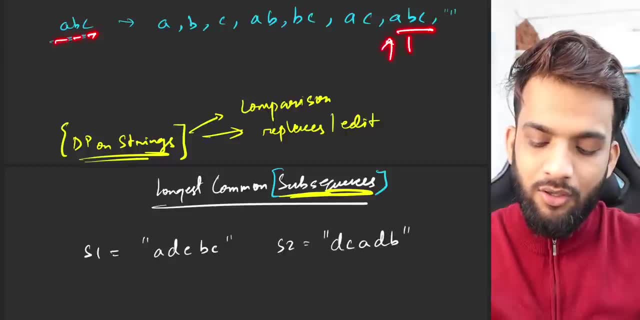 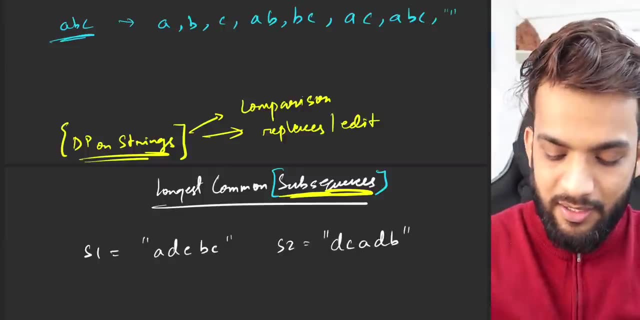 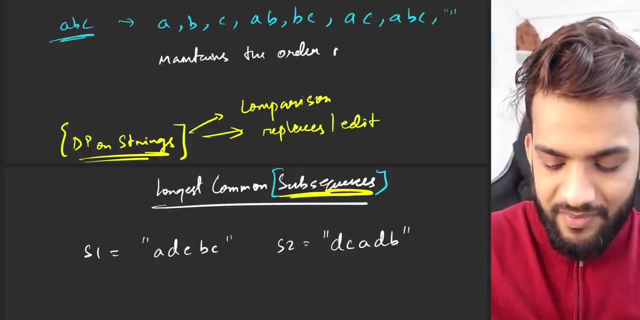 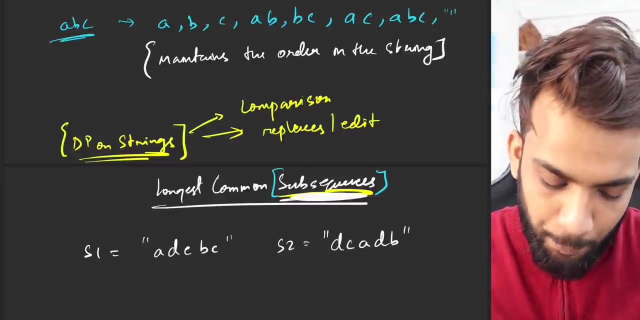 ABC is consecutive and maintaining the order Very simple. It can be consecutive. It cannot be consecutive. But as long as it maintains the order, maintains the order in the string, then you can call it as a subsequence right. And in order to print all these subsequences, you might be thinking 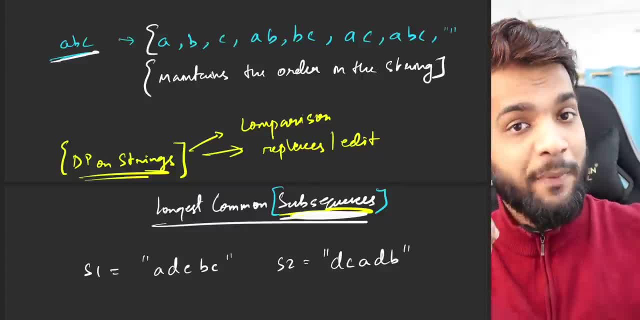 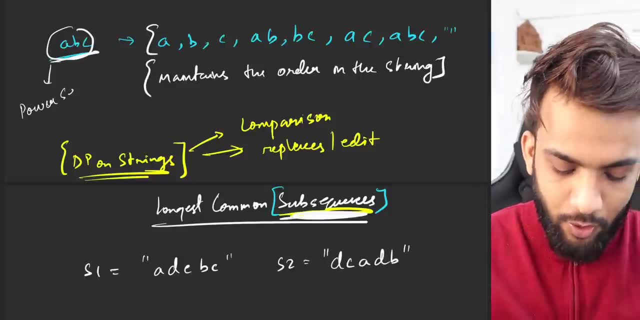 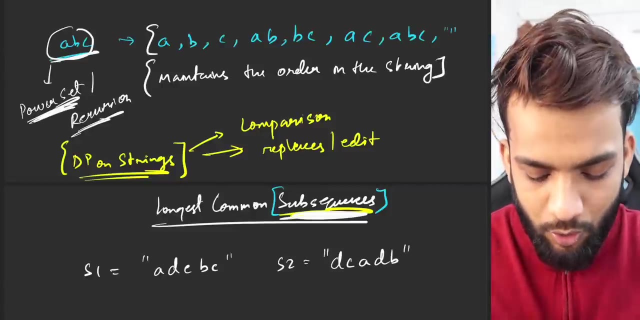 how do I print all the subsequences? So, in order to print all the subsequences, you can use either power set- I have a video on this- or you can use the recursion method. Again, I have a video on both of them And if you watch the video for any given string, 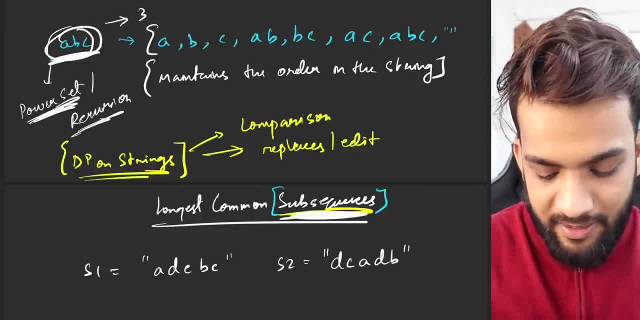 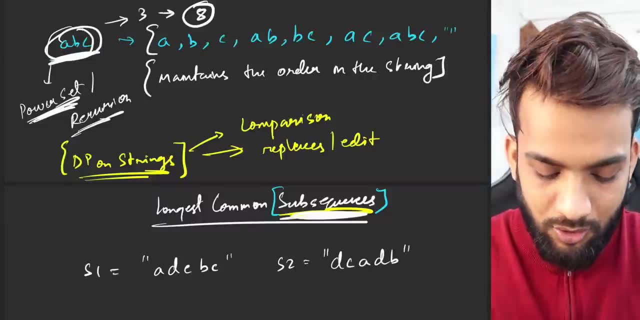 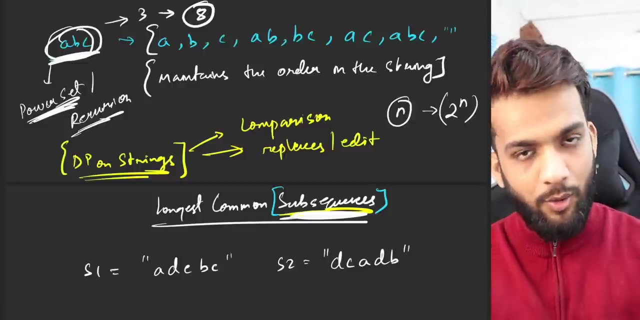 like this string is of a length 3, and the number of subsequences is 8, including the empty one where I say I do not pick any one. So for a string of length n, the number of subsequences is 2 to the power n. okay, So that is what subsequences mean. So what is longest common? 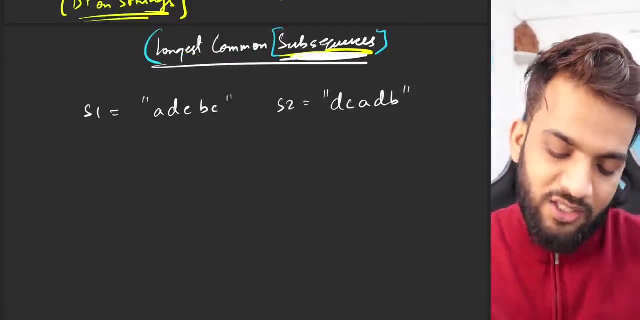 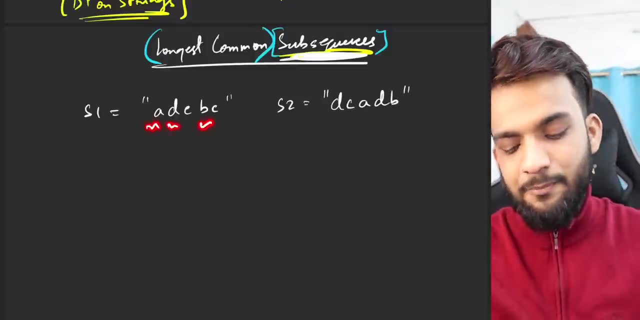 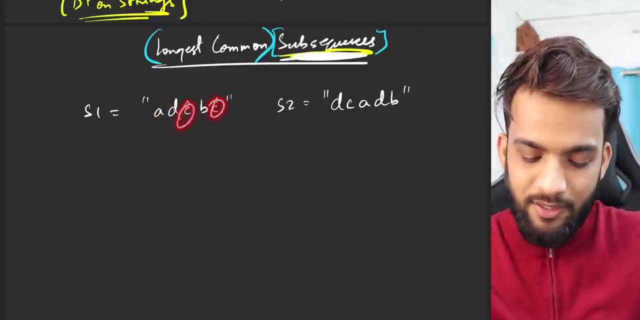 subsequence. What does this signify? What does this term signify? So I can say over here: A D, E is a subsequence. A D B is a subsequence. A E- C is a subsequence. D B- C is a subsequence. E C is a subsequence. 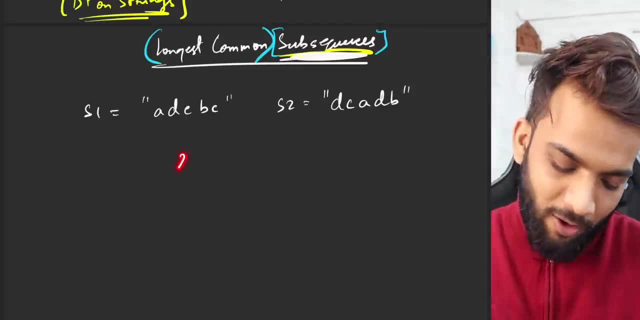 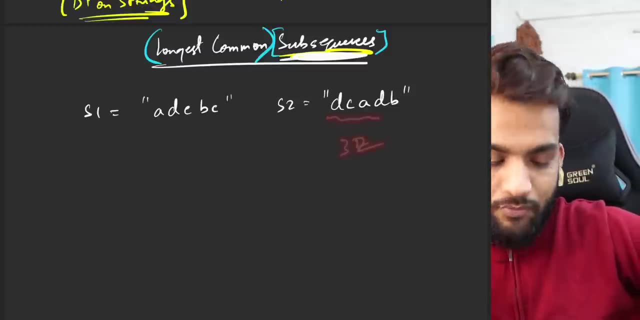 D, C is a subsequence. There can be 2 to the power, 5 subsequences, 32 different subsequences. Similarly, over here there can be 32 subsequences. okay, So I can say: this guy can generate. 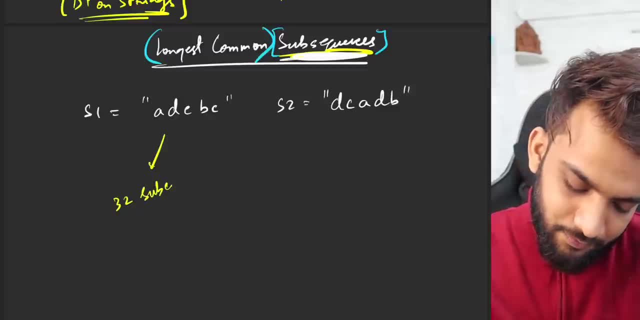 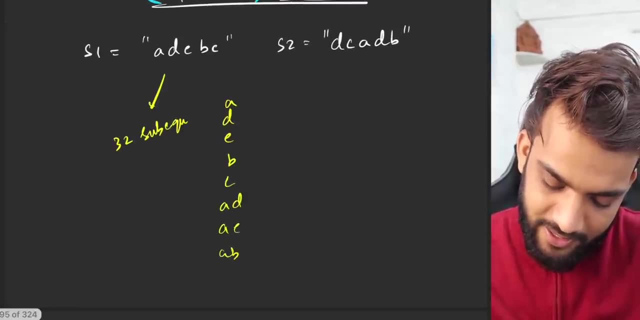 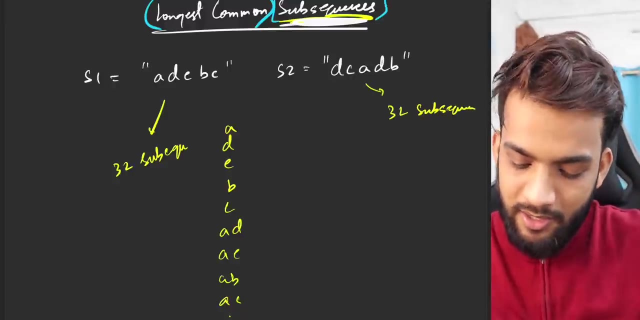 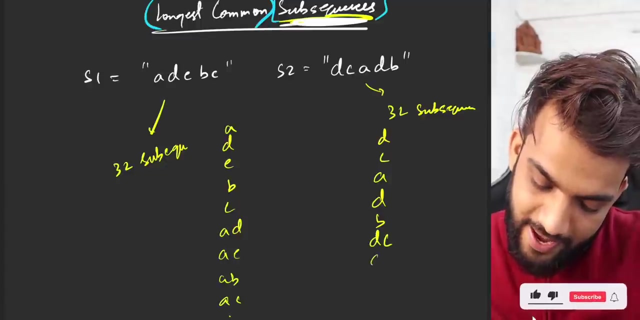 32 subsequences, Namely A, D, E, B, C, A, D, A, E, A, B, A, C, and so on. And this guy can also generate 32 subsequences correct, Namely D, C, A, D, B, D, C, D, C, D, A, D, D, D, B, and so on. 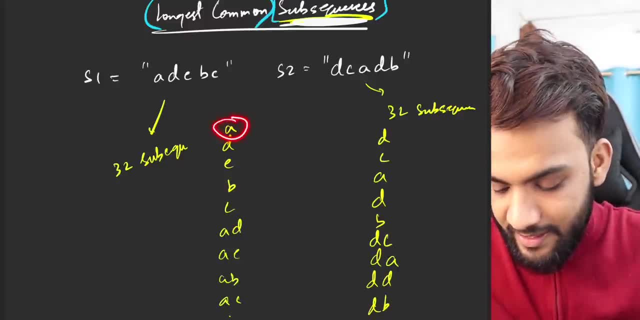 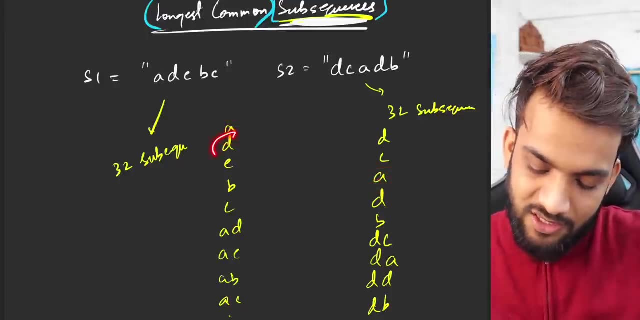 Now what you need to do is you need to take this A. does this A exist? Yes, So, as of now, the common subsequence, one of the common subsequences is A. Does D exist? Yes, One of the common subsequences is D. Does A D exist? No, So A D is not a. 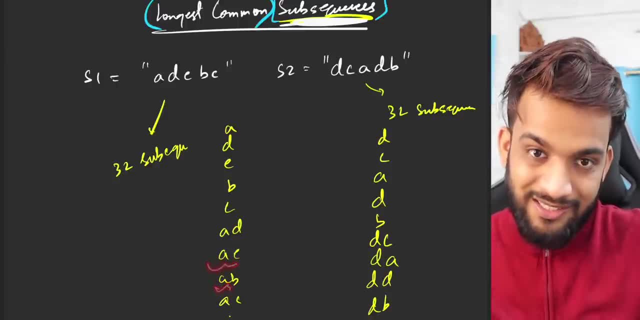 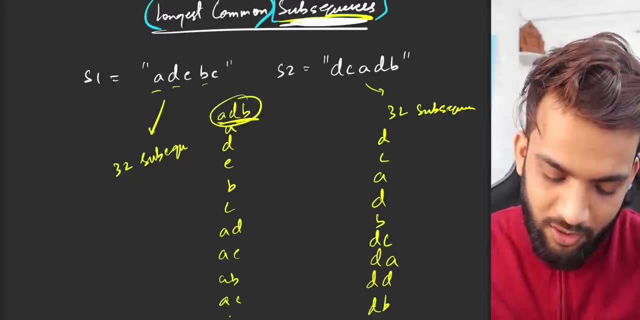 common subsequence: Does A C No? Does A B No? Similarly, you have to go on writing and you will see: A D B exists over here. A D B and A D B also exists over here, So you'll find. 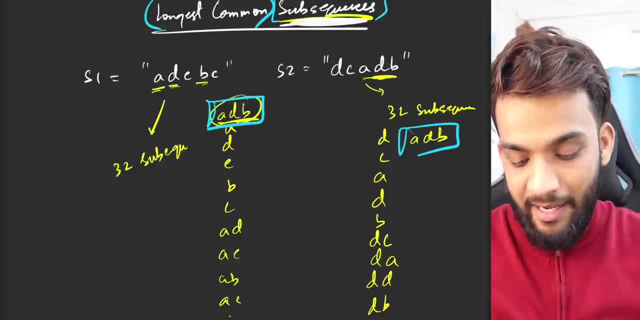 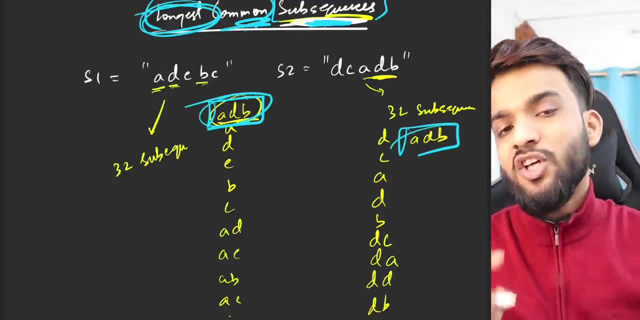 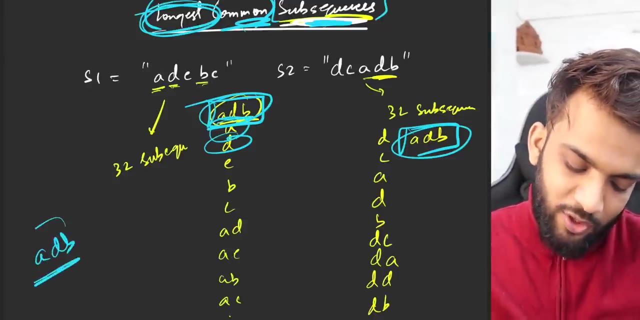 A D B is common in both of them And you have to find among all common subsequences which one is the longest. So A D B is the longest that you'll find. Yeah, there was A, there was D, but you need the longest. So the longest is A D B. And what is the length of? 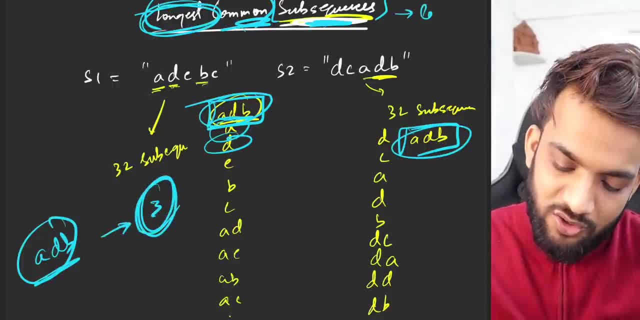 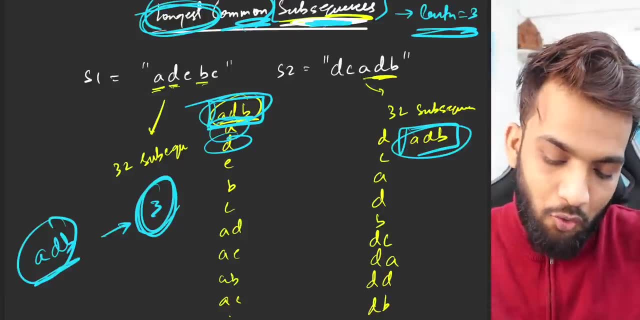 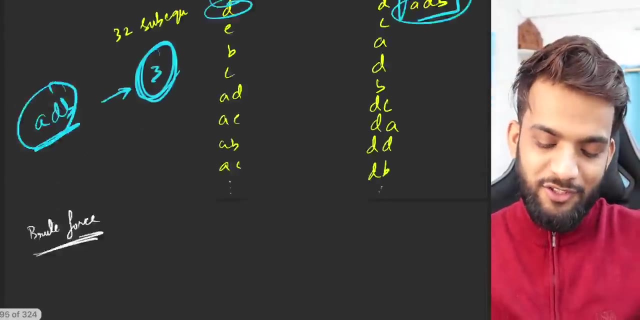 this Three. The length of this is three. So you need to tell me the length of this, which is three. So that's the question, Pretty straightforward. Now you might think let's apply brute force. Okay, that's correct. What is the brute force? Generate all the 32. 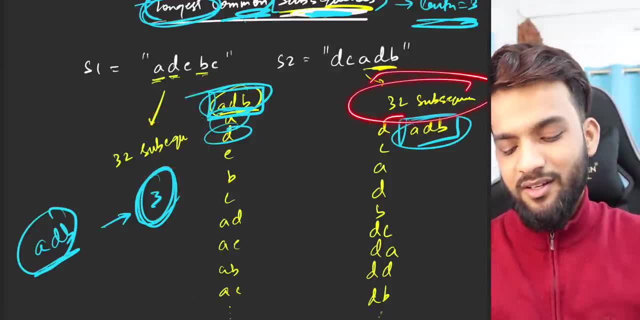 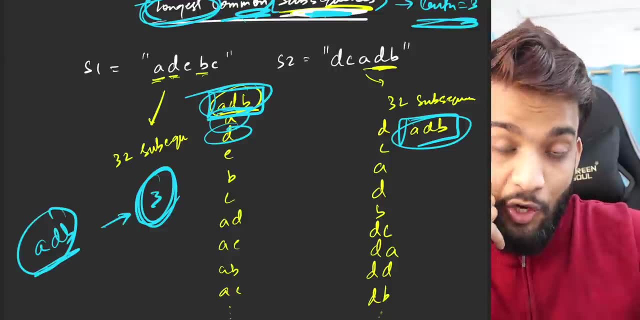 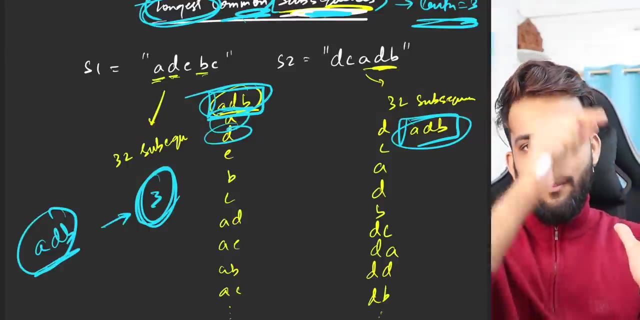 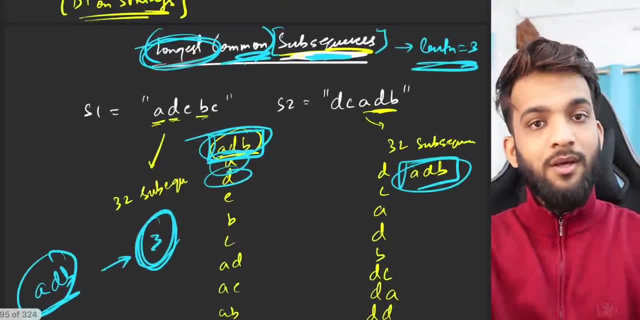 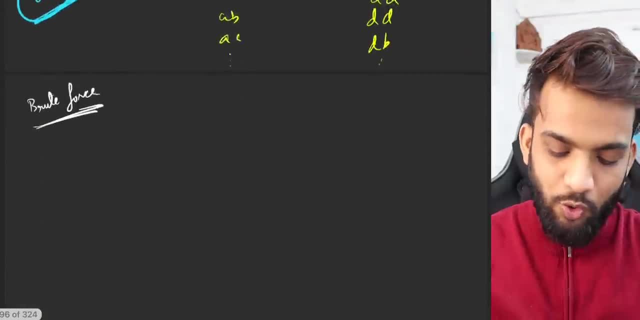 take one, compare and get the longest Among them. So that's going to be true to the power n, because you have to generate all of the subsequences exponential in nature. So the brute force is going to be exponential in nature. 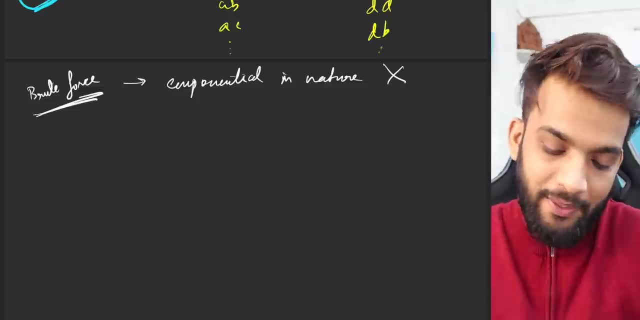 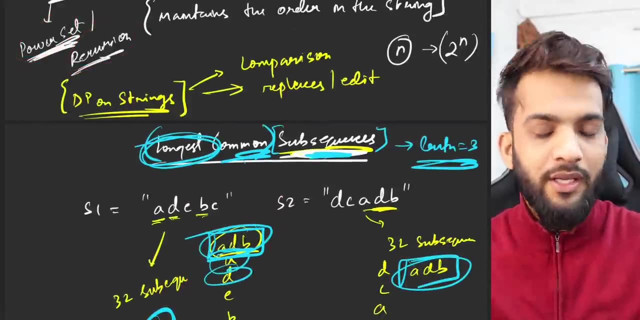 Hence a pattern that I will not follow. But yeah, if you want to generate all the subsequences, feel free to watch out the power set video or the recursion video that I will be leaving the link in the description. Okay, so if not brute force, then what? 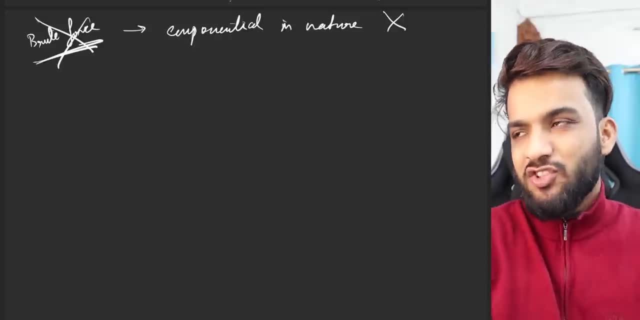 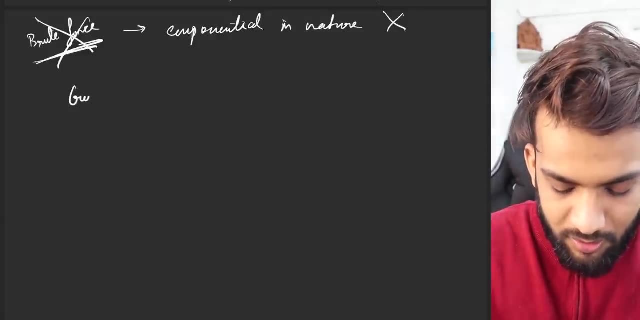 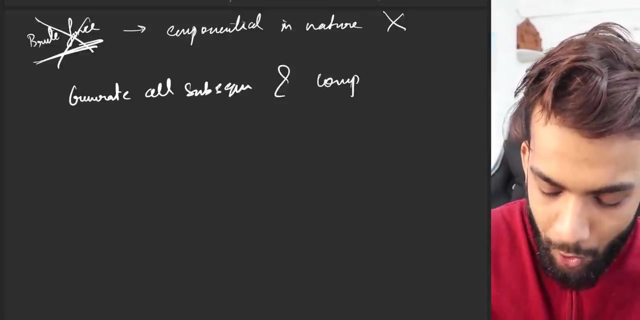 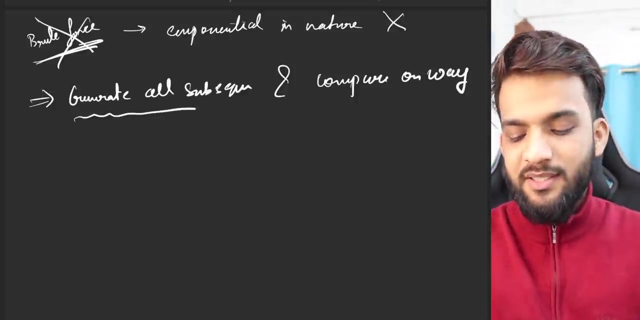 Then my brain says, okay, let's do some. let's generate all the subsequences and try to do comparisons. Okay, Generate. that's what we did: Generate all subsequences and compare on. way, That's what I'll think And that's a standard way, Like you have to generate all subsequences. 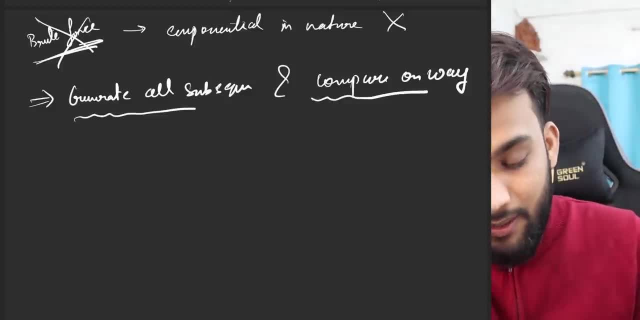 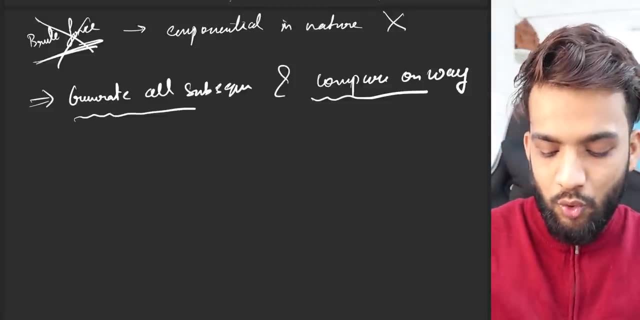 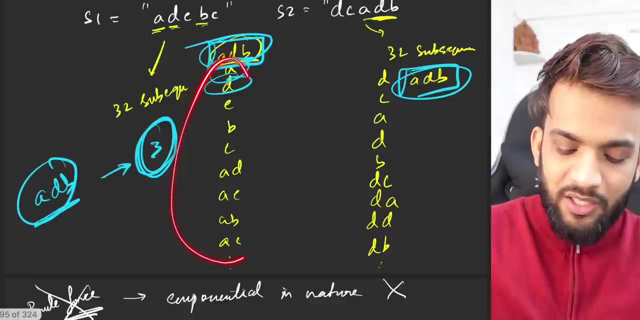 and compare on way. That's a standard, standard way that we generically do in uh recursion or like and on DP on strings. I'll be telling you about that. So you will be tending to follow a recursion method where you will not generate these. Instead of that, you will. 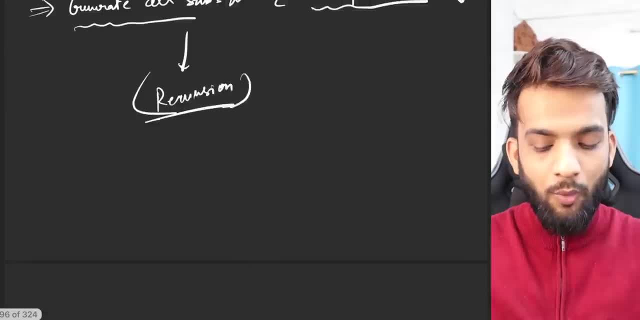 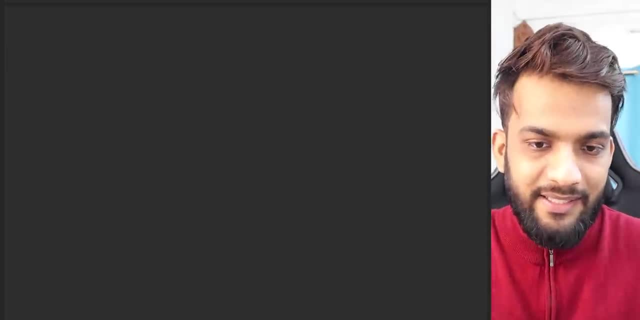 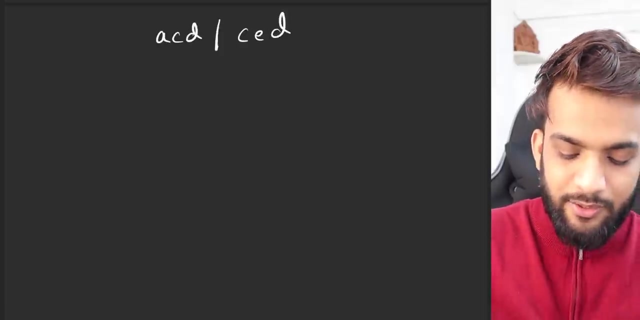 use parameters to generate them. I'll be showing you how. So first let's understand something in deep learning. Let's take an example super quickly. Uh, ACD and CED. Okay, Assume these are the two strings that you're looking to solve, ACD and CED- Okay. Now if you go to generate 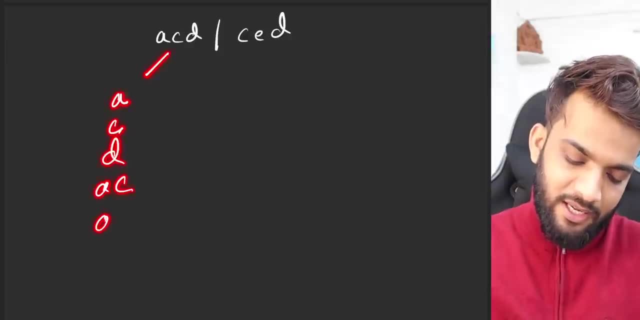 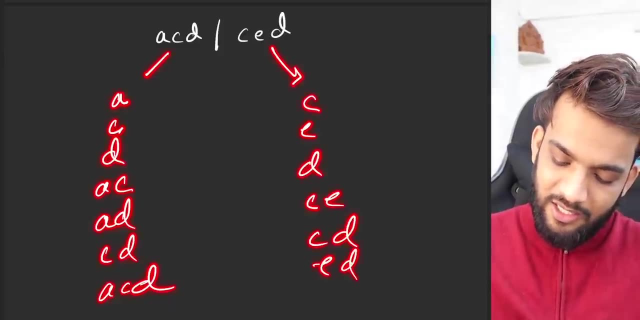 all the substrings will be ACD, AC, AD, CD, ACD, and over here it will be CED, CE, CD and ED, CED. Then you figure out, the longest being CD and CD. So thereby this is the longest, which is of length. 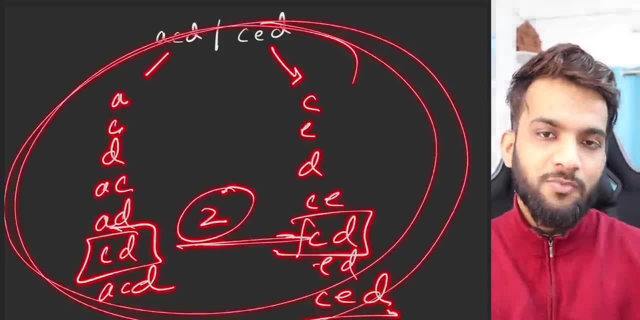 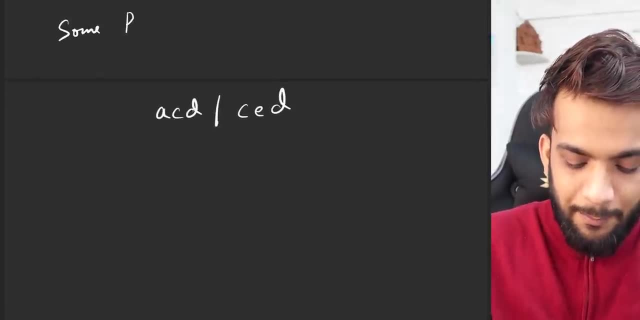 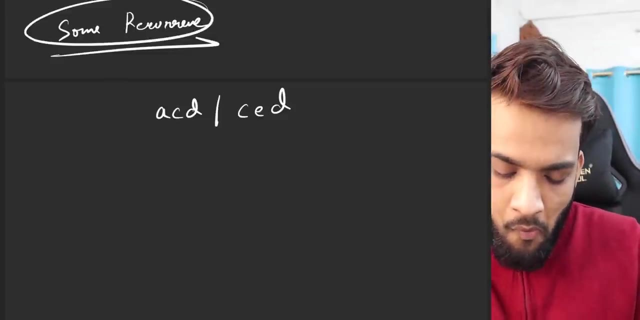 two. But if you generate this, that doesn't make sense. That's where we will try to write some recurrence. We'll try to write some recurrence. that probably gives me the answer through the way. Through the way is my question. Okay, So assume you're solving this entire portion, this entire string and entire string, Okay. 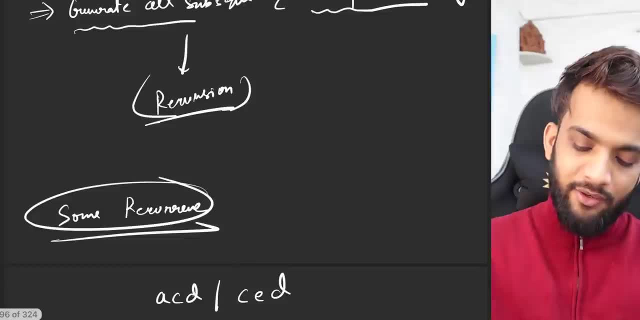 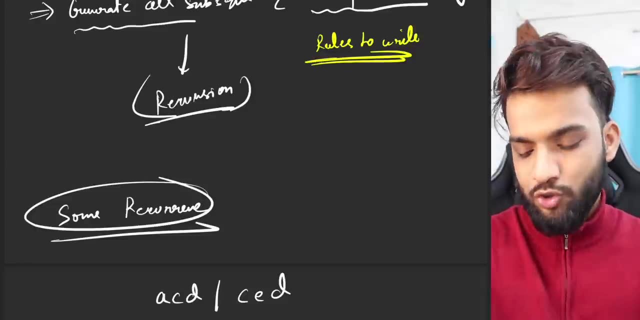 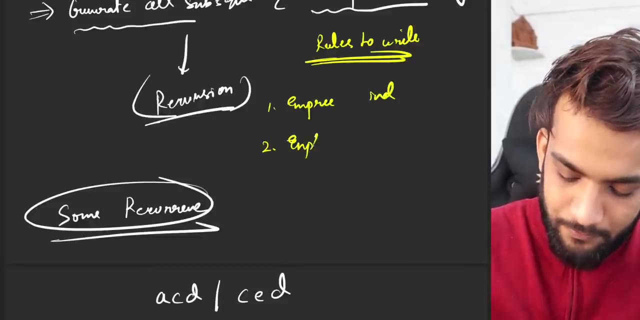 And generically, generically, what are the rules to write the recurrence? Let's, let's quickly just jot down the rules to write recurrence And then we will try to follow those paths: Express everything in terms of indexes, Explore possibility on that index, That's it. 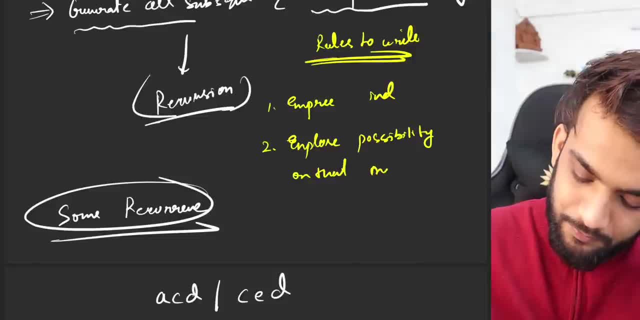 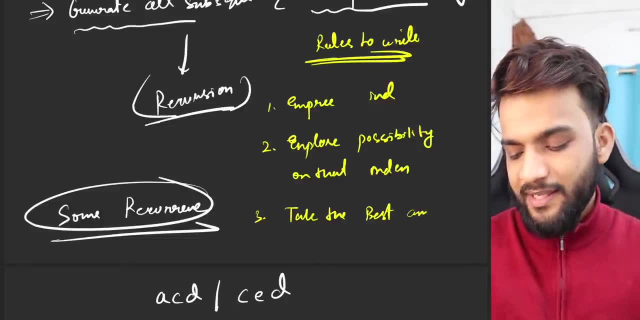 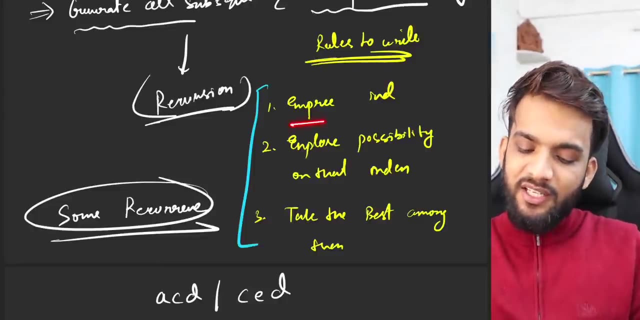 Explore possibility on that index is what we do. Take the best among them because you're looking for longest. Take the best among them. These are the three rules that you generically follow. Now express everything in terms of index. Okay, So either you can write it in terms of index or you can write it in terms of index. 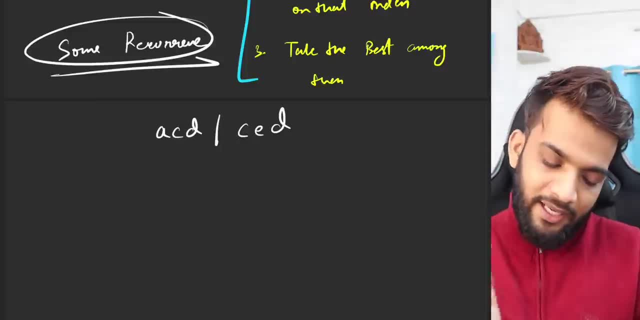 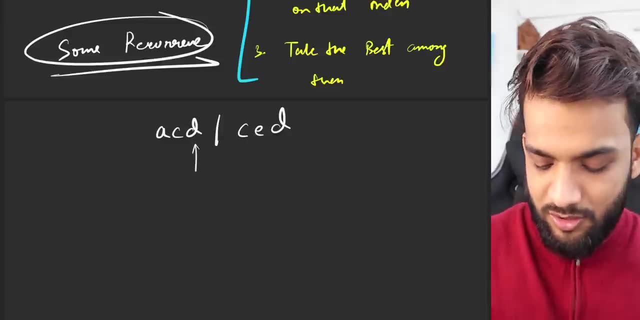 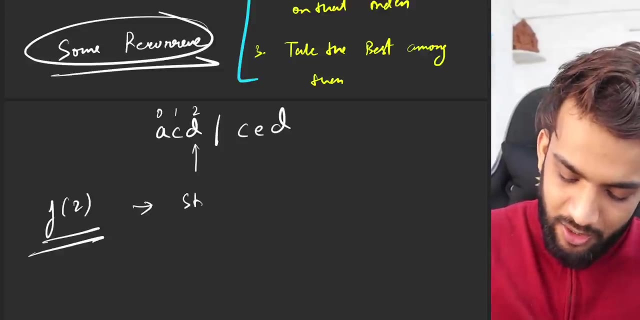 You can carry this entire string or you can say: hey, listen, probably I can have a pointer here. Let's understand: Probably I can have a pointer here which is somewhere around index two, and F of two signifies the string till index two. Okay, Probably you can say: 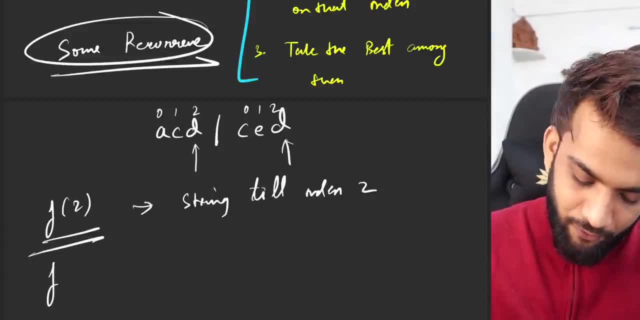 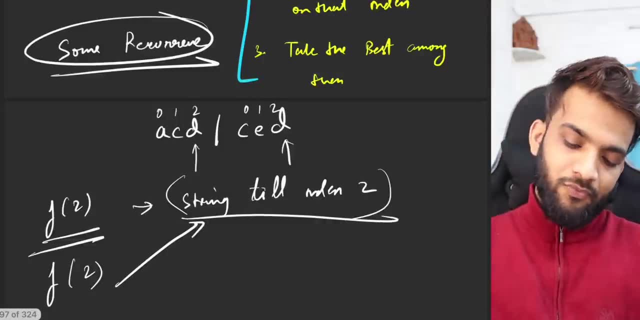 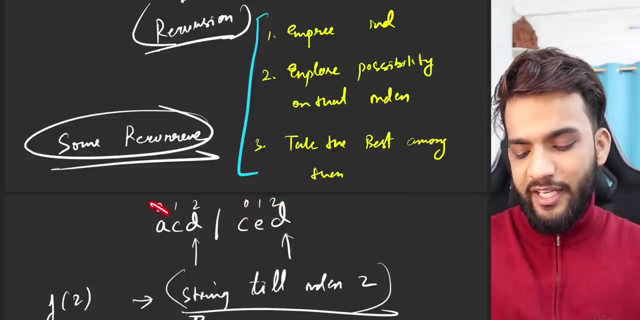 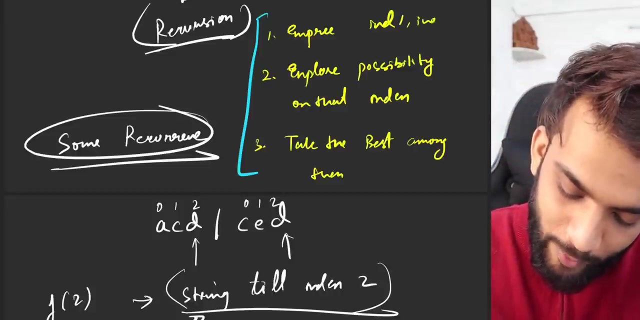 I can keep a pointer here, which is again index two. F of two again signifies the string till index two. Something to observe: A single index cannot express both the strings. A single index cannot express both the strings. Thereby I will have to represent them by two indexes. 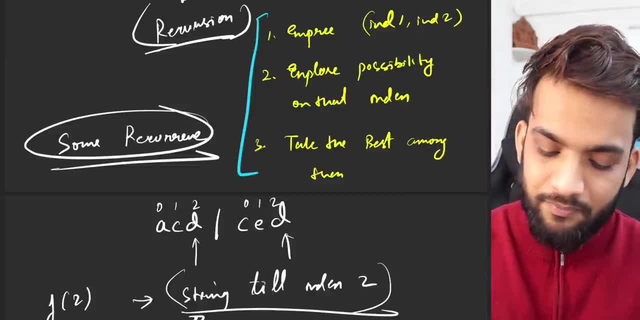 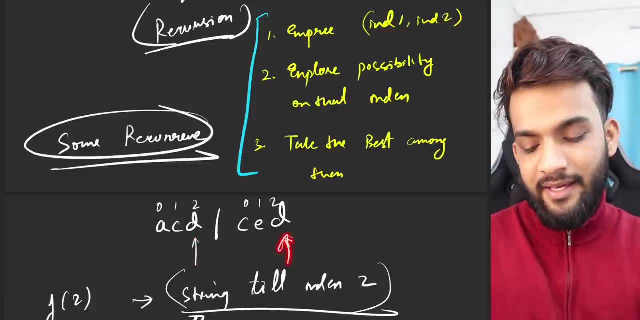 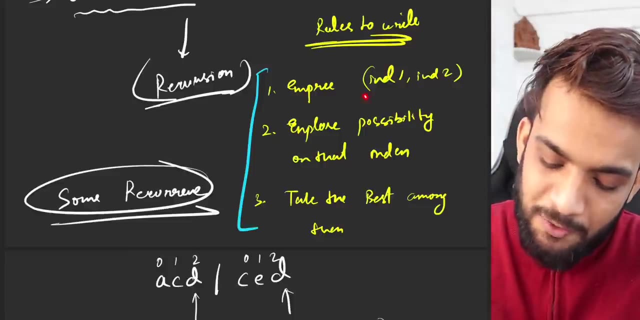 I have to represent them by two indexes. where index one represents this guy, Index two represents this guy. That's the first Modification that you have to do in the rules. Since you're dealing with a couple of strings, you express them in terms of index one and index two. Very simple, Like in all the array problems. 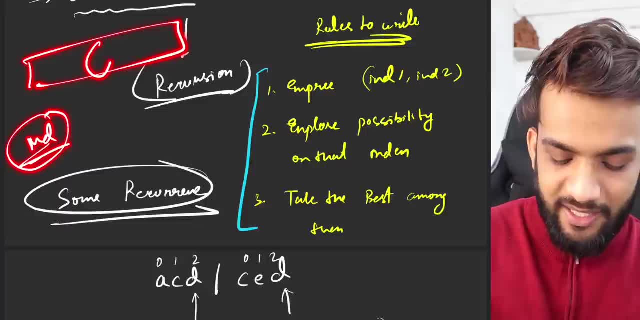 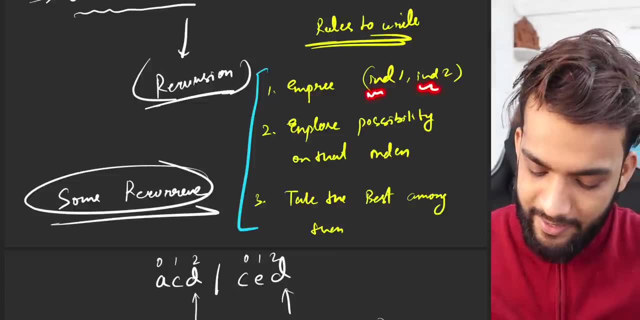 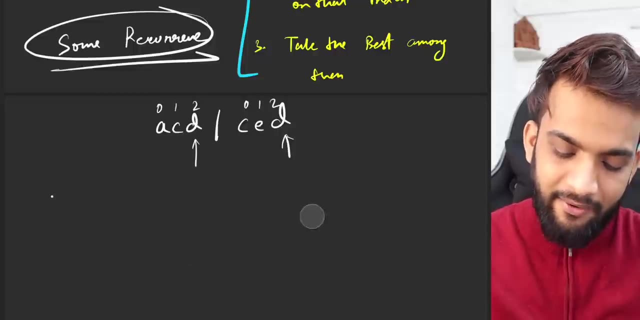 you express everything in terms of index, because there was an index, Then you decided to pick, not pick or similar kind of things you did. Over here we will have index one and index two, which we'll be representing. So can I say, if I omit this and I write this something? 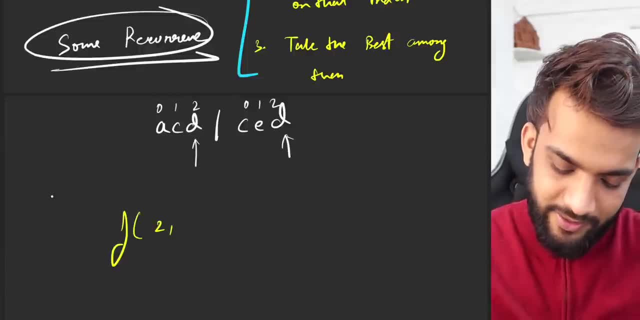 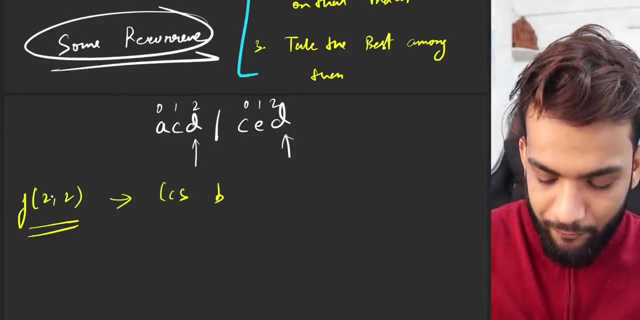 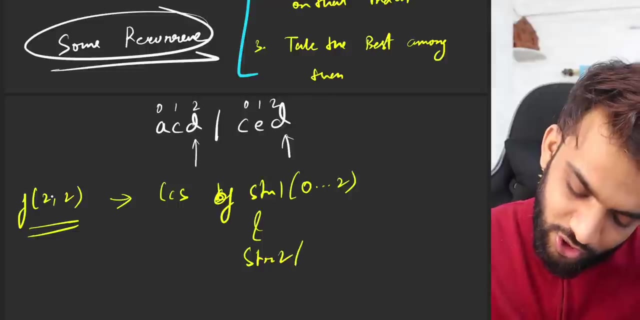 I can say f of two comma two. rather, let's write it in a smaller way- F of two comma two. what does this represent? Tell me the LCS of string zero to two, string one zero to two and string two zero to two. This is what this f of two, two will represent. So we have understood. 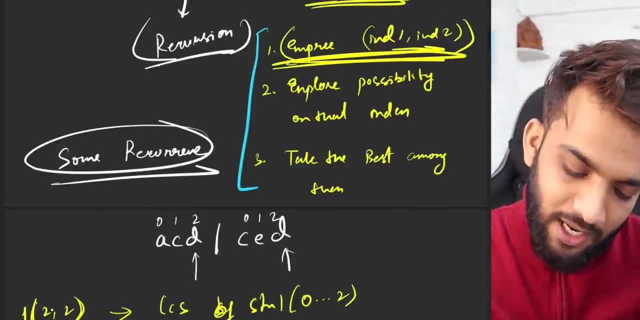 the expressing term. We have understood the expressing term. That's done. If I'm writing something as f of, Let's say f of two comma two, Let's write it in a smaller way. Let's write it in a smaller way. 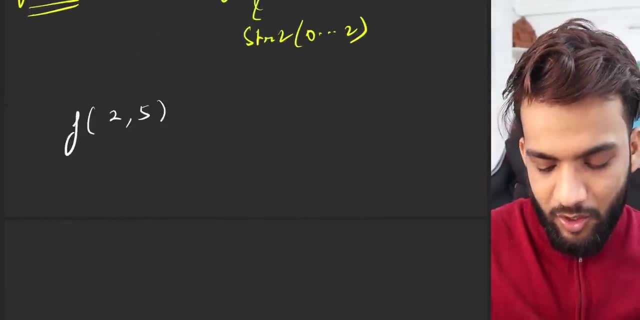 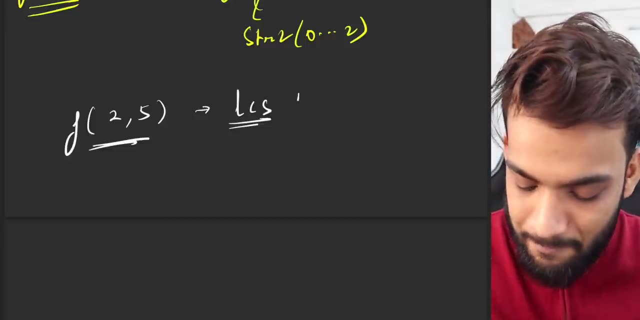 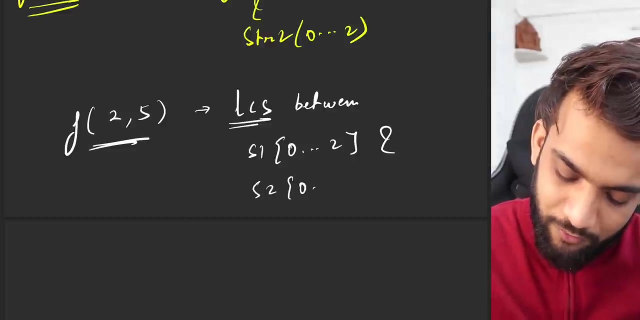 Let's say two and five. What does this signify? This signifies: give me the longest common subsequence between string s1, zero to two, and string s2, zero to five, A smaller string and a larger string. This signifies this, So I hope you have got an idea what I'm meaning to. 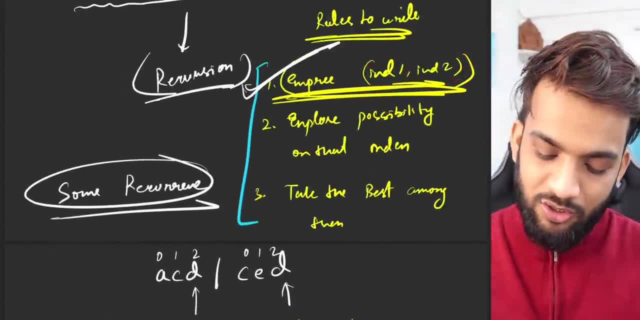 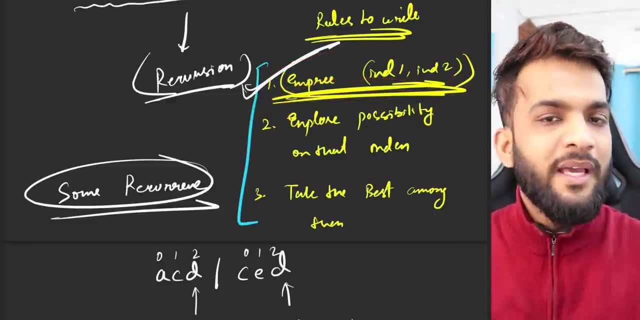 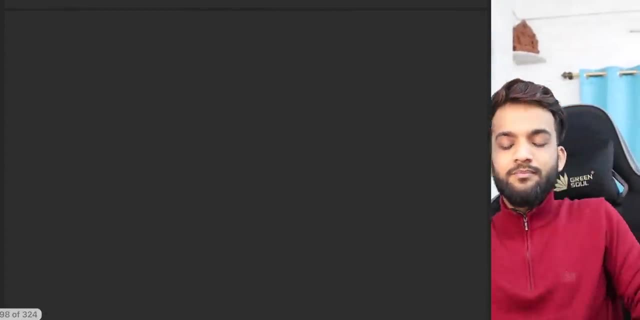 say, by index one and index two. So this we have figured out. Now time to explore all possibilities, because if you do not explore all possibilities we will be having an issue. Okay, so let's try to explore all possibilities. Okay, let's try to write them. 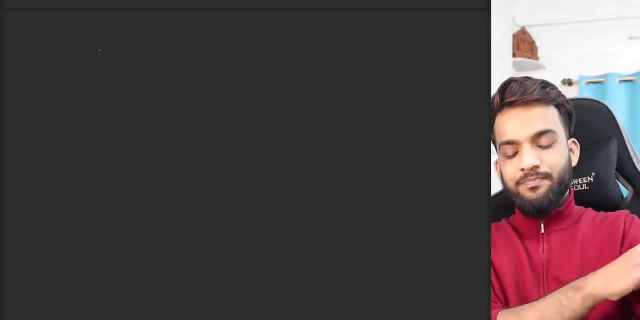 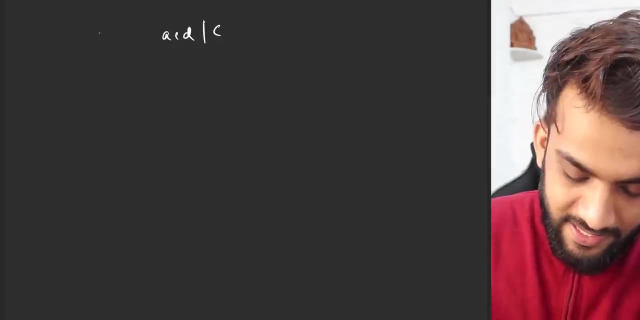 So can I say this? Can I say this? Okay, let's try. I'm having the string ACD and CED and I'm having a couple of pointers over here, And this is index one and this is index two. So a very straightforward question is if they're 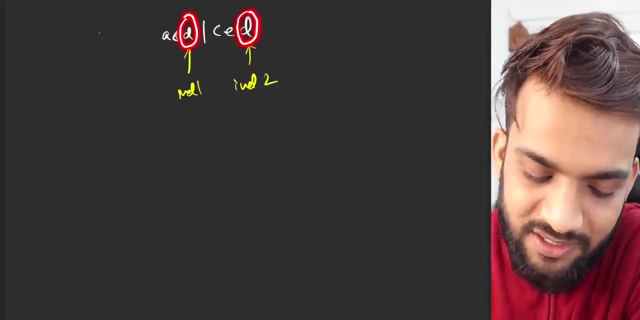 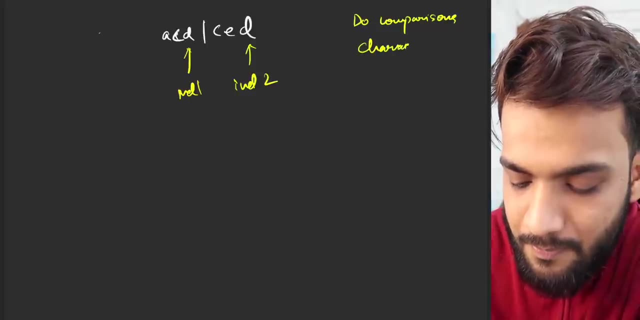 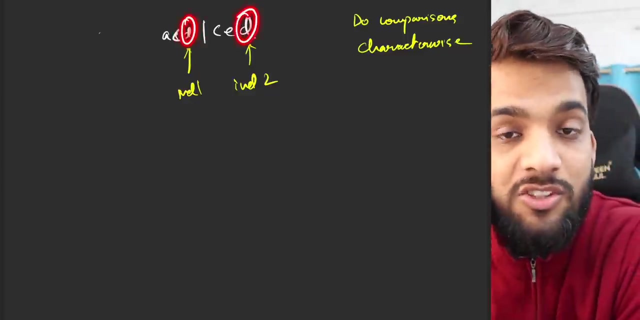 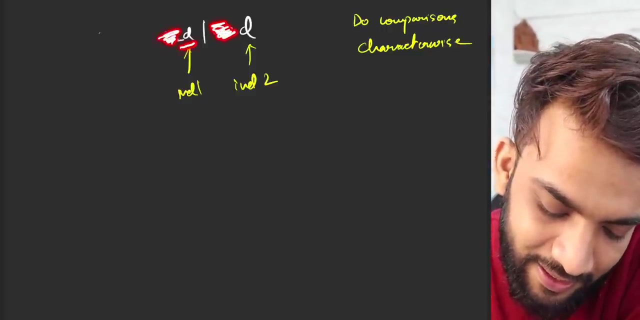 matching because this D, like do comparisons characterize, Remember this, Do comparisons characterize. So this D and this D is matching. That's something we can see. This D and this D is matching. So can I say, If I just do not think of these things, and this D and this D is matching, Can I say I got a. 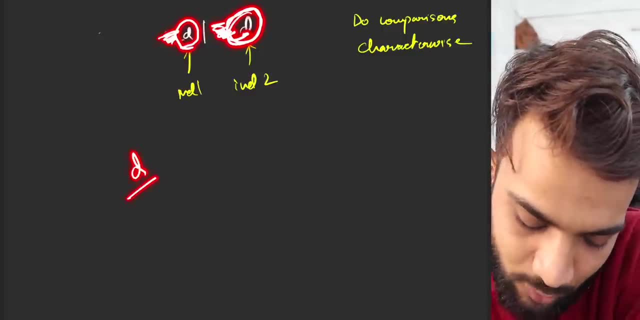 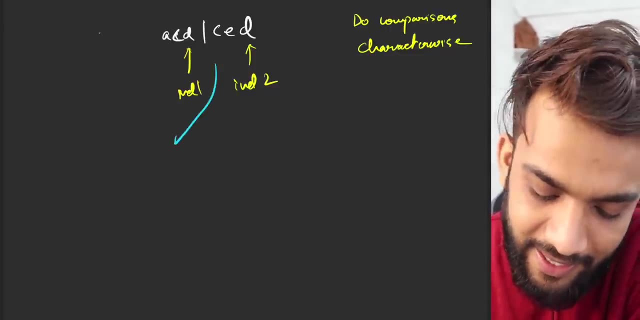 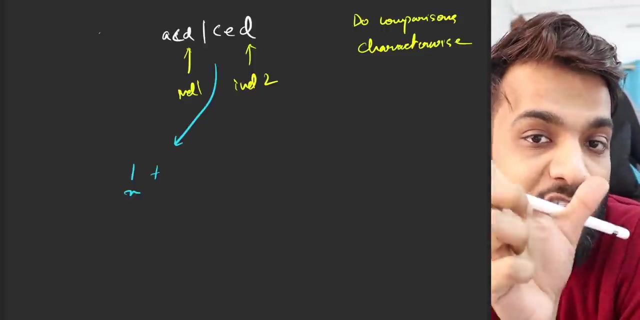 subsequence of length one. I got a subsequence of length one that is D, which is common in both of them. Again, makes sense. Thereby I can probably say one of the possibilities that I can have is: I got one subsequence of length and then I shrink the string. Then I shrink the string and say 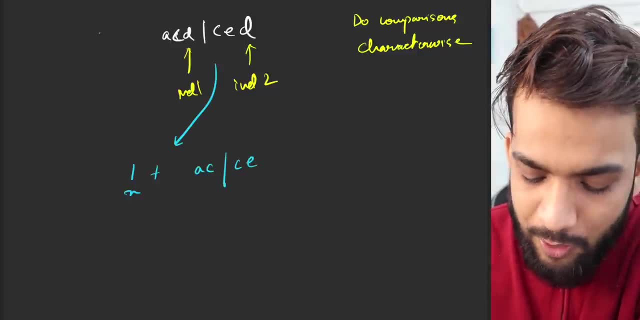 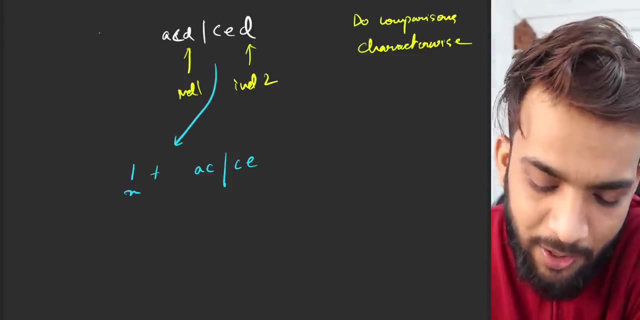 the new string is AC and CE, In which probably you can find an answer. In which you can probably find an answer. So does that make sense? It does, Because if these guys are matching now you just have to take these two strings and you've to ask them. 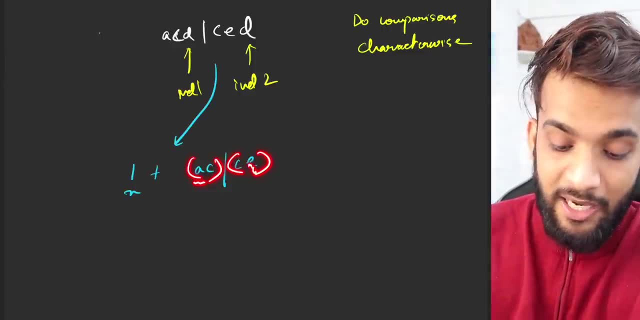 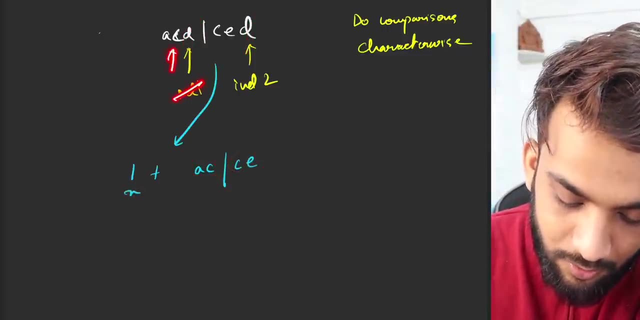 what's the common, What's the longest common in them? Because I've done for D, which is one. What is AC? I said what is AC. This index will come here, which is index one. So I can say AC is index one over here. 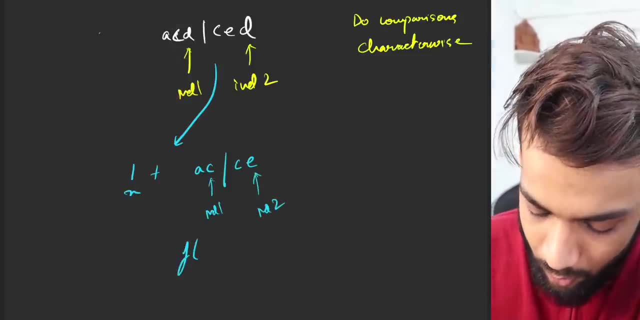 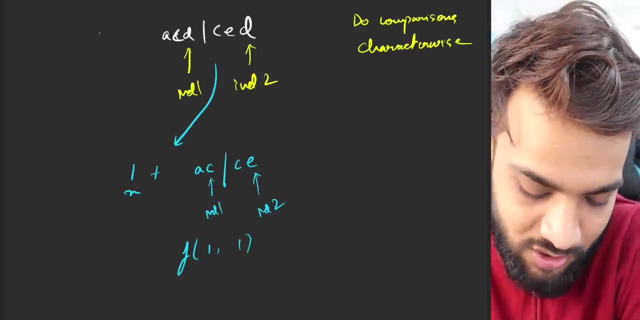 CE is CED is index 2 over here, which is nothing but f of 1 comma 1, f of 1 comma 1. why f of 1 comma 1? very simple, because 1 for this t and i've shrink the string. this is the string, so that's f of 1. 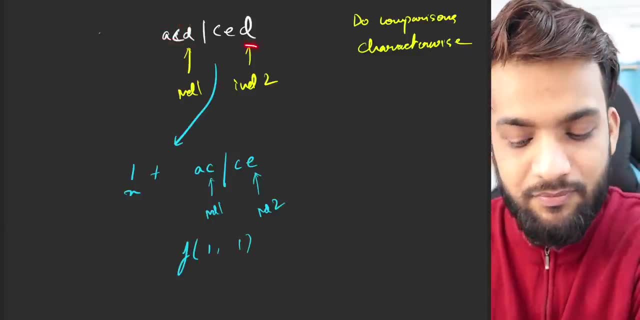 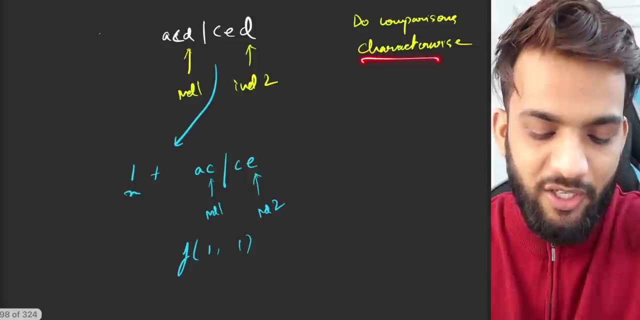 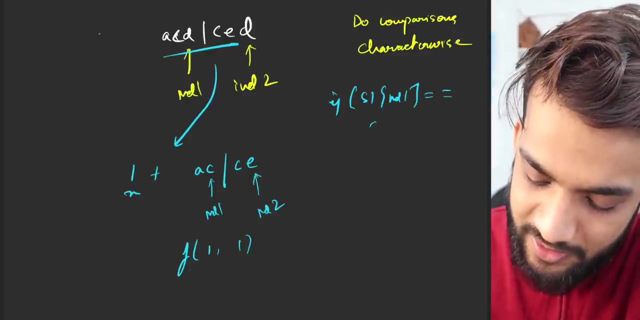 which means 0 to 1 is the string and this d you took. so again 0 to 1, so f of another 1 is there. that's how you can do it if they are matching. so if character matches, index 1 matches with index 2, can i write this as: 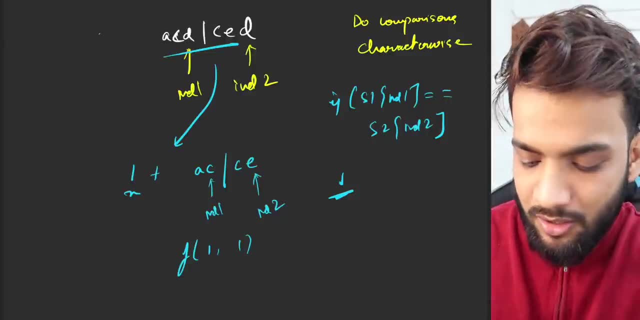 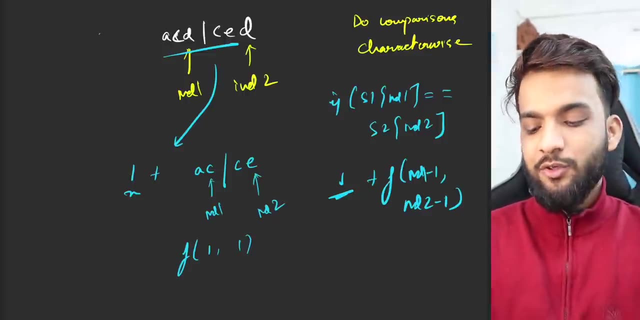 i will add 1 to the answer and i will reduce index by 1 and the other index by 1 as well. can i see this? i'll reduce index 1 by 1 and index 2 by 1 as well, and this is going to be the. 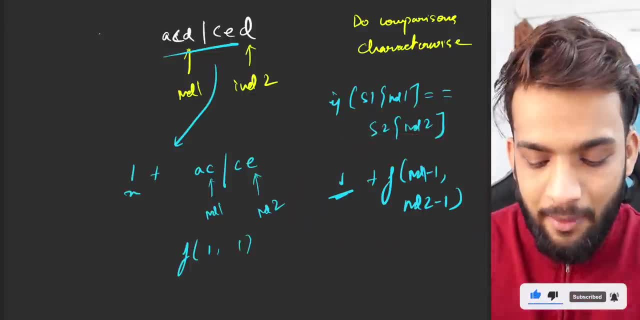 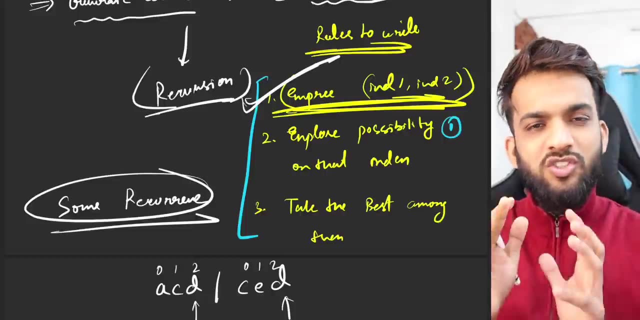 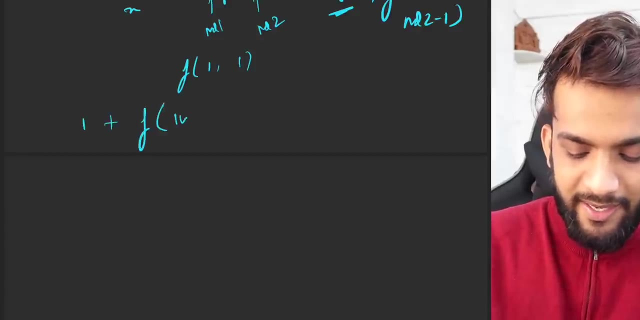 recurrence if you both of the guys are matching. okay, so we have. we have probably done one possibility, you've done one possibility over here, which is if both of them are matching, then it's kind of very simple enough. you say one plus f of index, one minus one index, two minus one, and that's going to be the. 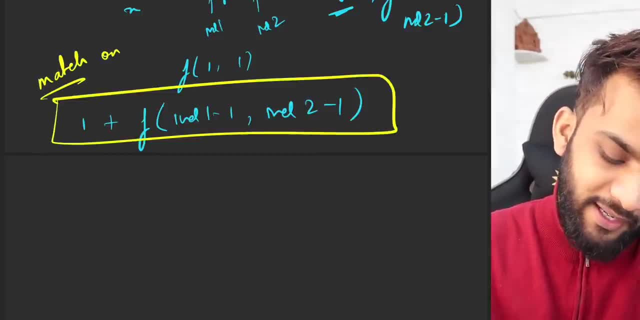 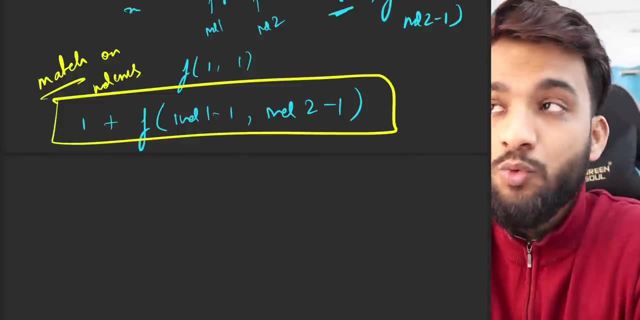 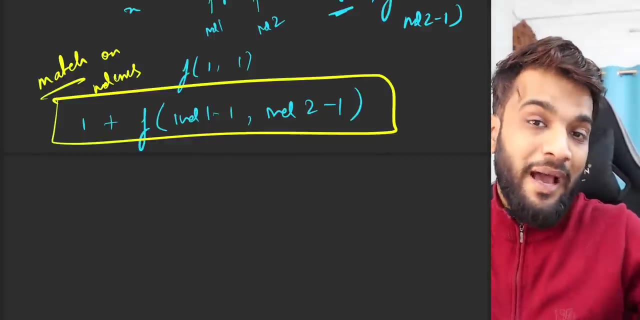 case, if match on indexes, if match on indexes, that's one possibility. okay, now what about the other possibility? because what if they do not match? because in all the string problems you'll, in all the comparison of string problems, you'll see match and not match, match and not match in. 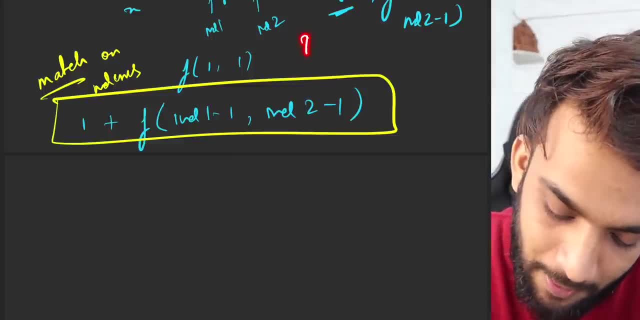 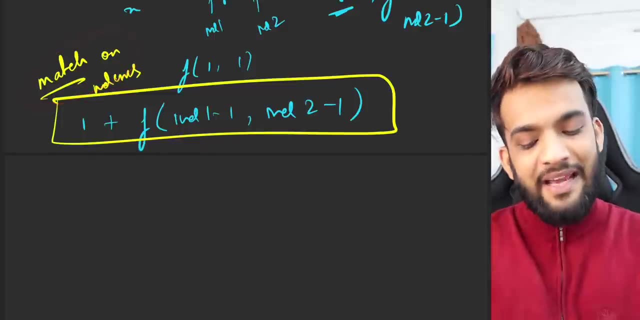 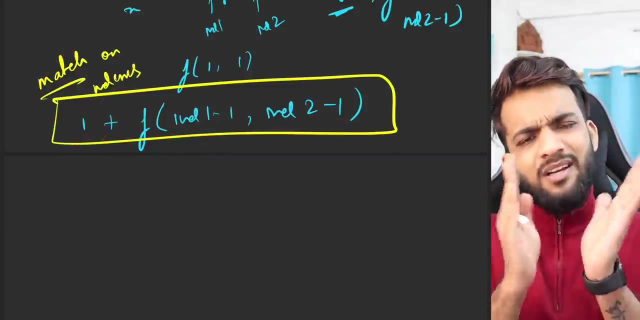 previous problems of arrays it was it was pick, not pick. over here it will be match not match. so for match is, you will generally add to the answer and it will move back by index. in matches you'll generally add the answer and move back by index. similar to pick. similar to pick when you moved one. 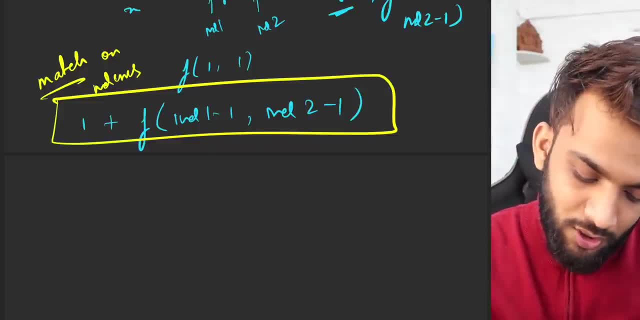 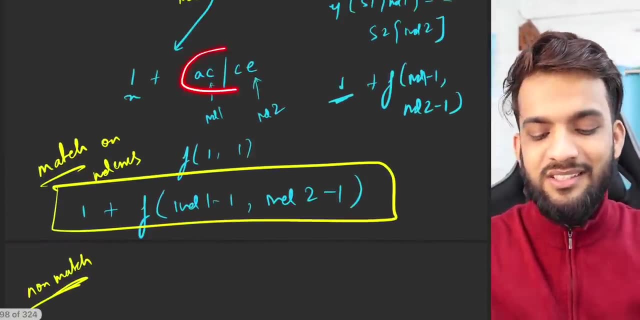 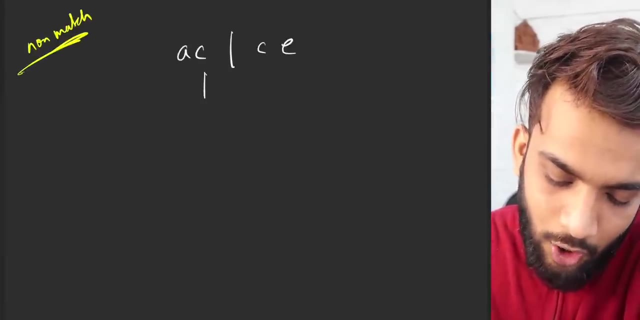 back, one back, okay. so what about non-match? let's talk about non-match. what if they're not matching? yes, what if they're not matching? because in the next step it will be ac and ce. what if they are not matching? let's see if i have ac and ce and they are not matching, something i know for sure. 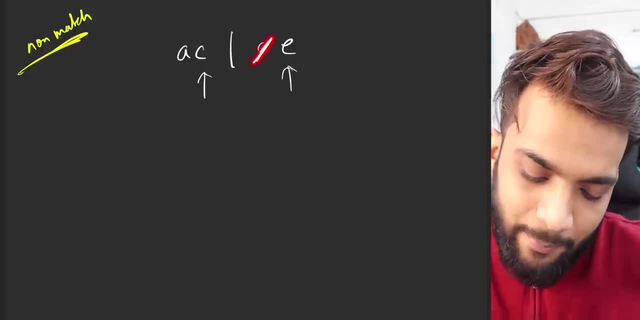 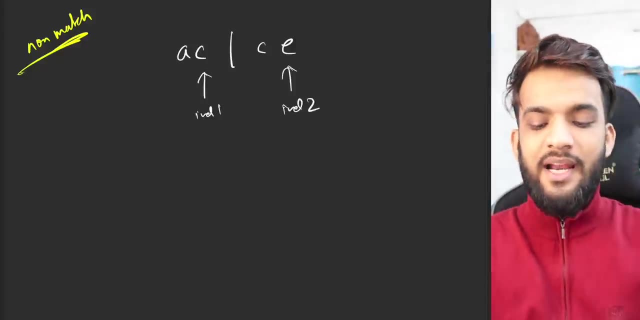 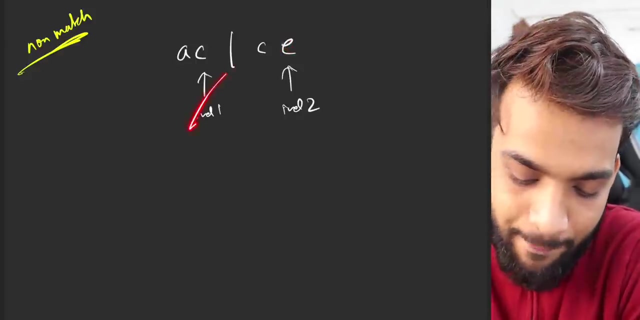 is, if i go ahead, this c will match with the c, but as of now, my index one is standing here, my index two is standing here. so how will i go and compare this c and c? because as of now i'm standing at e. if i move them both back, i will miss out on a comparison of c. i'll miss out on a comparison. 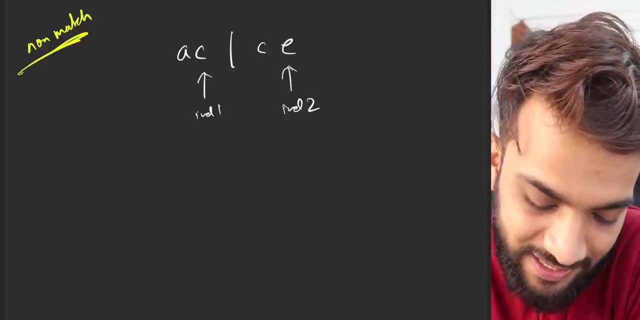 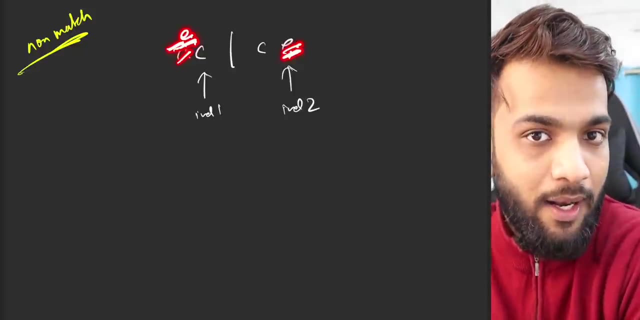 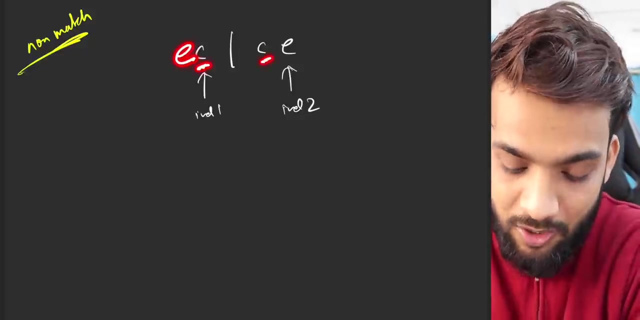 of c, right, or what if there was an e here? so this e would have matched with the c, so i can also miss out on the comparison of e as well. you understand, if i write ec, then what will happen? this c and this c might match because they're standing in the other places. or this e? 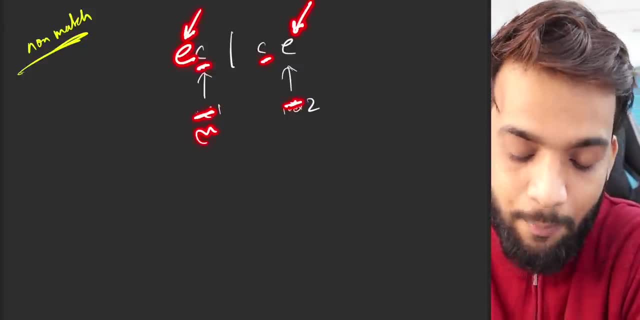 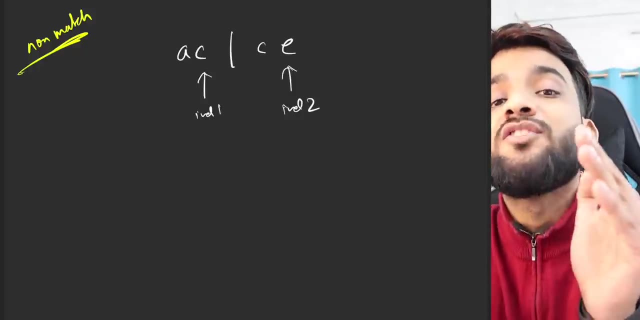 and this e might might not match any day, because they're standing at opposite, standing at different places. thereby you have to apply your brain, hearing you. thereby you have to apply your brain in such a way that you explore both the possibilities. yes, what are the? both the possibilities? 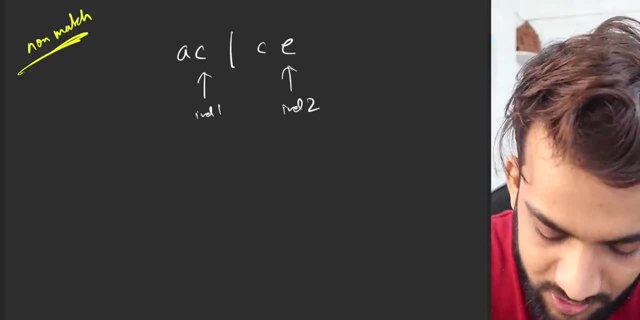 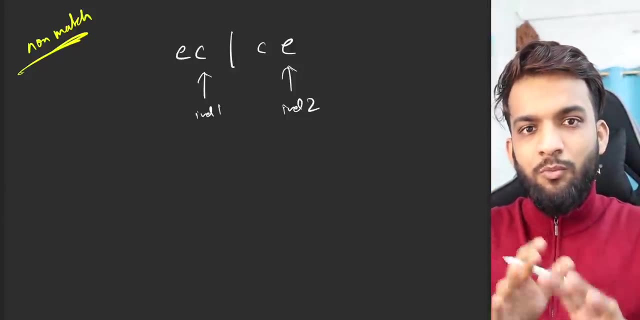 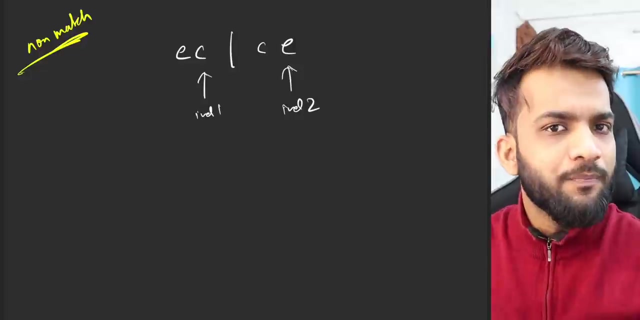 you say, hey, listen, for example, let's just to understand, let's do it easy. you will say, hey, listen, let's do one thing, let's move only one guy. i'm like okay, but which guy? let's try both, because in both the directions you might find the answer. i'm like okay, i'll be like okay, this c did. 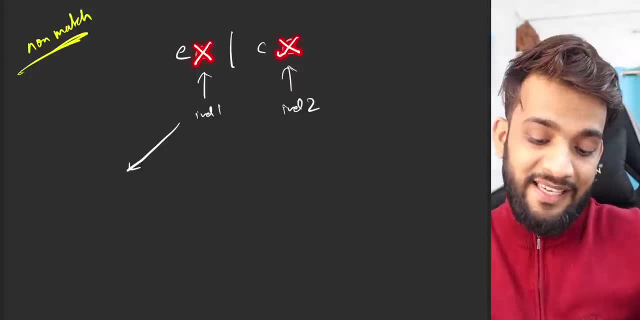 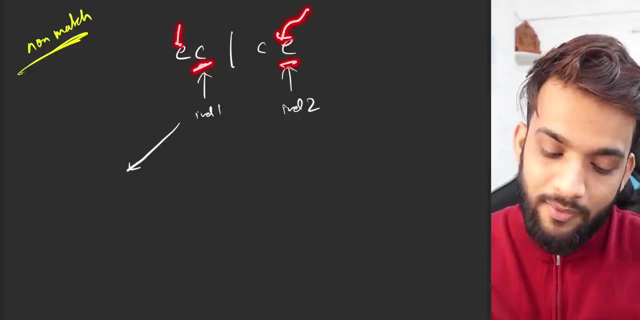 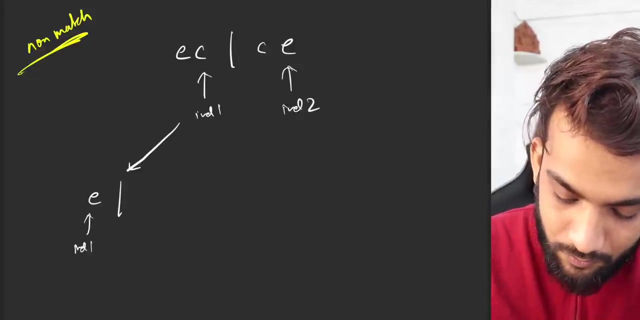 not match with e did not much, but this e might match with the c. i'll be like: okay, this c did not match with e, but this e might match with the c. let's do one thing: let's move the index of one only. let's keep the index 2 as it is. and since they're not matching, the answer added to the. 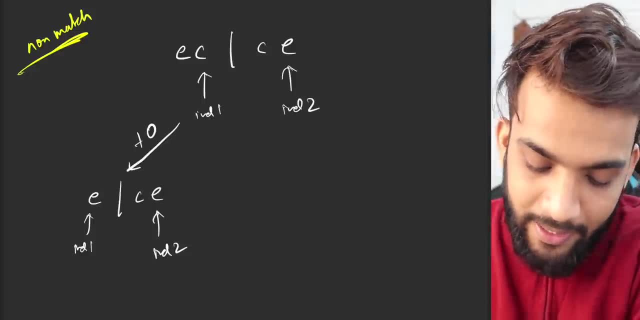 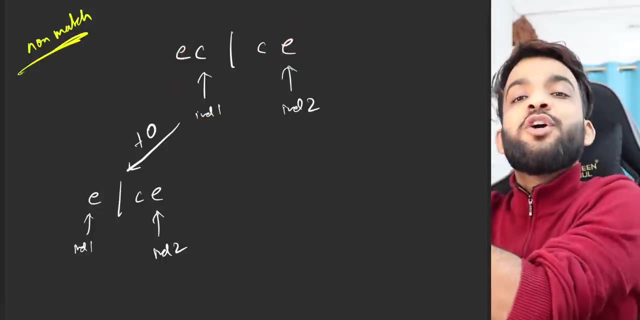 longest will be zero. okay, make sense. i'll be like that, that does make sense because i'll just move this index. i'll keep it because this guy might match in future with these guys. okay, but then you'll miss out on this c. i'm like, okay, let's take the other way as well. 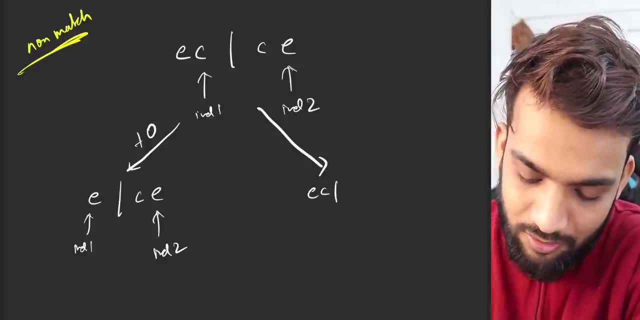 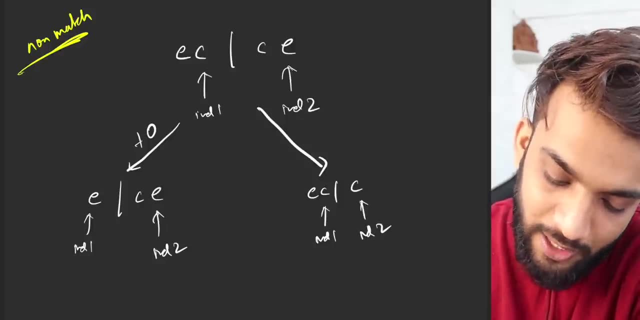 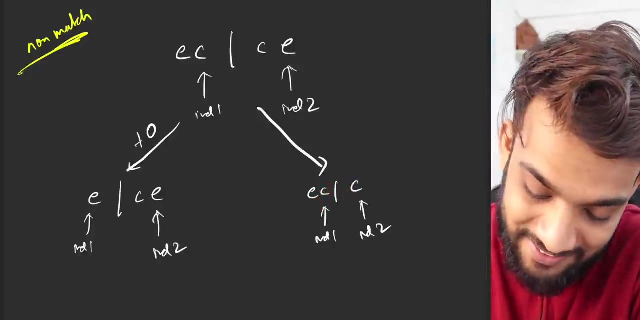 when i say, okay, listen, let's keep ec, that means let's keep index one, let's move c, let's move index two, let's move index two here. okay, makes sense. now the cnc might match. now the cnc might match out. why? because of match on indexes in the next step. 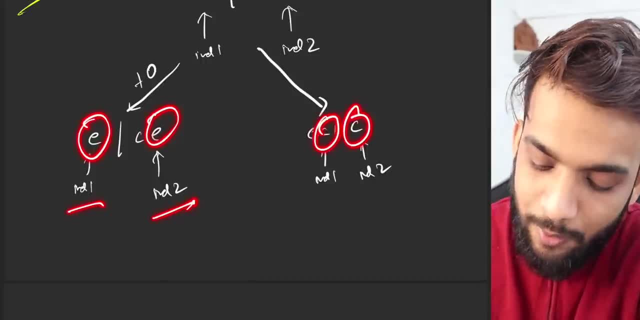 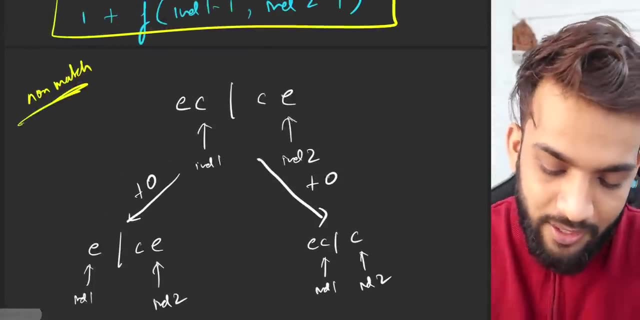 E and D will go and match on indexes, C and C will go and match on indexes, And over here there's a plus 0. That's sure, But did you understand what I tried to do? I said, hey, listen, if they're not matching. 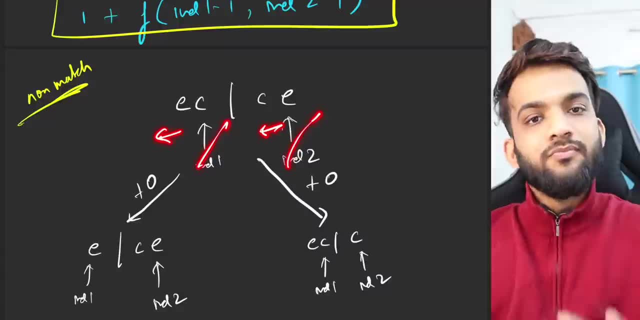 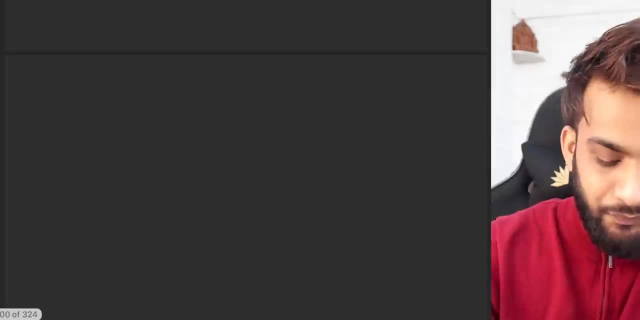 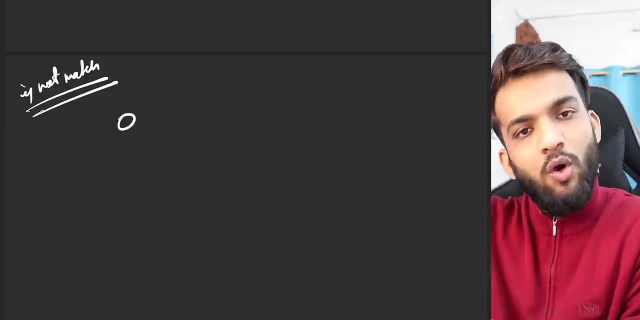 let's either move this or either move this. There's both the possibilities. I'm like: okay, does make sense. So can I say: if not match, then the answer added will be 0 for sure, because there is no length that you are matching. 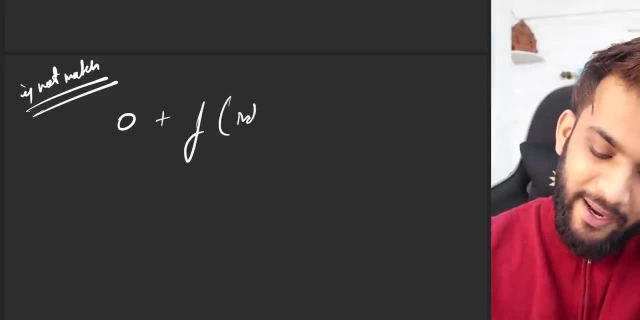 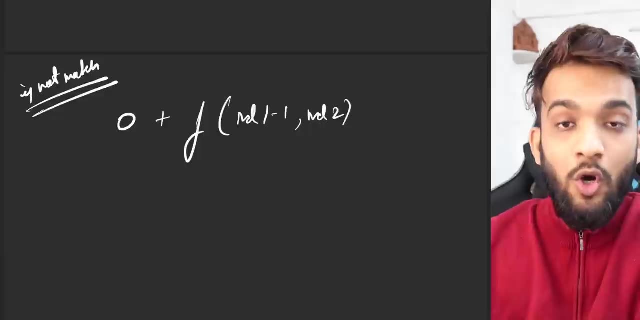 Plus F of index minus 1 is what you will go. Sorry, index 1 minus 1 is what you will go, And it will keep the index 2.. Or you will go: you will keep the index 1 and it will go the index 2 minus 1.. 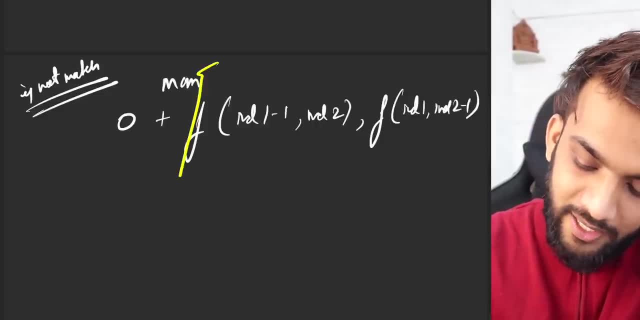 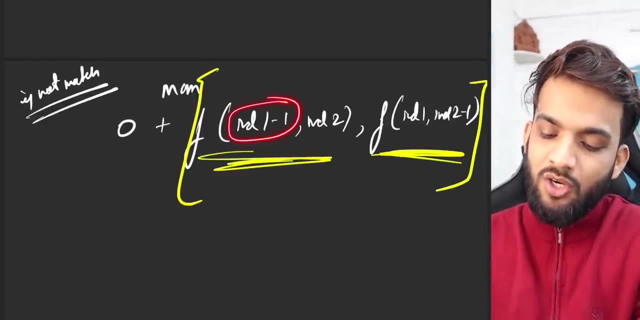 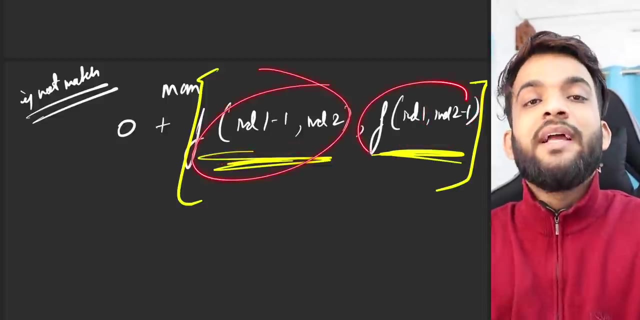 Okay, And it will take the max of both the guys. Yes, it will take the max of either this guy, or either this guy And you can easily just move this, or you can easily move this And the max of this, and this is what you will get- the answer. 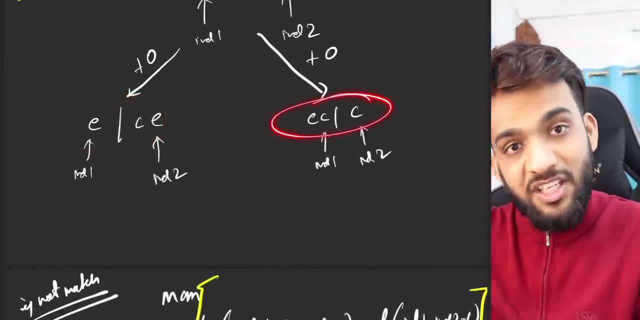 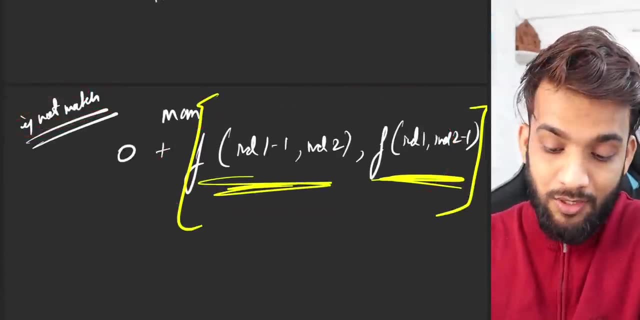 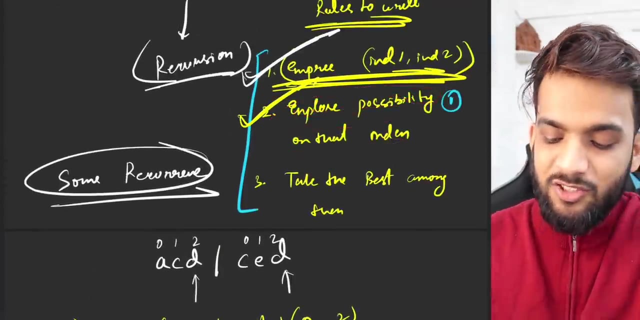 Like: either solve this guy or either solve this guy. Whichever gives you the maximum answer is going to be the max answer. This is what, if not, match will be. So we have also explained: Explode all possibilities on that index. Take the best among them. 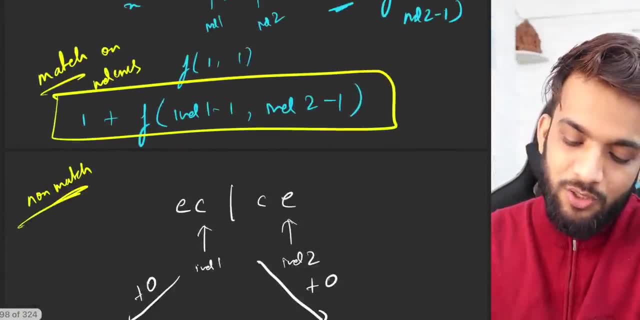 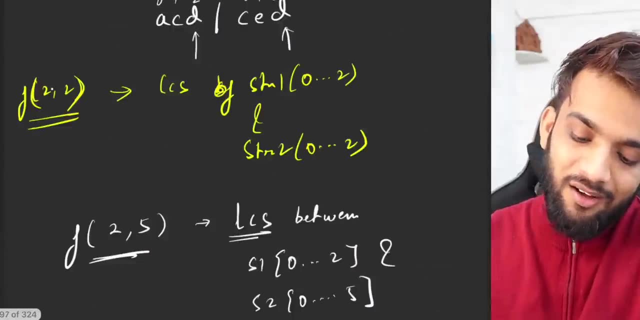 You are taking the best among them. You either take on match. you either take this. If they do not match, you take the best of this or this. So you have also done: take the best among them. So that is how you can easily think in terms of DP on strings. 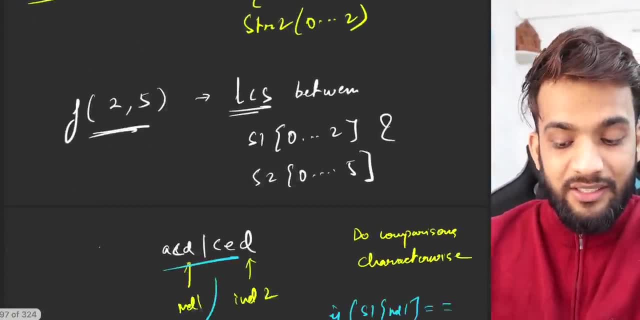 I will be drawing the recursion tree, Do not worry about that, But that is how you can easily think of DP. on strings, What are the base case? We will think about that, But let us try to write as of now the code in short: 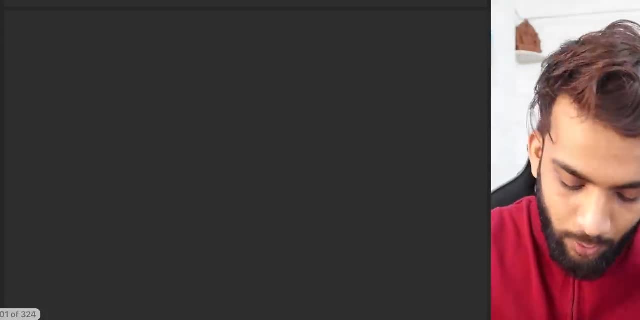 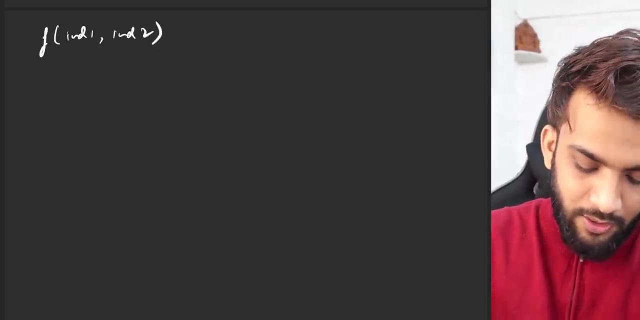 And then I will think about the base case. So I will be like, okay, F of index is F of index 1, and index 2 is there, That is for sure. Let us forget about the base case. What are the cases? 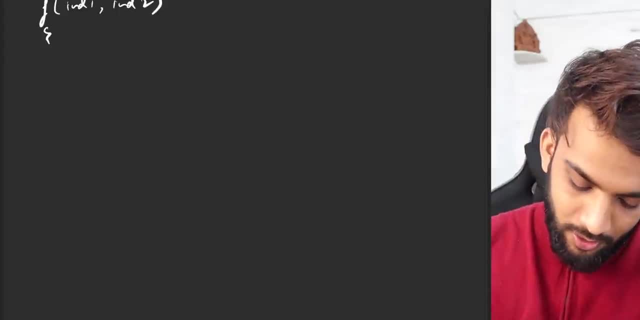 Possibilities: Match or not match. So if they match, Can I say: if they match, then it will be index 1 equal to equal to index 2.. It can be, And what will be the answer? The answer is very simple. 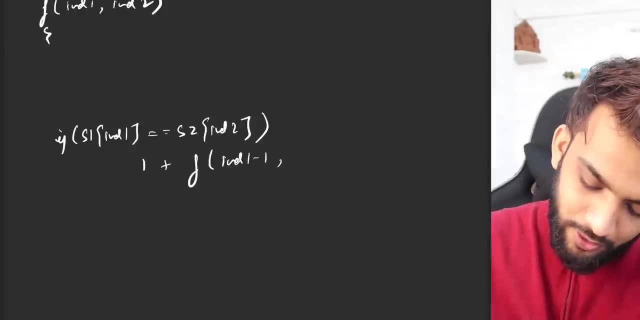 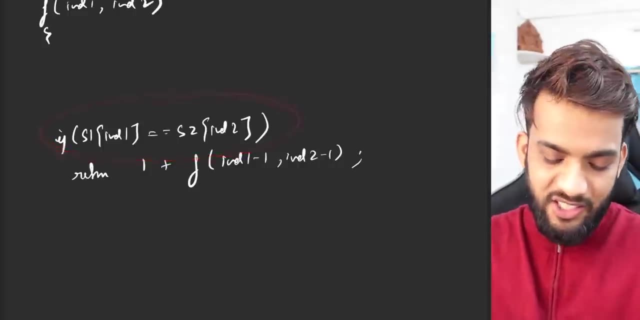 1 of F of index 1 will also move, index 2 will also move and you can easily return them. So if this line does not, if this line executes, the program returns over here and it goes back. The rest lines will never execute. 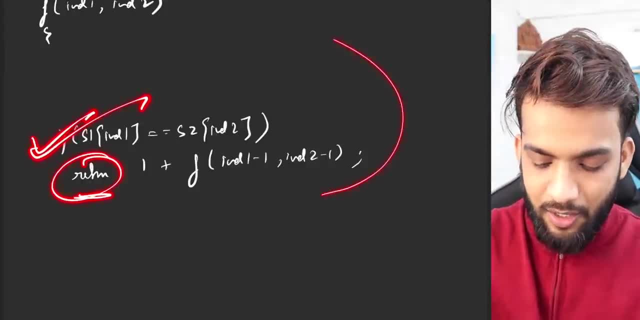 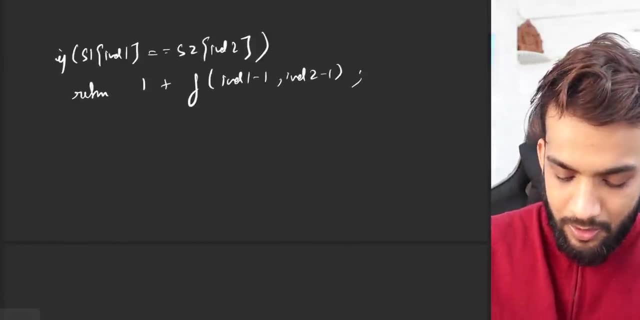 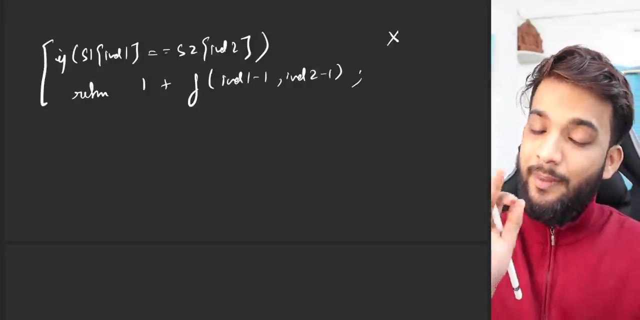 Remember, if this if executes, the program returns over here and these lines will not be executed. So I will write the next lines. What will be the next lines? The next lines will be very simple. I will be saying either: if this is not happening, if this is not happening, thereby no match. 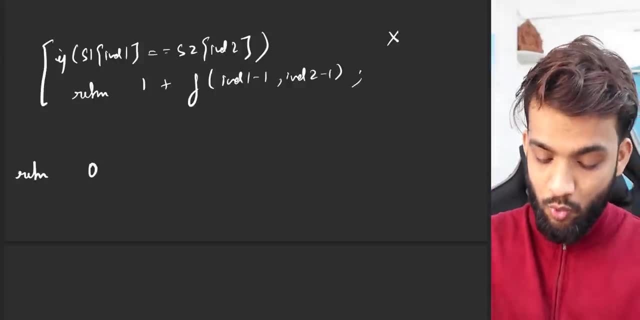 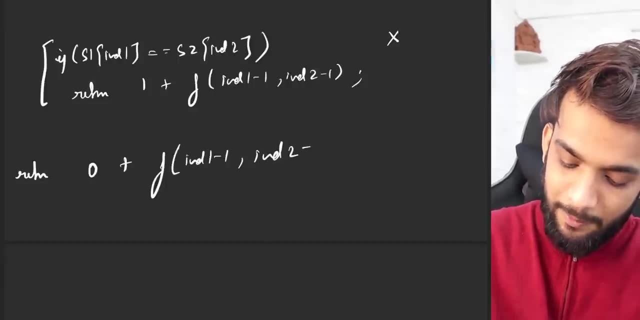 If no match, can I say the answer will be 0 plus, I will move the index 1 by 1 and I will move the index 2 minus 1.. Sorry, index 2. I will keep it like this, or I will be keeping the index 1 and I will move the index 2 by 1, and I will take the max of the best of them. 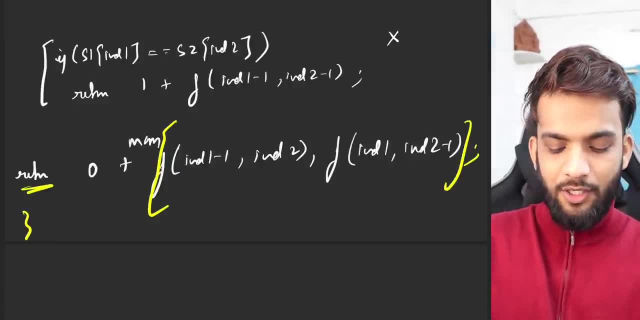 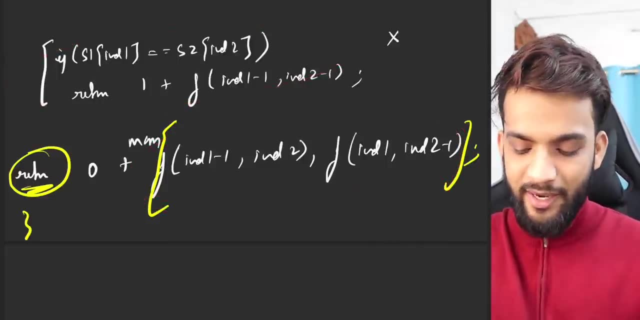 The best of them And that's what I will return. If they are matching, it's fine. If they are not matching, then take the max of these couple of guys and return. So if I just write it in a sophisticated way, in a sophisticated way, it will look something like this: 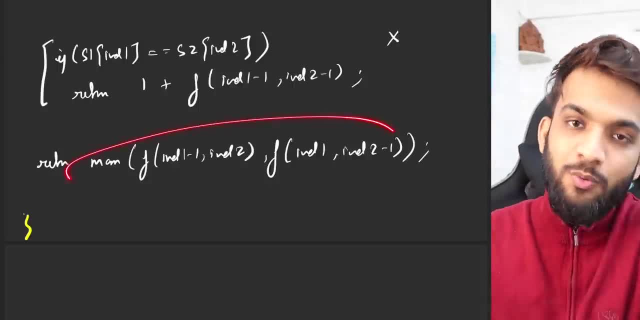 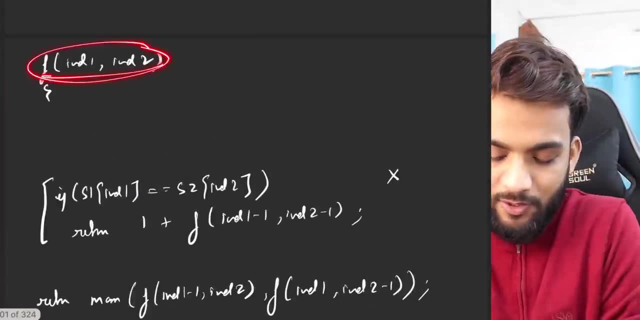 Like 0 plus 0 doesn't have any significance. This one not match. this one match As simple as it can get. So that's what about? that was about the possibilities, But what is the other thing that's remaining? 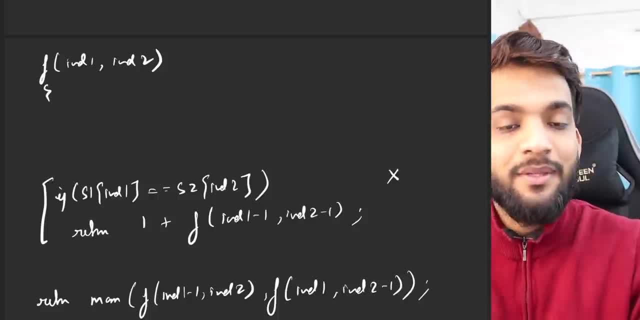 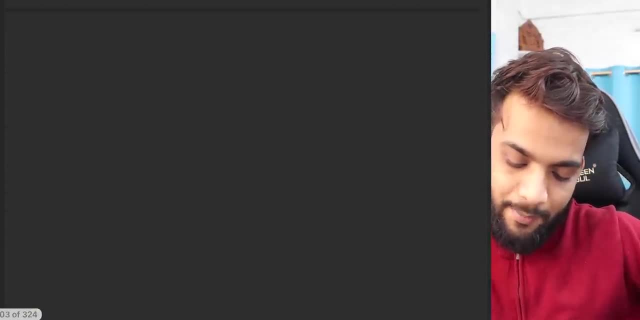 That's base case. yes, That's something which is base case. Let's think about the base case. So can I say when will the base case come? Okay, let's come back and see When will the base case come. 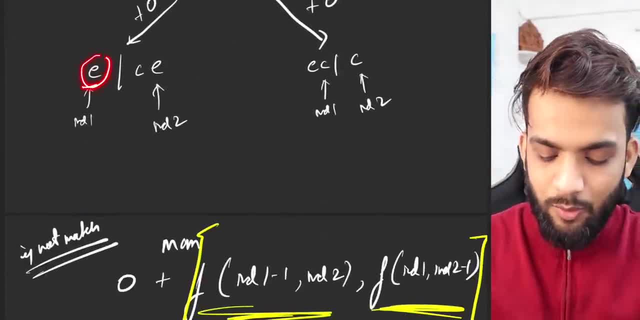 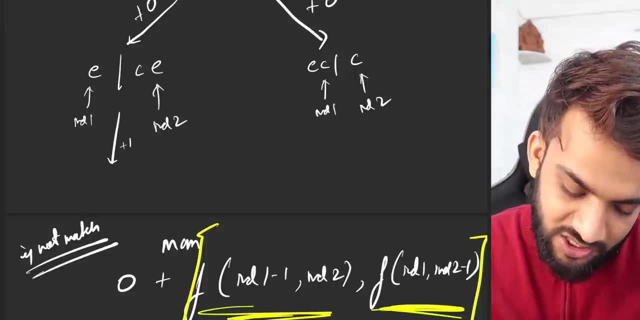 Can I say I am a T? I am a T At this portion. what will happen? You will say: I will do plus 1 because because this E matches with this C And thereby this index will go minus 1.. 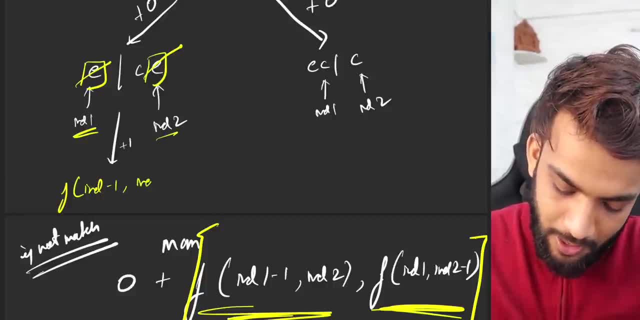 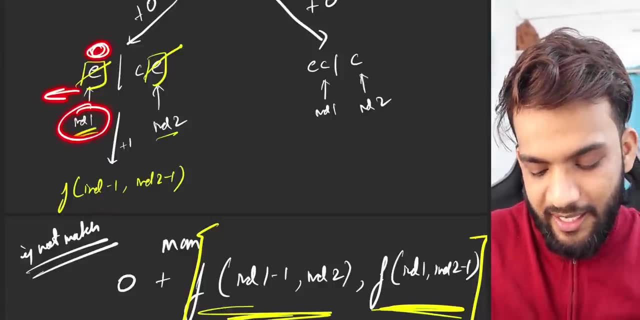 And the other one will also go minus 1.. But if, if this guy goes minus 1, it will go to negative, because this was the 0th index. It will go to negative, And if it goes to negative it's over. 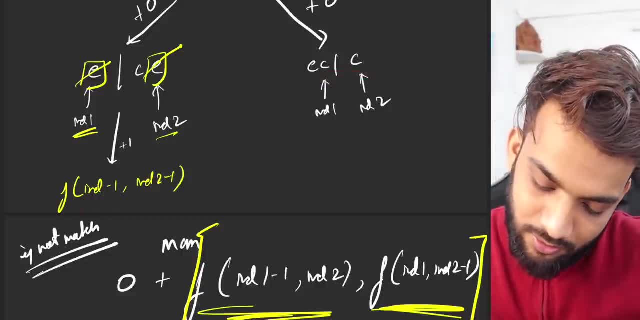 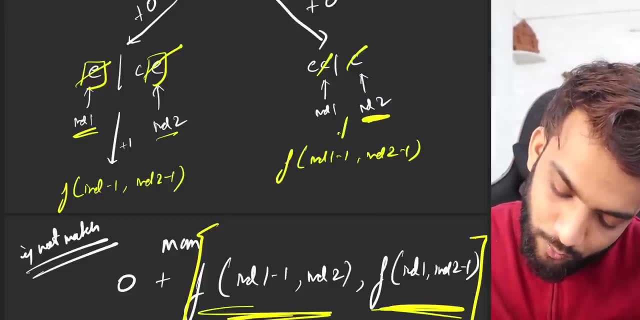 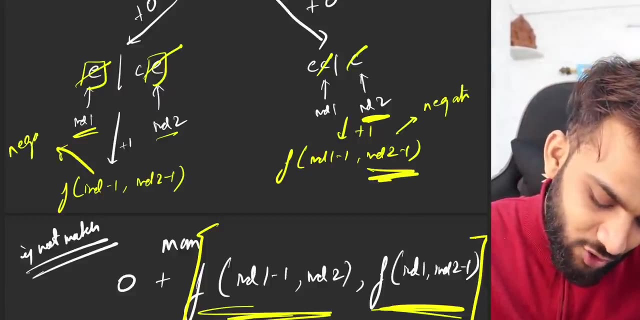 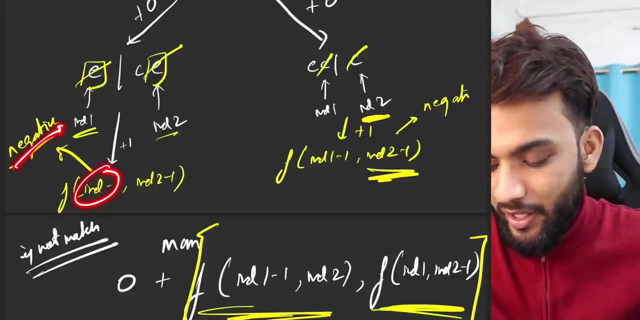 And similarly over here. this will happen. They are matching, So index 2 will go to negative, Index 2 will go to negative. This will become negative Over here. this becomes negative because they have matched. So when you are comparing, when you are comparing, either of index 1 becomes negative or either of index 2 becomes negative. 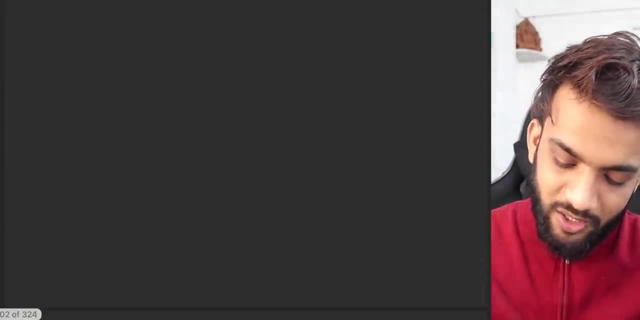 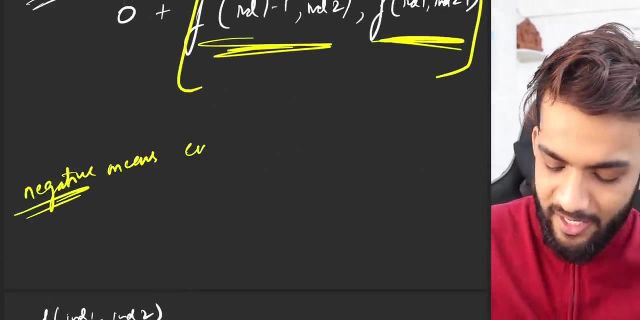 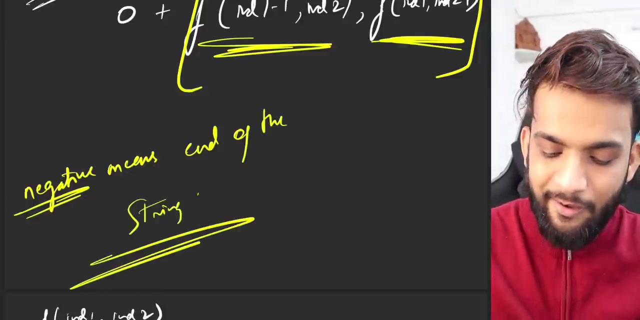 What does negative signify? What does negative signify? Let's try. Negative means end of the string. Negative means end of the string. Very simple guys, If, if, if. F of 2 means string 0 to 2.. 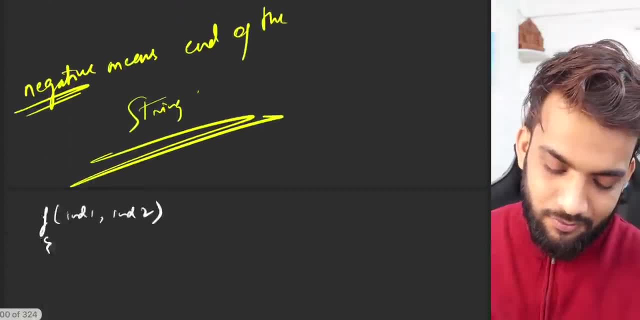 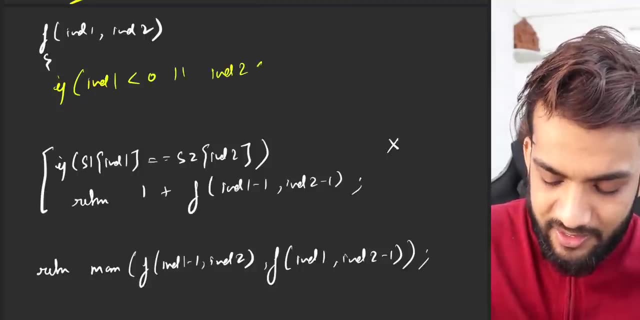 Negative will mean end of the string. So can I say? can I say: if at any moment index 1 is lesser than 0, or or index 2 is lesser than 0, I can say it's the end of string. 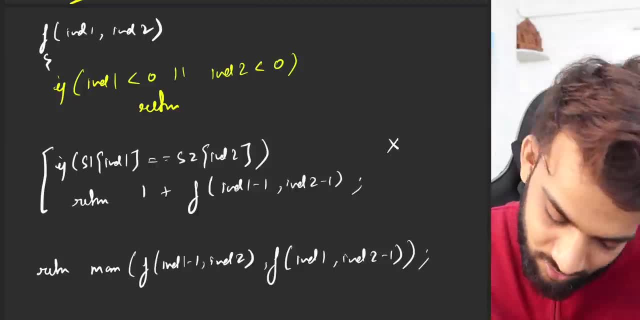 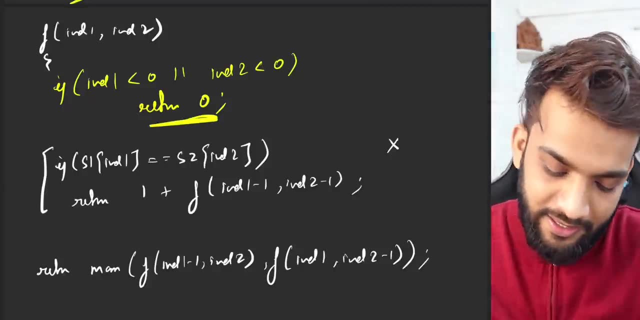 If it's the end of the string, what is the longest length? 0.. What's the longest length? 0, guys. So I can say this is 0. And I can easily return: If this goes negative or this goes negative, you don't have anything to compare. 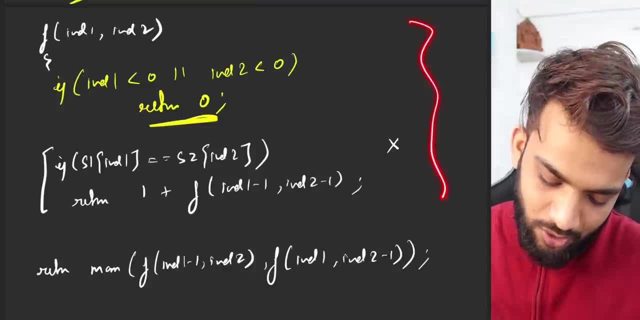 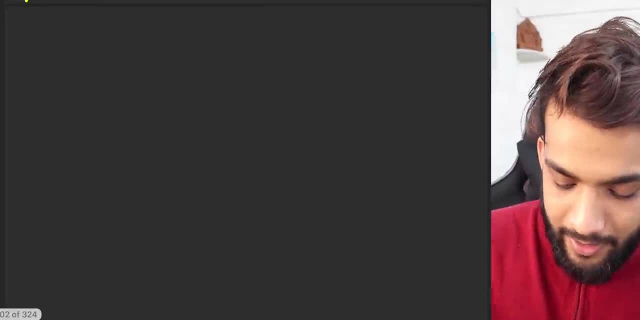 So the returning length will be 0.. This is how the recursive code will look like. Now, in order to get more clarity, what I'll do is I'll take this example and try to do a recursion tree so that it gets clear on you, like on a crystal clear method. 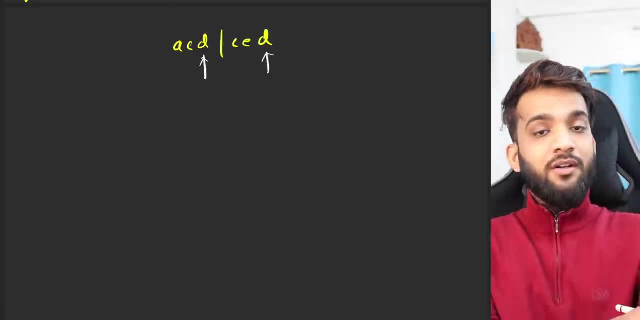 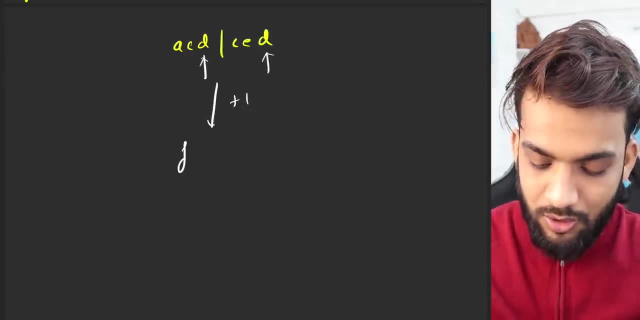 C, E, D. Okay, Where are we? We were here, We were here. Okay, What did the first step F of one one plus Perfect, And I'll call the function. So over here it'll be something like 0, 1, 2, 0, 1, 2.. 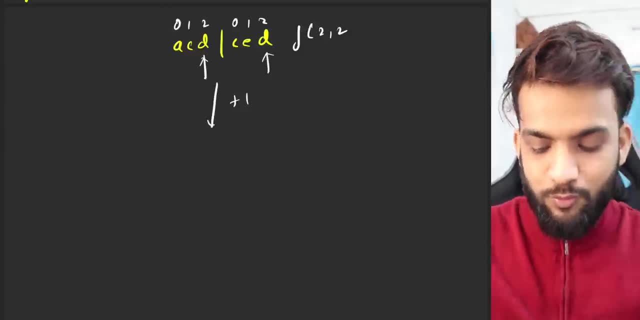 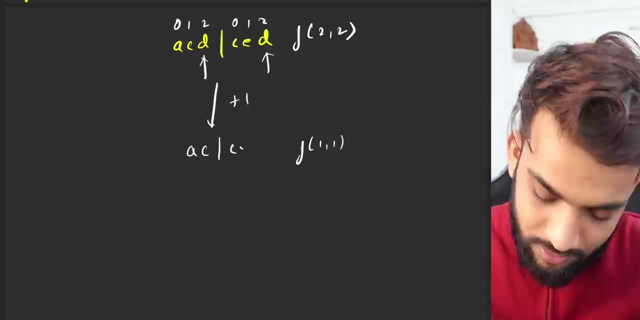 The function call will be for F of two, two Right. What will be the next function call, Plus one on F of one, one which will be A, C and C E? F of one one means A, C and. 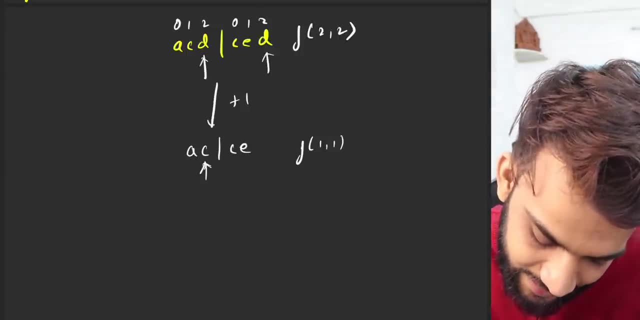 C, E. So AC is here and E is here. Are they matching? No, So there will be two split calls. There will be two split calls. Let's do the two split calls. So if I do the two split calls, what are we going to get? 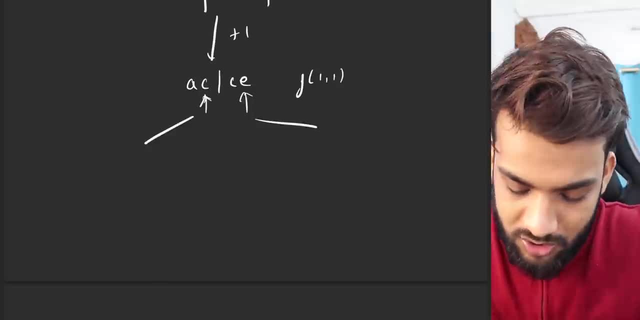 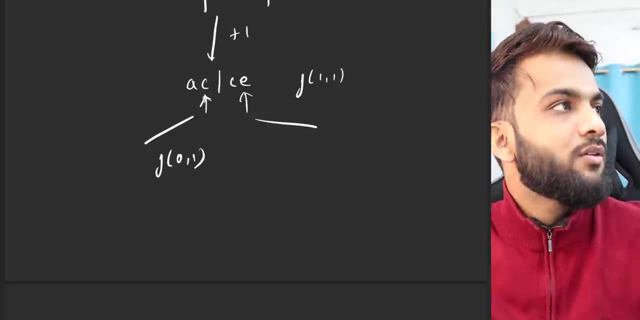 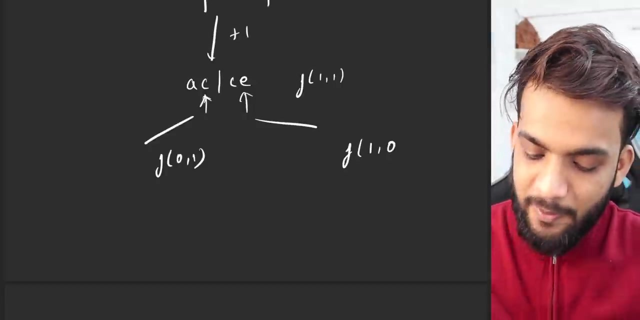 I get a two, I get a two right. Okay calls: it will be plus 0, and f of 0- 1 will be one split call and f of 1- 0 will be another split call. basically, you reduce 1 or reduce this one. that's what. 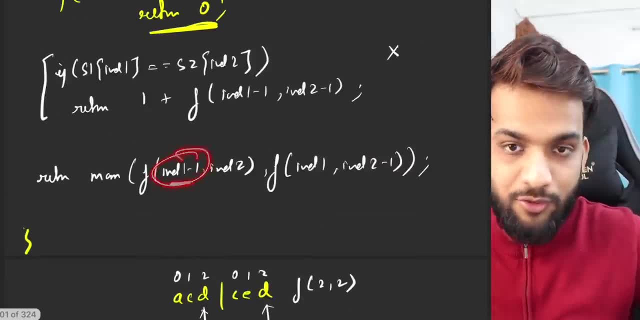 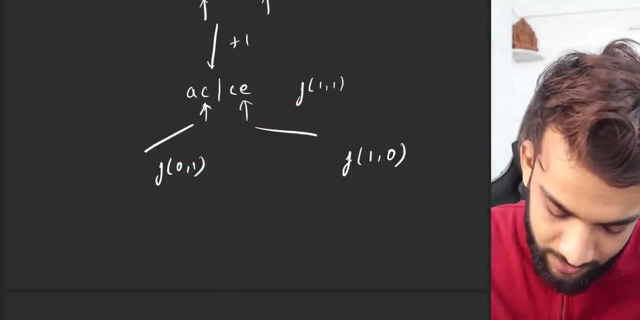 you did right, that's what you did. you either reduce this or either reduce this, so a split of 1 of 0 or a split of 1 of 0 will happen. okay, so what does this signify? 0 of 1, a CE, and this signifies AC and C. perfect, we are standing over. 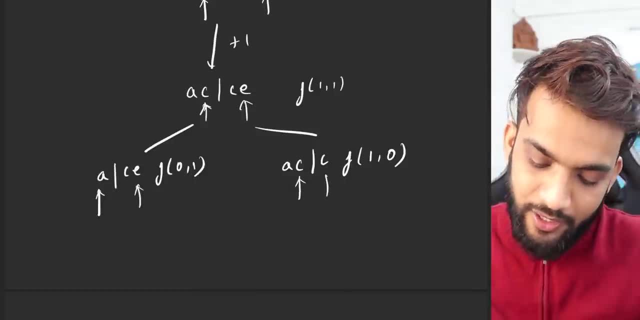 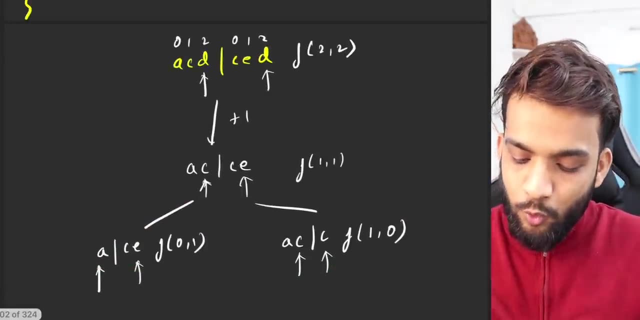 here, we are standing over here. we are standing over here and we are standing over here. okay, so this recursion will be solved at first and then this recursion will be solved at first. you are understanding right. f of 2, 2 will call f of 1, 1. f of 1, 1 will call this and call this and take the max of this and the. 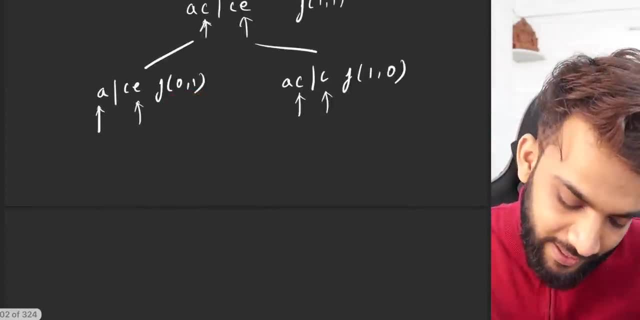 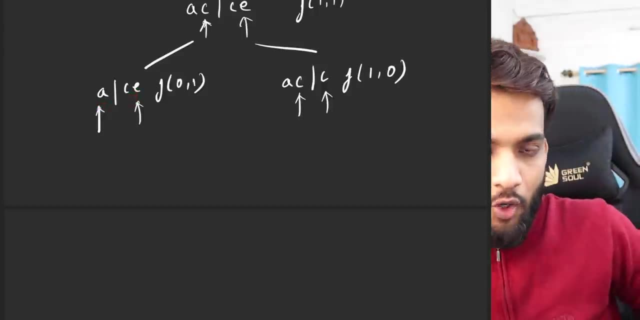 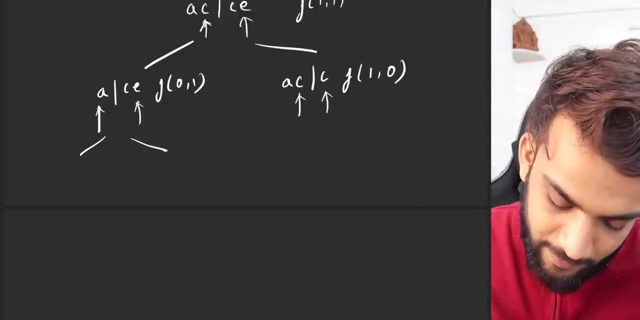 max of this. so f of 0, 1. what will happen? a e- e are not matching, then they are nowhere matching. a and e are nowhere matching. so what will happen? again, two split calls will happen if they're not matching, two split calls. and what will be for the split call? it will go to minus 1 comma 1. 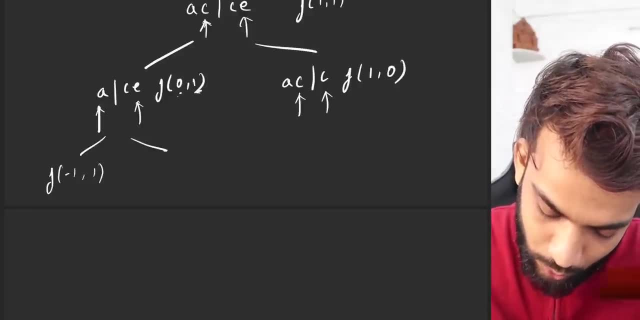 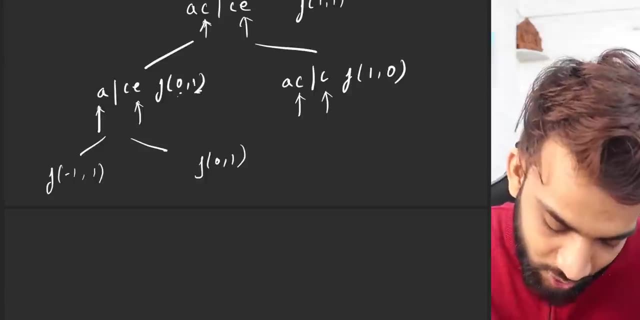 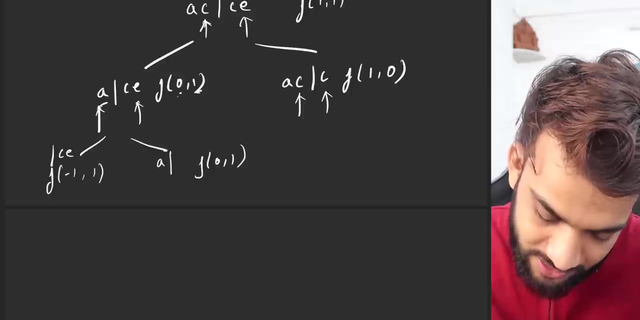 what will happen to the split call. I'll go to f of 0, 0, f of 0: 0. understand: 0 is a split, 1 is so basically you reduce, so over here it gets reduced to nothing by CE and over here it gets reduced to a by C. why? because you're moving this guy. so 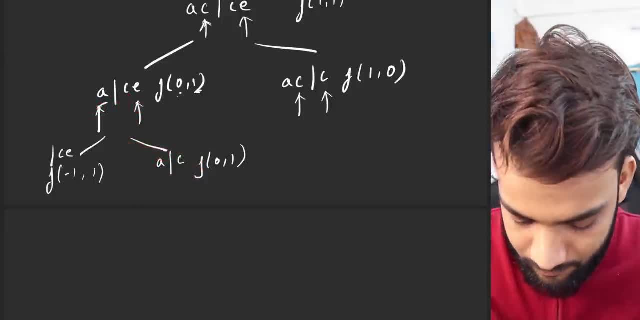 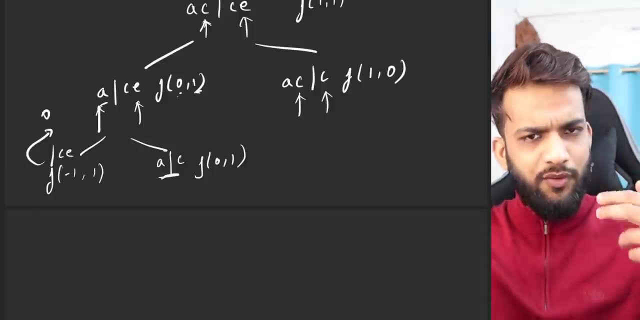 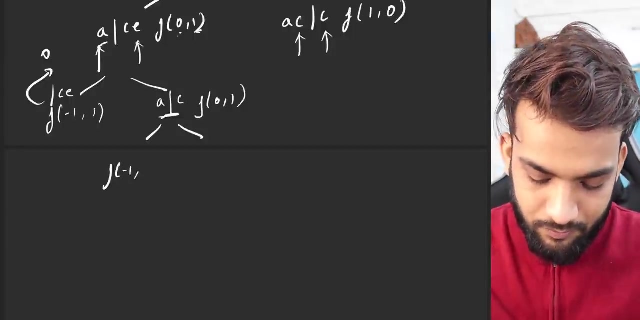 a by C is what it reduces to. okay again, what will this return? negative, this guy returns 0 a of C. if you go on solving this, what will happen again? two split calls: f of minus 1 comma 1 and f of 0 comma 0, or rather this will be a. 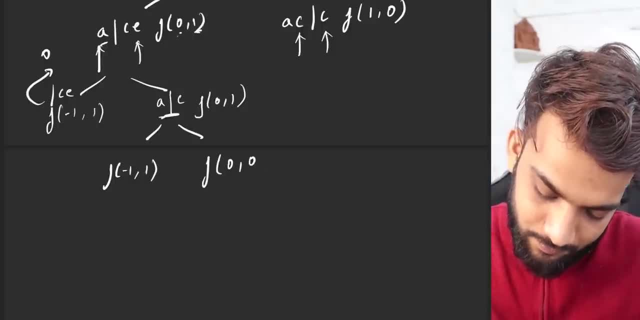 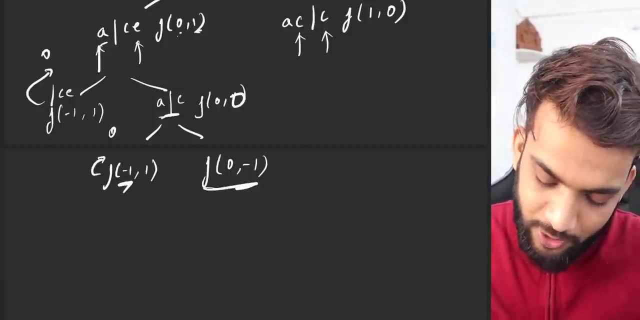 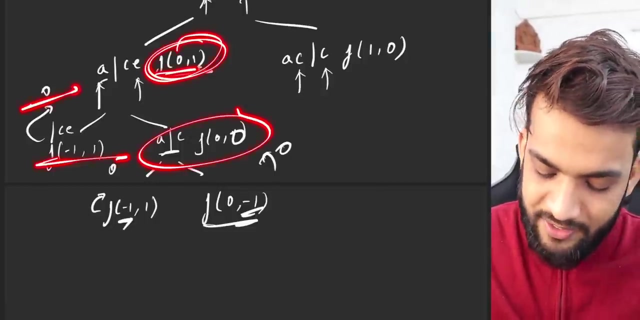 a set of number of numbers where c is equal to 1, or even if it is equal to 1 right now: f of 1, 0, kanske 2, c is equal to 1, f of 1 is equal to 1 and f of 1 is equal. 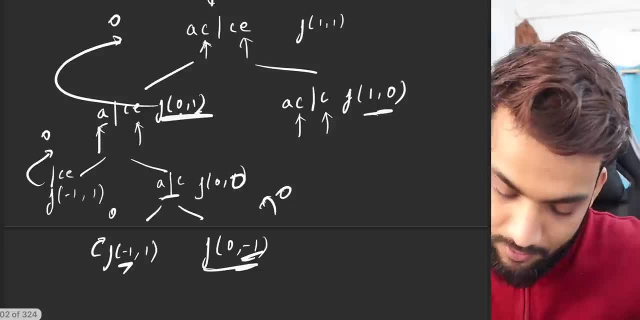 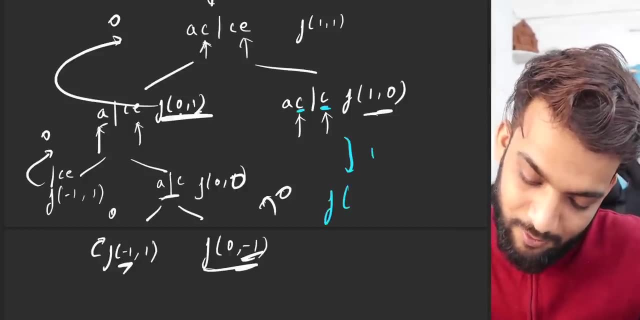 to 2 and again, if it's 0, then this will be x and if it's 0, then g is equal to 1. same situation if it is e, like that same situation has happened over here for this one f of both will reduce zero and minus one, so both will reduce zero, will reduce to minus one. 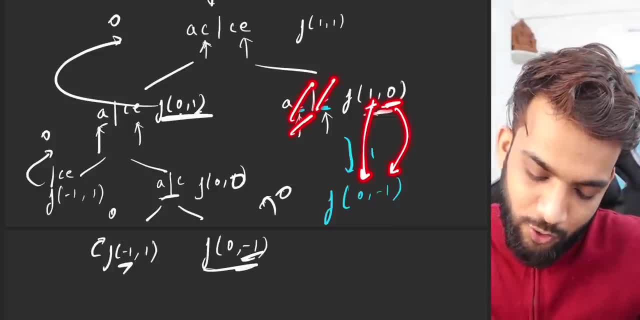 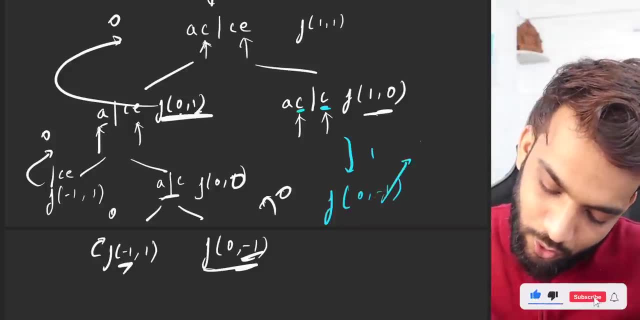 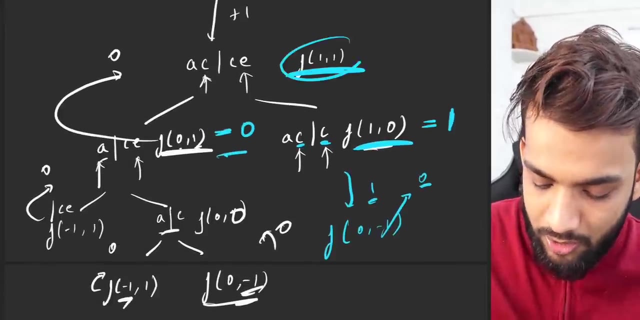 one will reduce to zero because c is done, c is done, so you move this to here and this is over. so one plus this. what is this negative? so this guy will return zero. so one plus zero. this guy's value is one. this guy's value is zero. so f of one. one called both the guys. 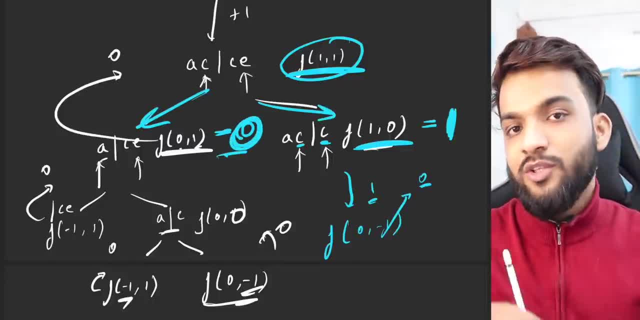 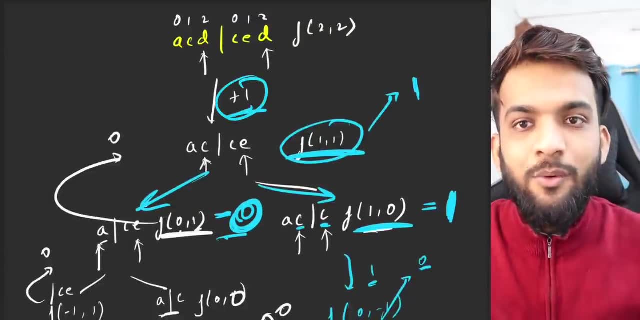 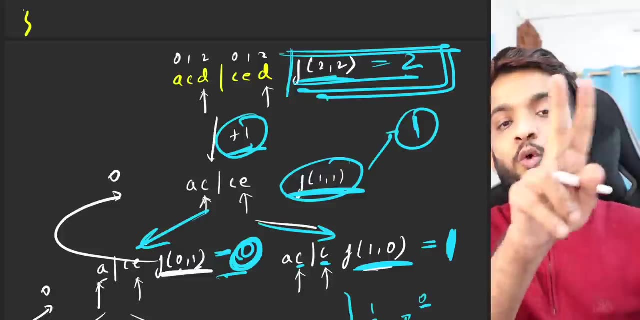 one guy gave him zero, the other guy gave him one. which one will he take? he will take one, the max of both the guys over here. we had a plus one, so plus one and plus one. f of two: two gives you two, which is the answer. f of two, two gives you two, which is the answer. and eventually cd is the string which. 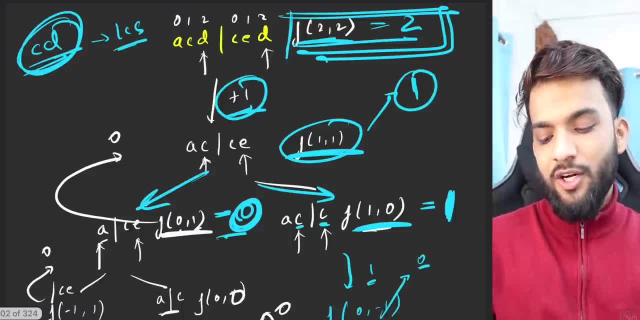 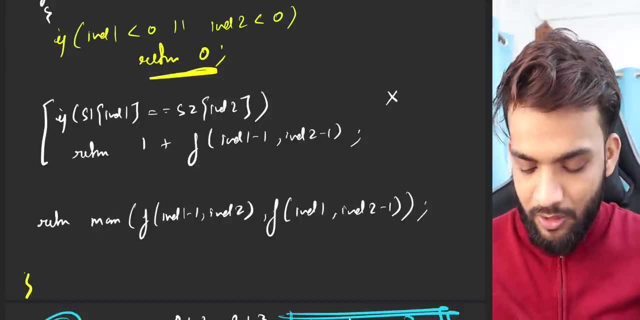 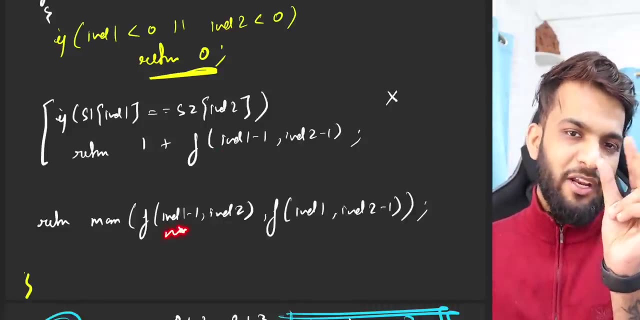 is the longest common subsequence. so you got the answer. so you saw the recursion tree working perfectly and it did give you the answer very straightforward in all the comparison of string problems. if they're matching, you just take both of them back, and if they're not matching, you take either one string. you shrink one string or you shrink the. 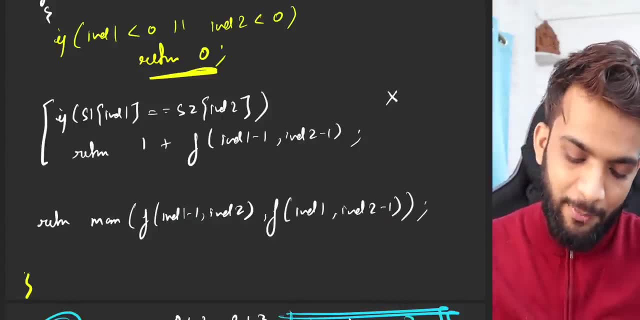 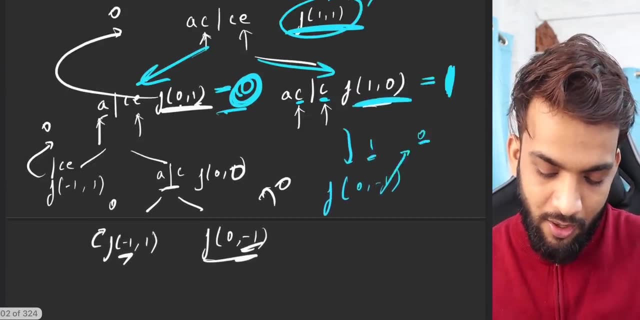 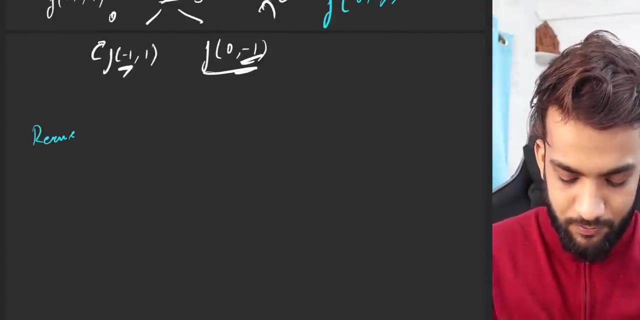 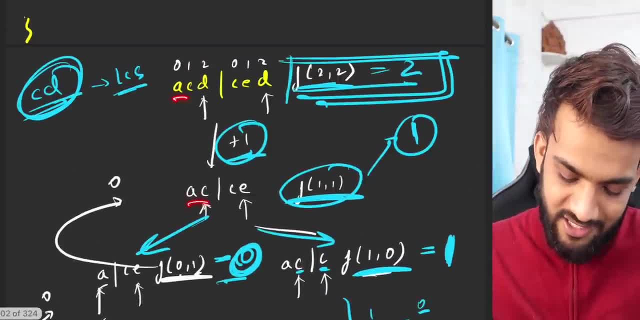 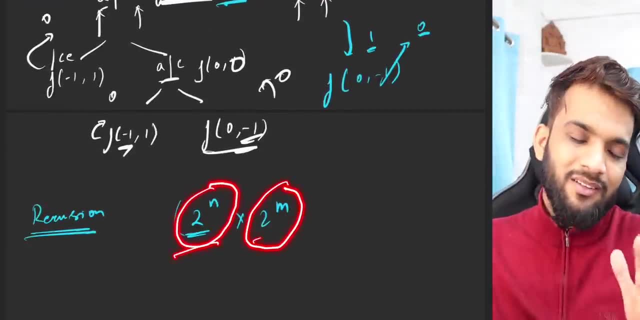 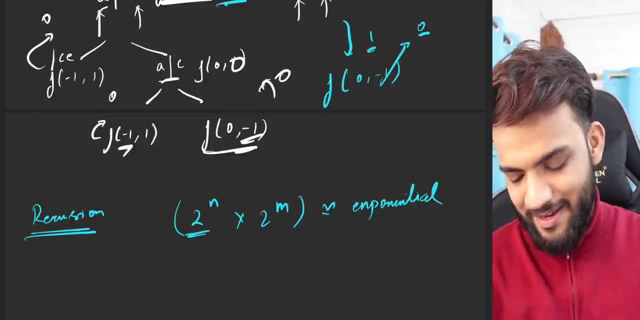 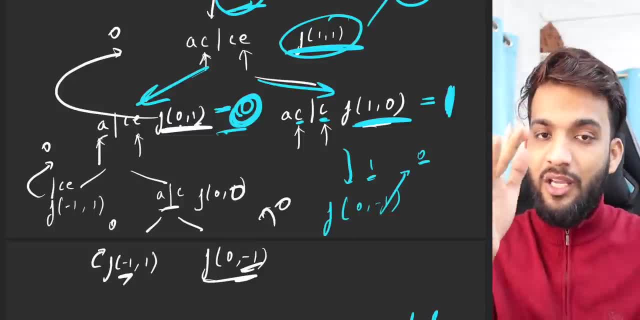 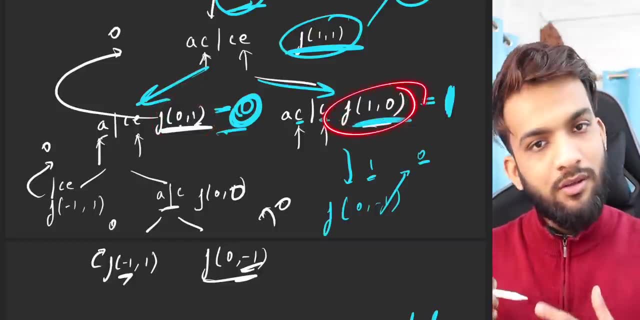 and we know we are doing recursion and we know we are doing recursion and we know we. that's okay, but you will see, if you take a bigger example, you will see states being repeated. you can take a bigger set of string and you'll see that the states are repeated. so what does f of? 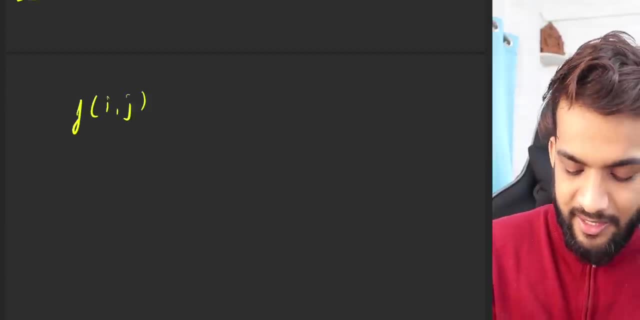 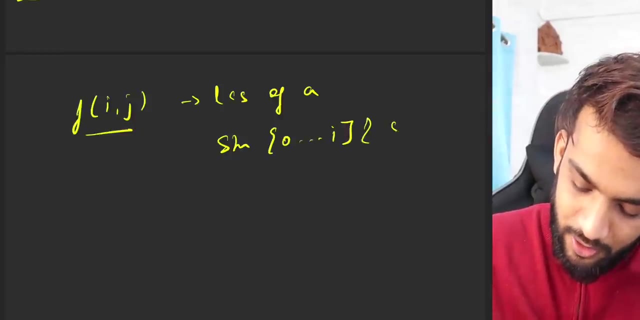 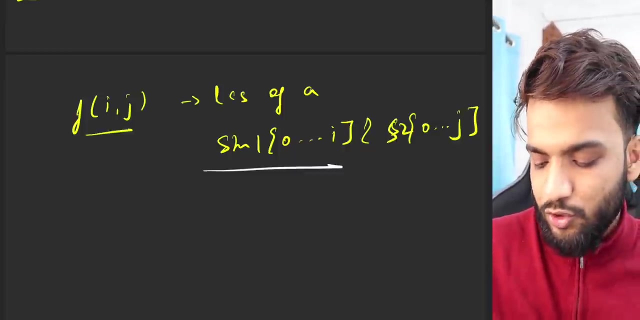 f of i. j state means it says lcs of a string from 0 to i and a string 0 to j. that's what it represents, right: lcs of a string 1, 0 to i and 0 to j. in this they want the length. so if someone 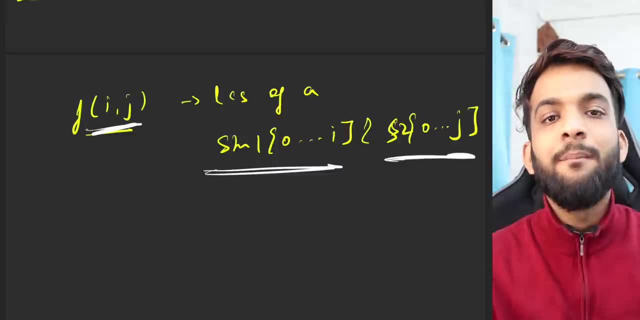 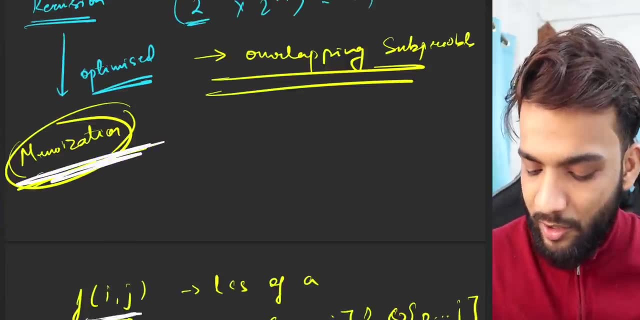 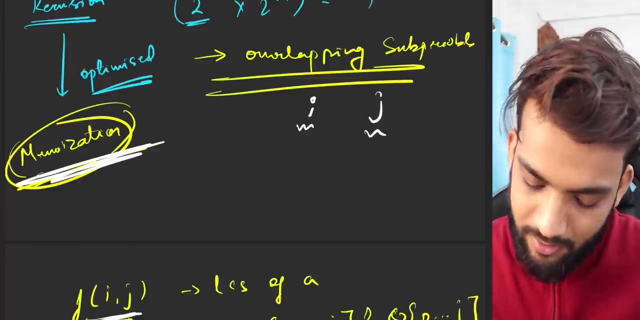 again comes up and asks you the same question: why do you want to pre-compute, why do you want to recompute? thereby we can easily apply memory action. what is the technique to apply memory? look out at the changing parameters. one is i, the other is j. what is about i? it's n. what's about j? 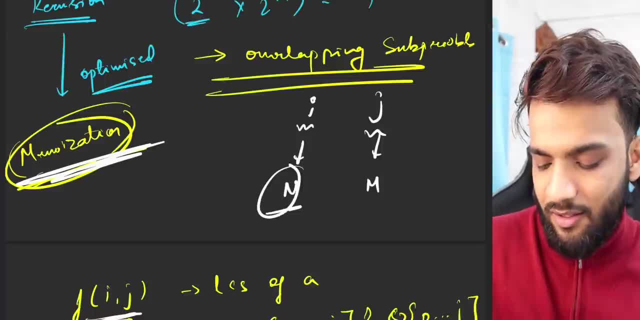 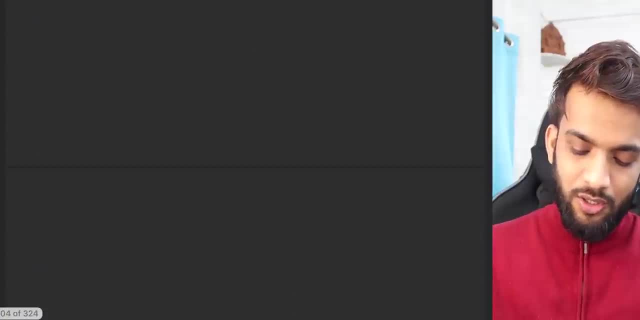 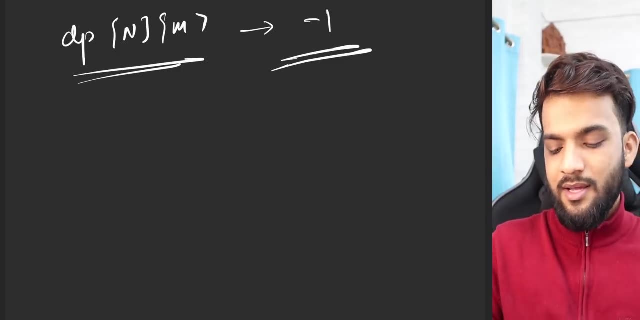 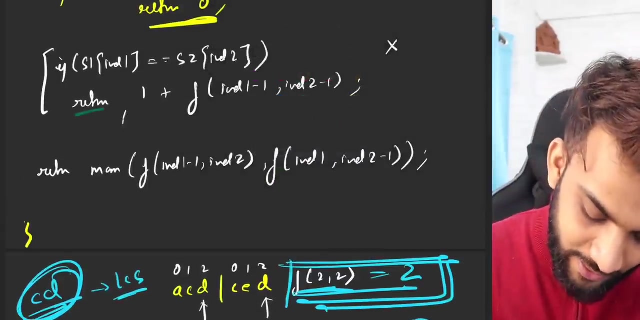 it's but but m. thereby you can say n cross m is what i will be requiring, dp. so you can easily just declare a dp of n cross m, initialize everything to as minus 1 and you can just go back and add these lines over here. this is a return statement, right? so over here you can say: okay, fine, i'll. 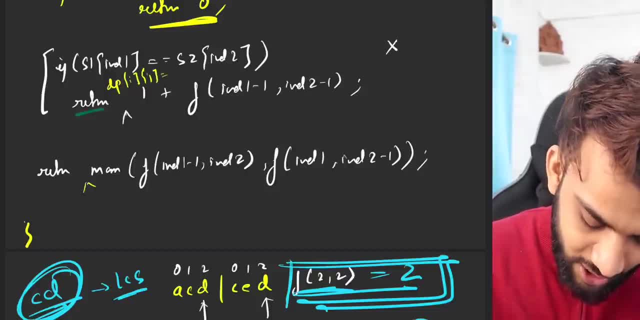 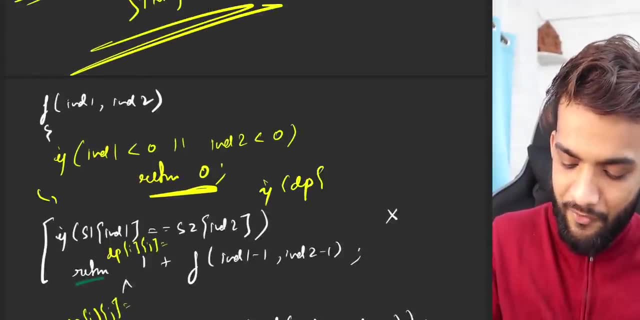 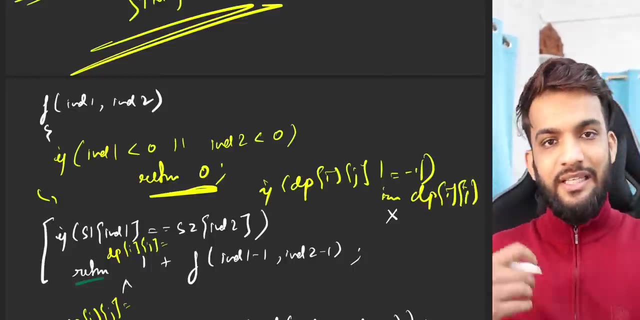 write dp of ij equal to this is a return statement. you'll say, okay, fine, i'll write over here and while, whenever it enters, a very simple line of dp of ij is not equal to minus 1, and you return dp of ij. that's how you easily do it. that's what the function resembles. so it's time to check out. 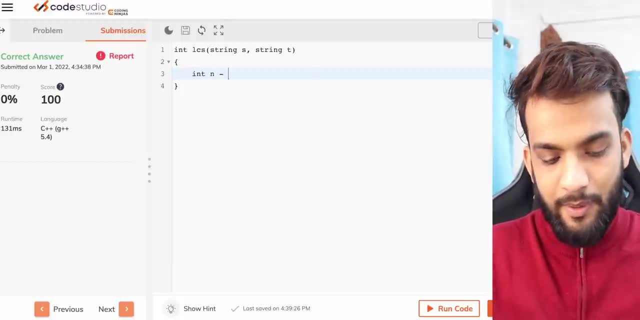 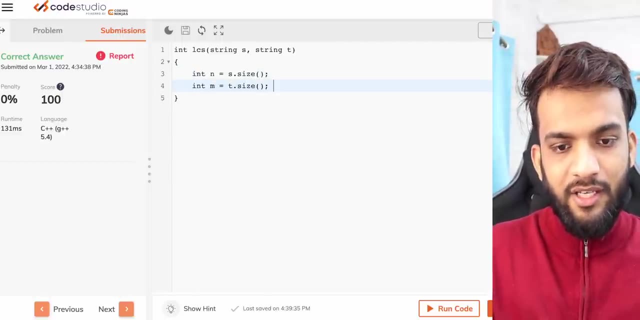 the code uh. so we're given the string s and the string dot t. so really you can just give s dot size, right, and you can just give m equal to t dot size, perfect. and right here you can say: return f of you can n minus 1, that is what you take, s and d, perfect. let's quickly write the function that. 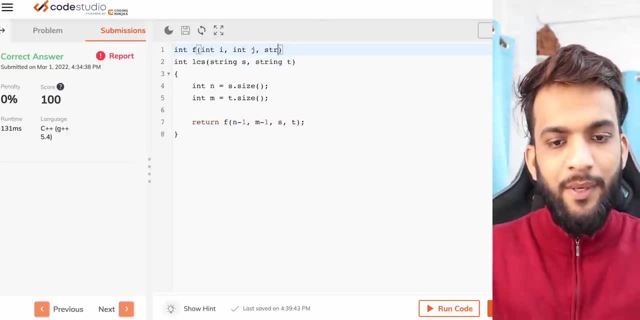 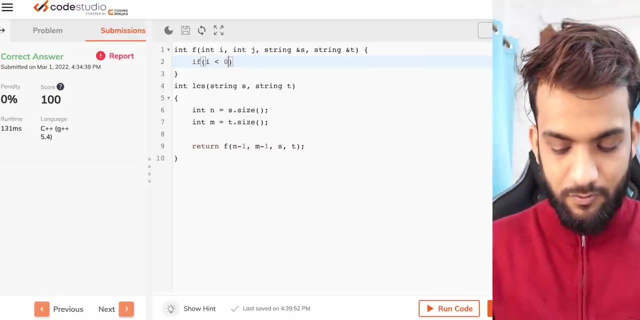 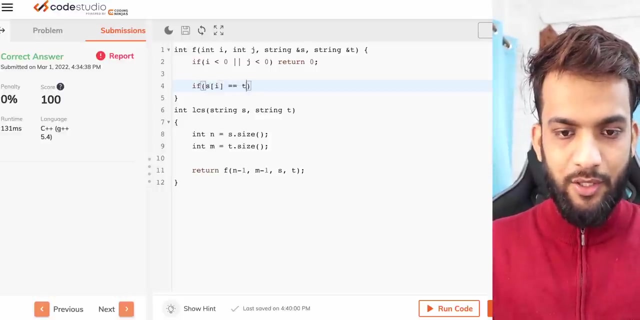 we generally write int f, int i, int j. make sure you pass the string by reference, because every time, if you create a new string, it might give you tle. this is what you wrote. this is what you wrote. return zero if they're matching. which is s of i equal to t of j. 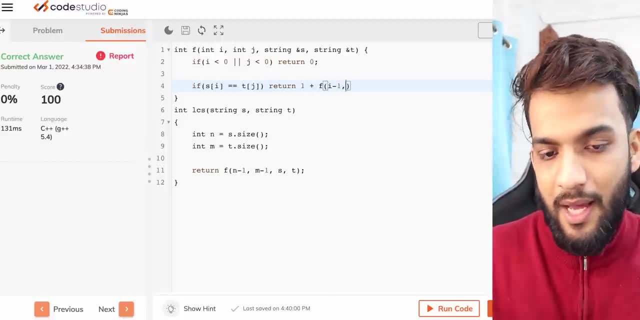 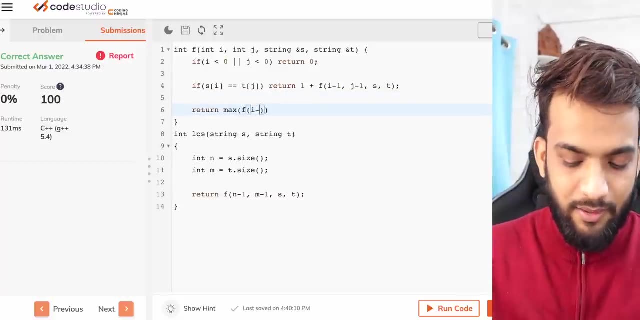 then you're going to return 1 plus f of i minus 1, j minus 1 and an s and a t and they're not matching. you return the max of either both of them click and i minus 1, j, s and t, or you just go one which. 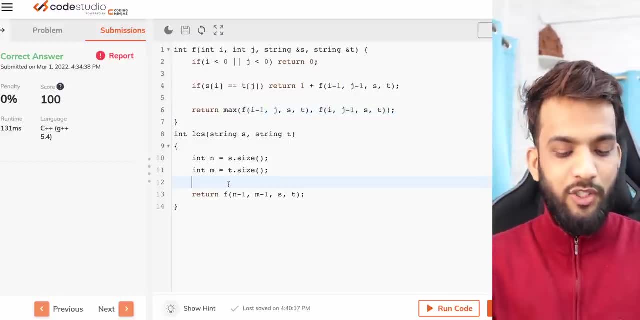 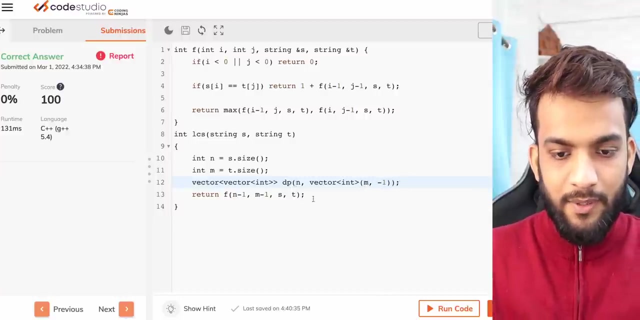 is s, comma t. this is how the brute force will look and obviously you need to optimize this by applying memoryization. so just apply memoryization over here, which is dp of n cross vector of int and m cross minus one. please make sure you pass the dp over here and once you pass the dp, right. 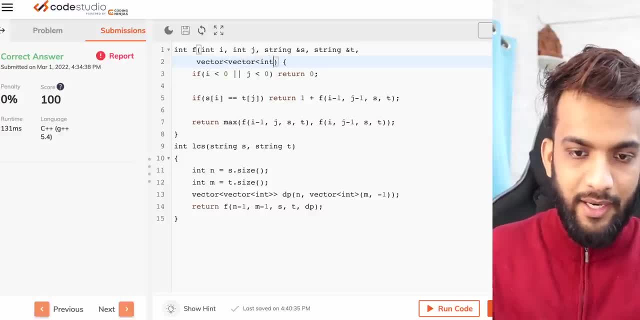 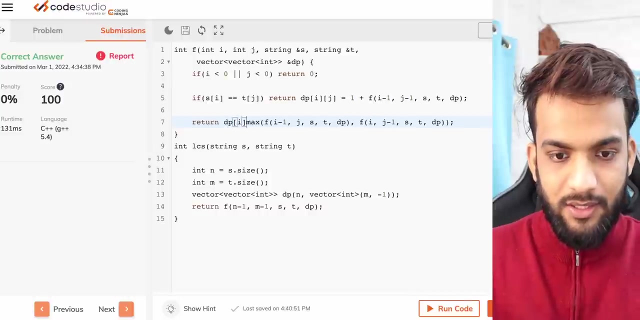 over here. you can say vector of vector, int and dp, and you just pass on the dp over here. you can just pass on the dp over here, you can also pass on the dp over here. perfect, and what i can say is: okay, fine, the next thing that i'll do is memorize. let's quickly memorize this as a last thing. you will see. 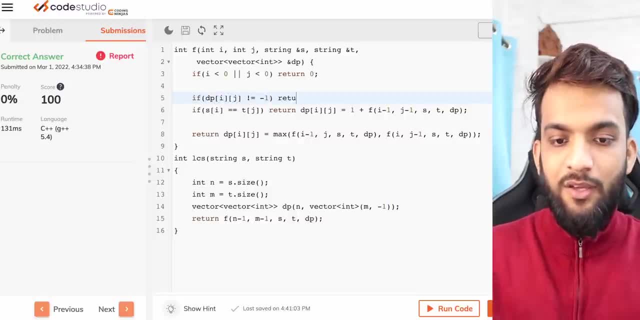 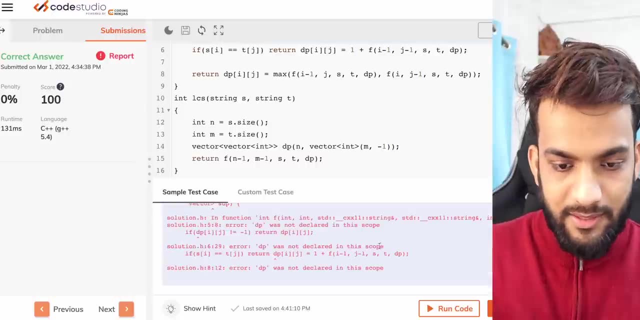 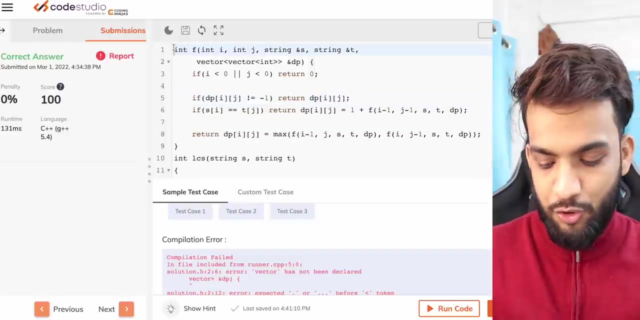 please check if the state has v s and that's what the code will look like. hopefully it should run. okay, it has some issue? okay, uh, db was not declared in the scope. okay, looks like vector has not been declared. so what it says is: you have to actually use hash include bits s, t, d, c plus plus dot h, because vector has. 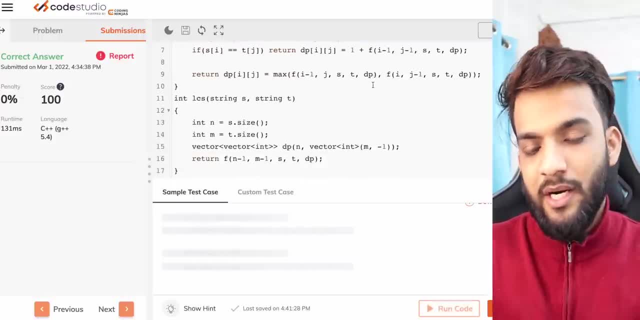 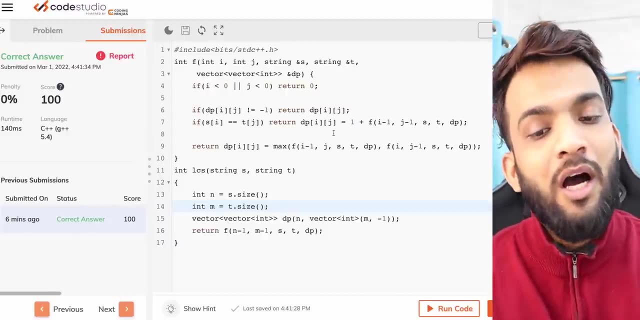 not been defined, so it can easily define this and after this i think it should be running fine. fine, it runs. now we're getting an hundreds code. now, that's the memoization technique will be now. the next step will be tabulation, because we have to optimize. 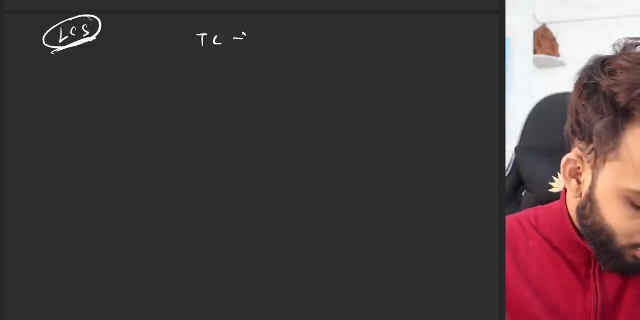 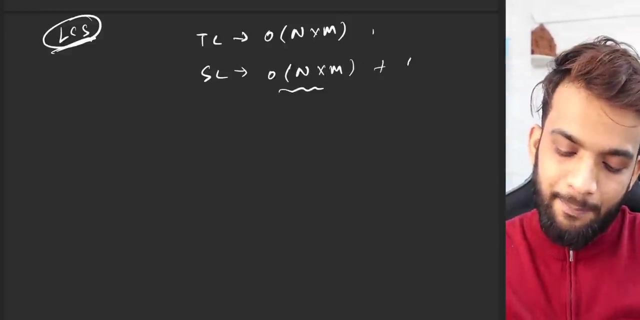 the auxiliary stack space and the time complexity in order to solve this by memoization was we go of n cross m, which we took in order to solve this using memoization, and the space complexity we took was n cross m for the states storage in dp and then we go of n plus m in an auxiliary stack space. 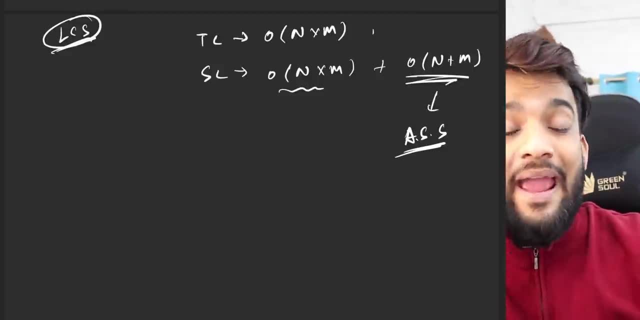 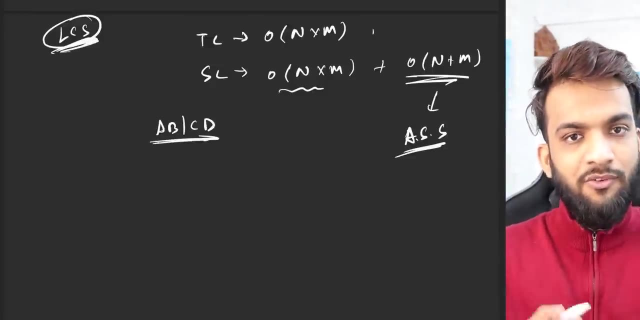 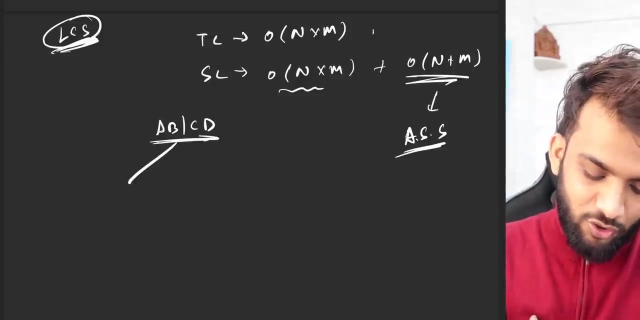 right now. you might ask why n plus m? i'll give you an example: a, b and c, d. i'll ask you to draw the recursion tree for lcs. if remember in match- in match it was one plus and in unmatch you moved in two directions. so this is unmatched. so you move in two directions, which is a by c, d and the other. 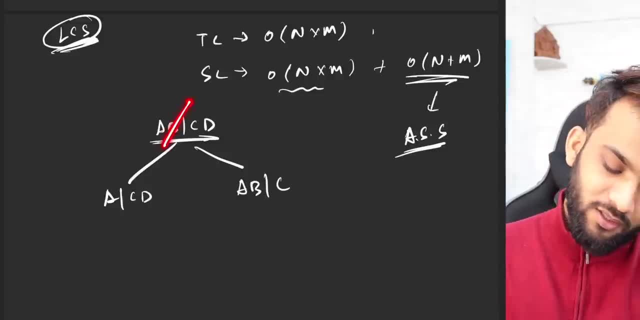 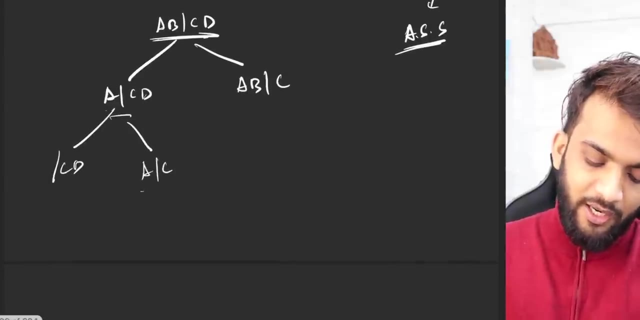 one is a, b by c, very obvious, because you either eliminate this or you either eliminate this again over here. you again move in two directions, because they do not match. so you either eliminate a, which makes it cd, or you either eliminate d, which makes it a by c. over here, again in two directions. you either eliminate a or you either 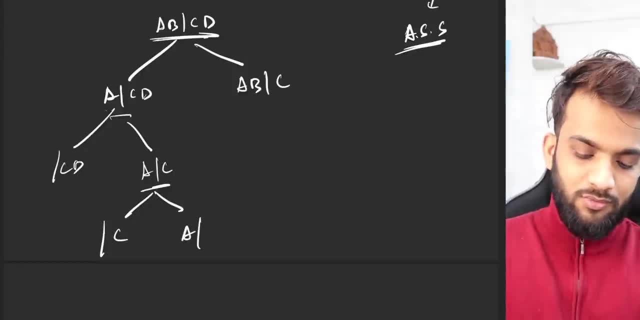 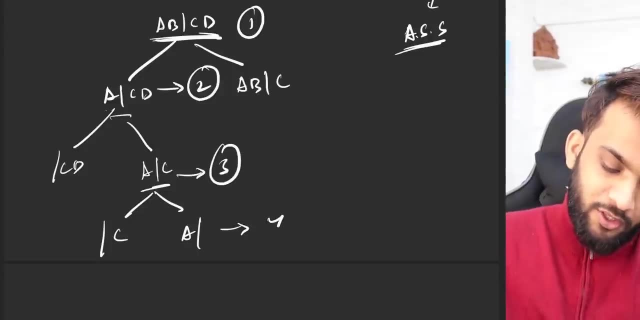 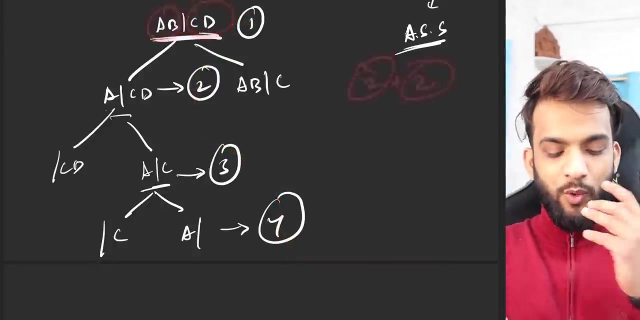 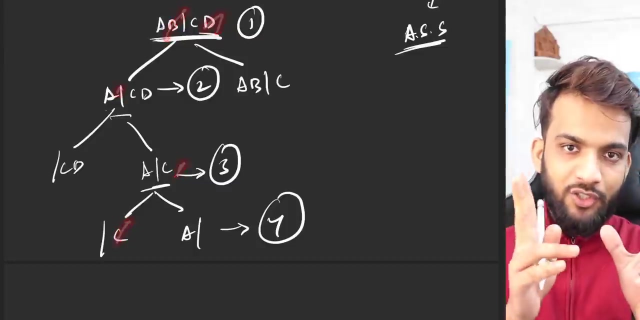 eliminate c. so if you carefully observe, one step, two, step three, step four, so at max the depth is four, length two plus length two, because what we did was we deleted v, we deleted d, we deleted c. so alternative deletions: if we do alternative deletions, there can be n deletions from string. 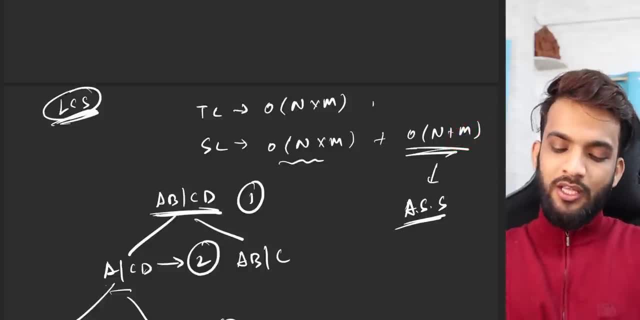 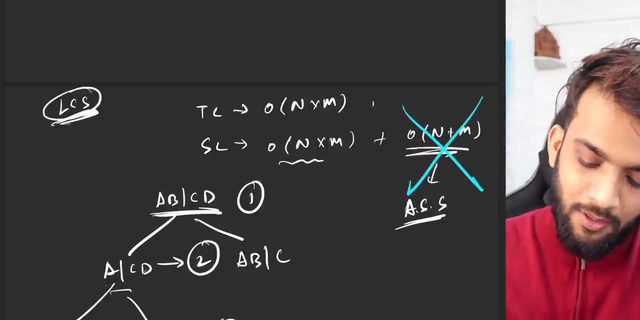 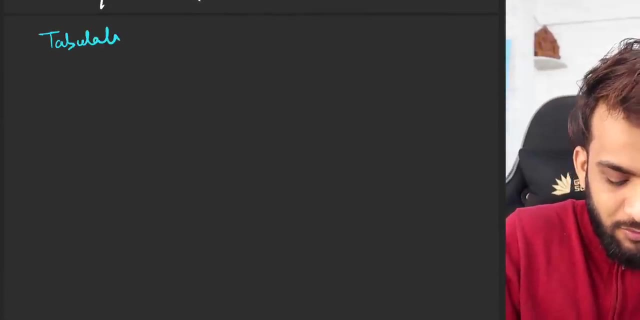 s1, there can be m deletions from string s2. thereby the auxiliary stack space will go as n plus m, but obviously, as always, i'm not a big fan of n plus m, so i'll have to omit this. in order to omit this, i have to write the tabulation: iterative bottom-up approach, whatever you can call it. 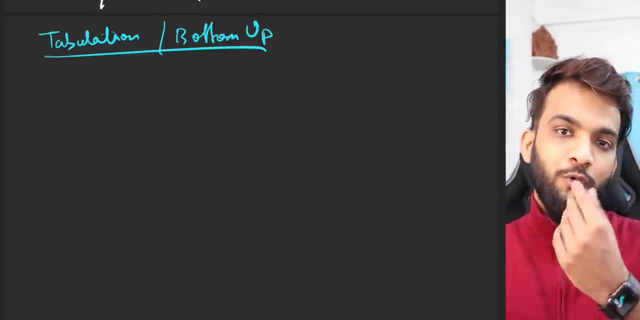 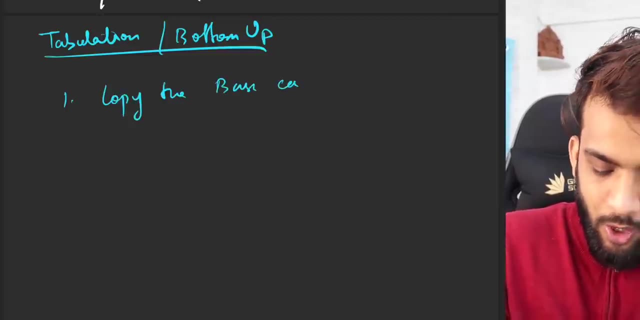 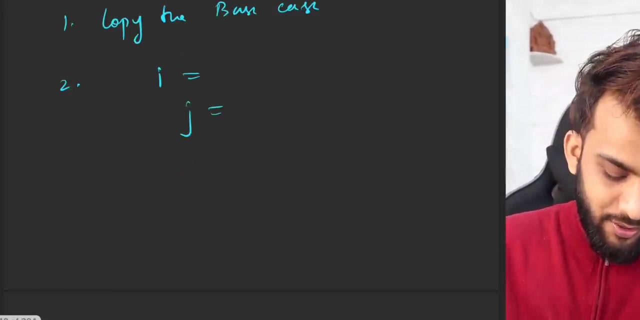 okay, so bottom-up rules. i've already told you what are the rules. copy the base case. i've already told you the rules. copy the base case. second, write down the changing parameters in the opposite fashion- perfect. third, copy the recurrence. if you can follow these method, i can. 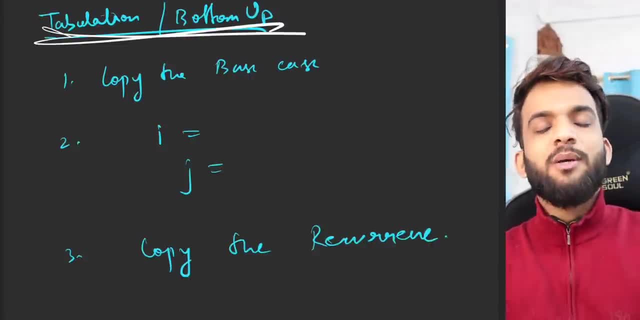 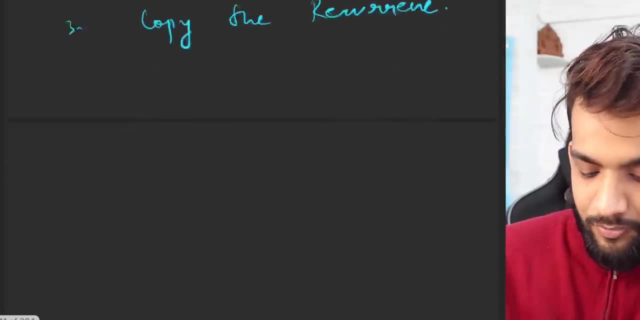 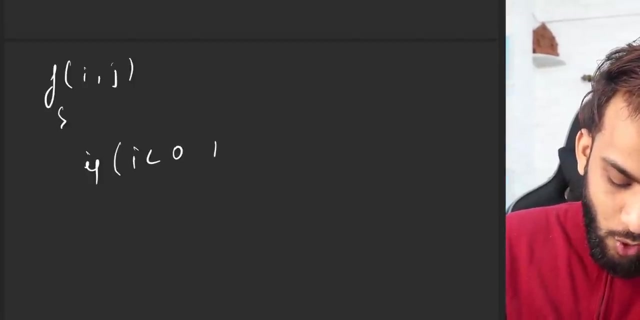 guarantee that you can write any of the tabulations or bottom-up for any of the questions, but copy the base case is a bit tricky over here. why? because if you remember the code, the code was i comma j and it was something like i less than zero or or j less than zero and you return zero. 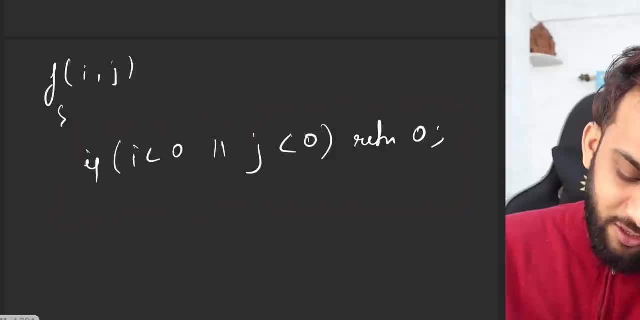 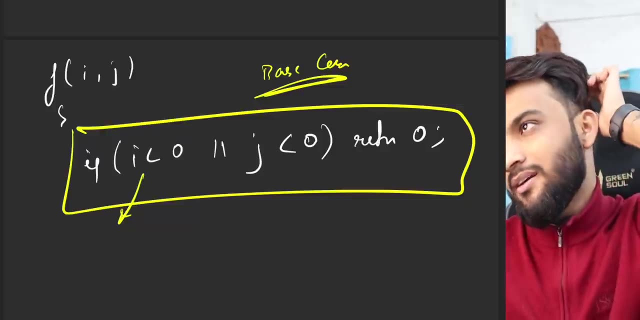 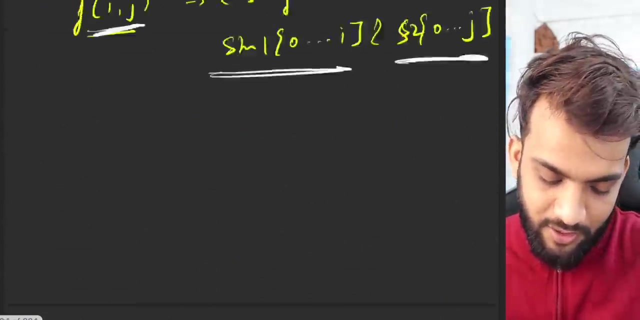 so over here, this was the base case, right, if you remember this was the base case, and in the base case i can be negative- and usually we did see, yes, usually we did see in the recursion tree. if you remember the recursion, they'll just stick it through the depression tree that we did in the recursion tree, the base, the. 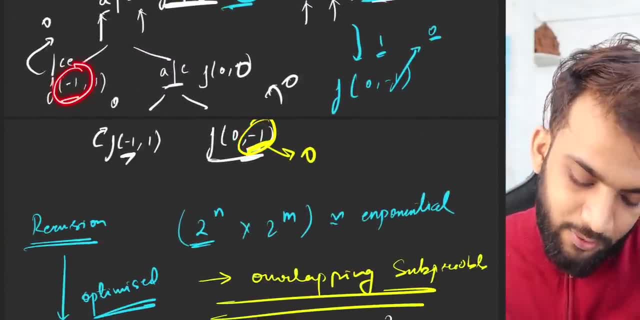 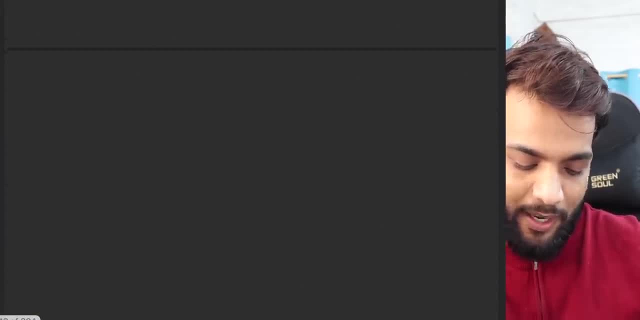 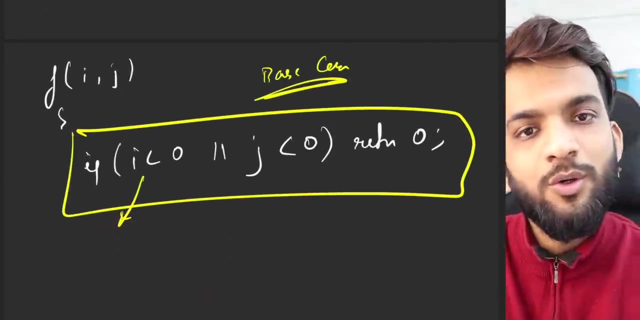 negative was minus 1 minus 1, minus 1. so we stopped at minus 1. so we can't. we can't write cases for minus one. in base cases can you write for minus one, because how do you write dp of minus one? that's not possible. that's not possible. so what we do is we 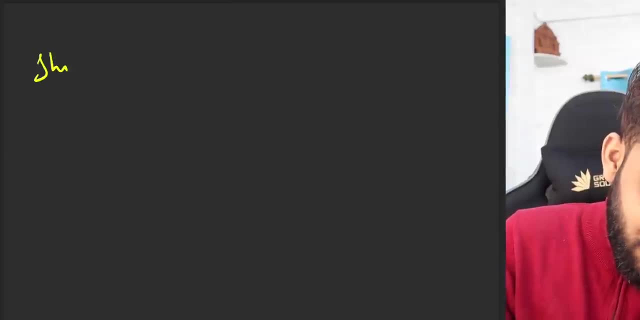 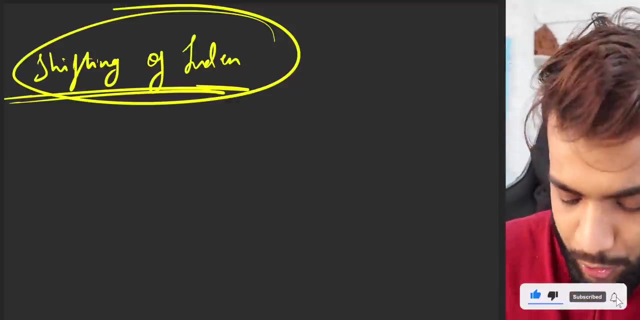 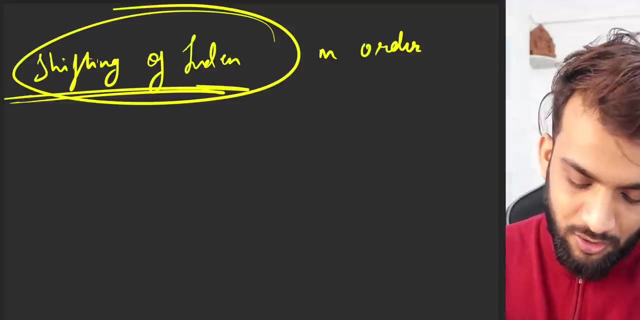 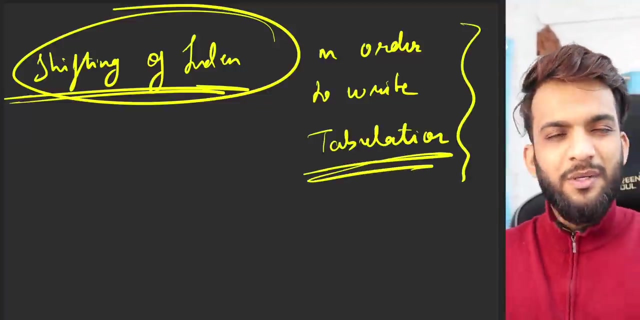 do a shifting of index. very simple: we do a shifting of index. we do a shifting of index in order to write tabulation. you can still write tabulation using this, but I want you to teach this shifting of index in order to write tabulation. like without even shifting of index, I can still write tabulation, but that will be. 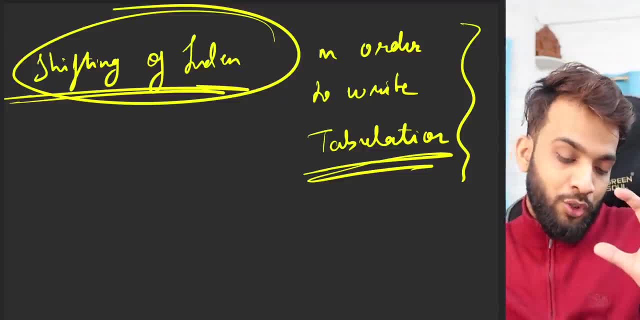 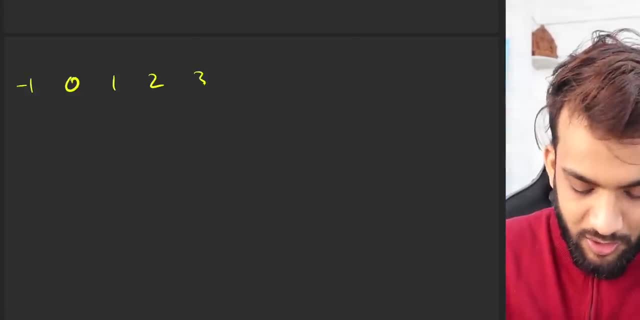 a bit tricky so I'll not go that direction. shifting of index. so as of now there was index 0, 1, 2, like minus 1 was the negative index, 3, till on n minus 1, and we were calling these indexes like: how did the function start the function? 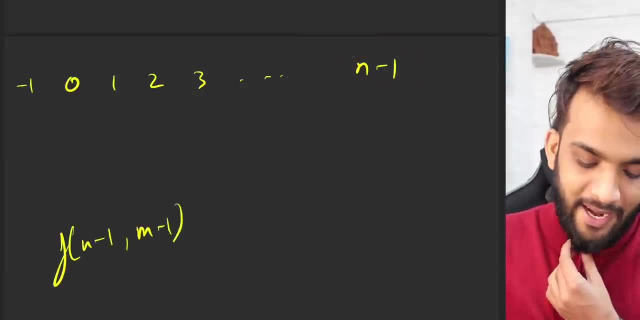 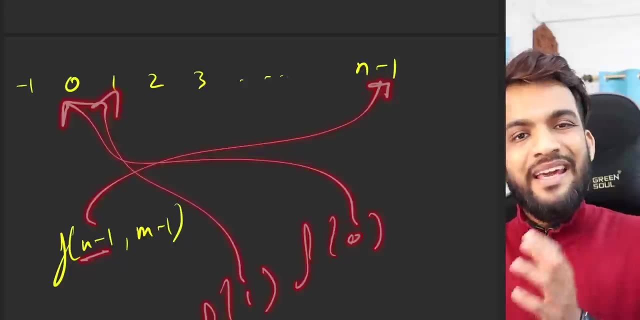 call started from n minus 1 at m minus 1 and n minus 1 represented this index. f of 0 represent this index. f of 1 represents this index. can I do a shifting? can I do a right shift of the index? and I see. 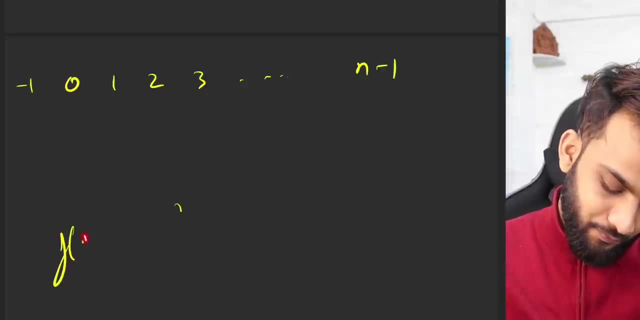 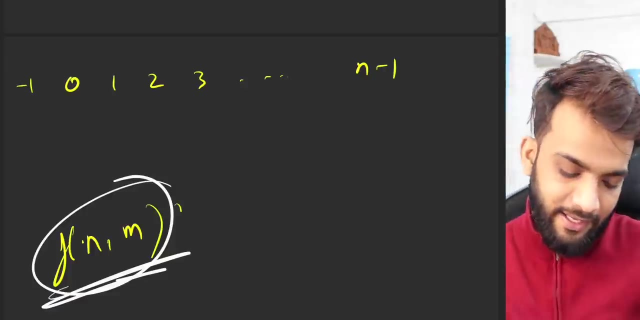 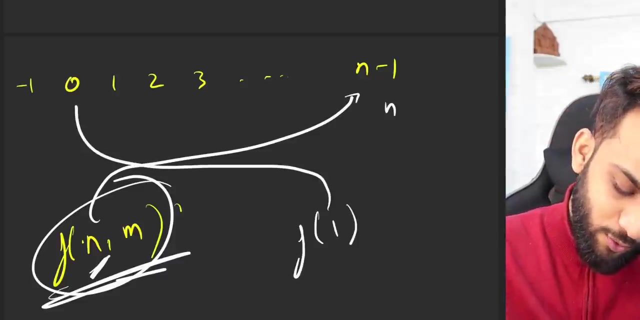 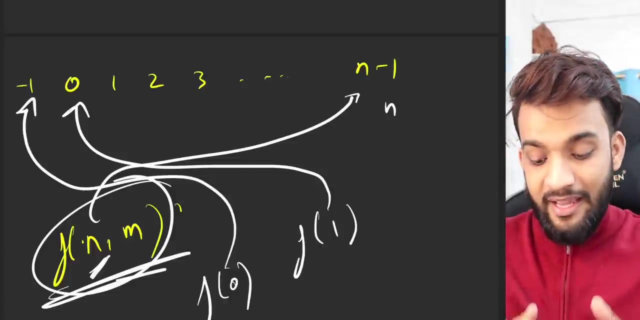 I see I will call n comma n. I will call n comma n. yes, I'll call this, but over here I'll say: hey, listen, n means n minus 1. okay, f of 1 means 0 and f of 0 means negative. I shifted the index one right, one right. n means n minus 1, 1 means 0- 0. 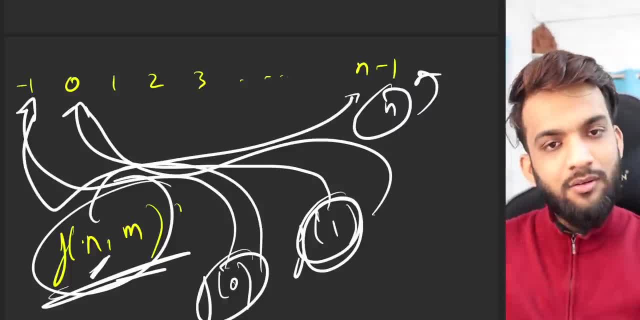 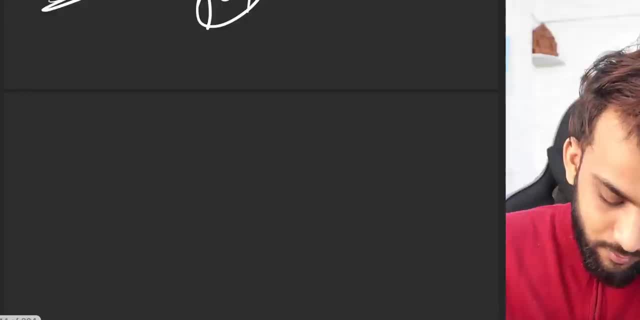 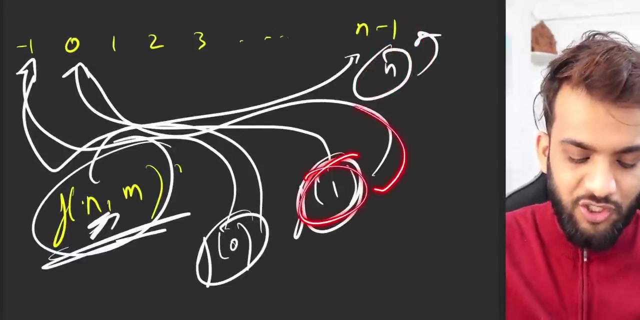 means minus 1. I shifted it one right. okay, makes sense. so we're shifting it one right. if so, can I say f of ij. if you've shifted IJ, like initially i is n and j, initially i is n and j is n, you shifted it. n is actually n minus 1, 1 is actually 0. so can I say: 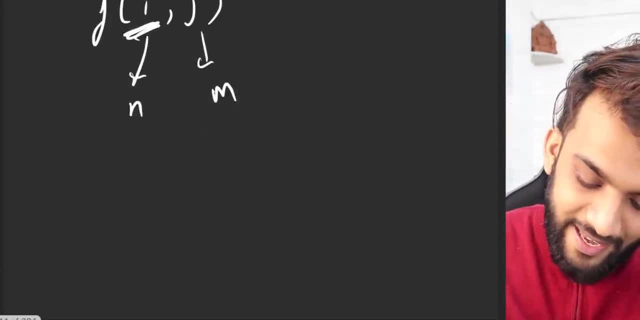 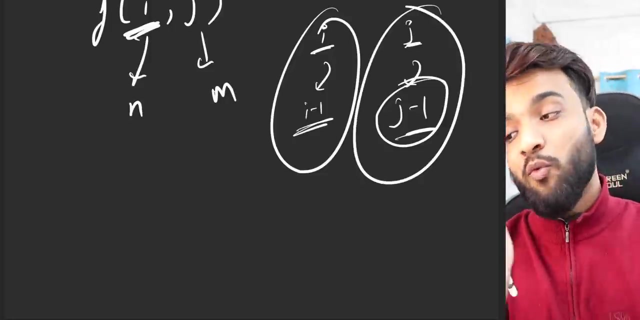 can I see that means every I that you're giving should be treated as I minus 1 and every G that you're giving should be treated as J minus 1, because that is the meaning. because, as of me, you're sending I and J in terms of one shifted index I. 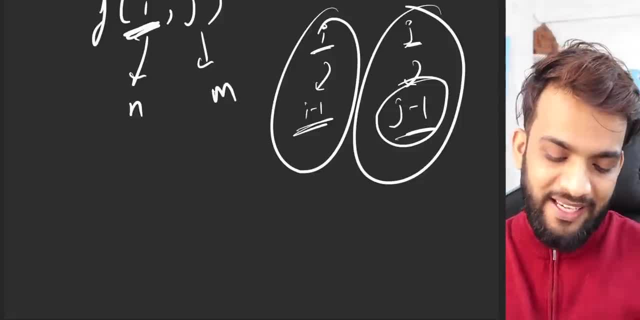 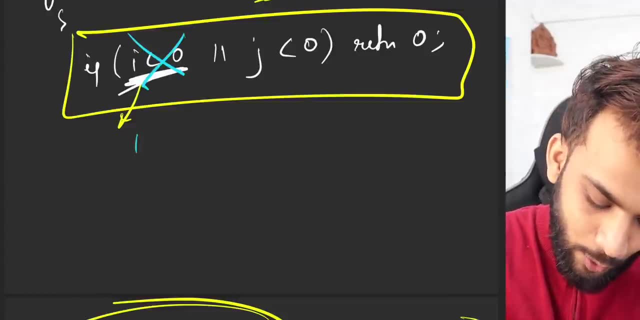 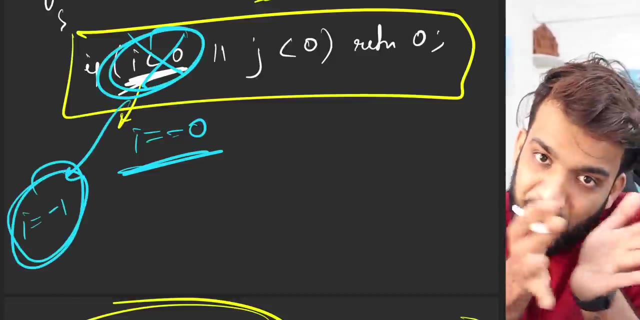 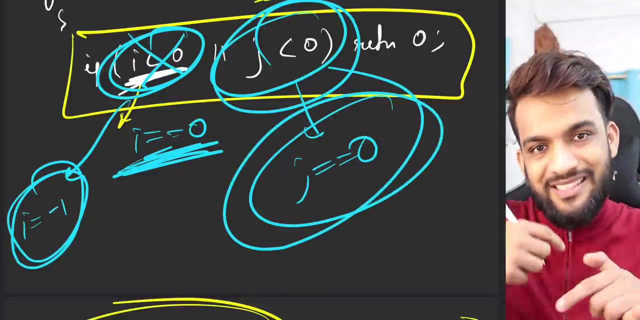 like does make sense, does make sense. so can I say instead of greater than 0, can I write this as I equal to equal to zero, because this signified i equal to minus one, but since i've shifted it, can i write: i equal to zero? yes, and can i write instead of this j equal to equal to zero? i can? the base case has been changed. 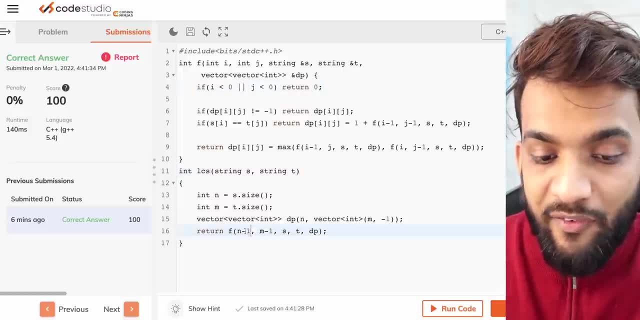 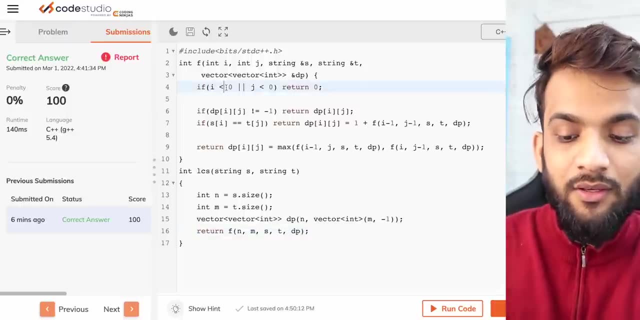 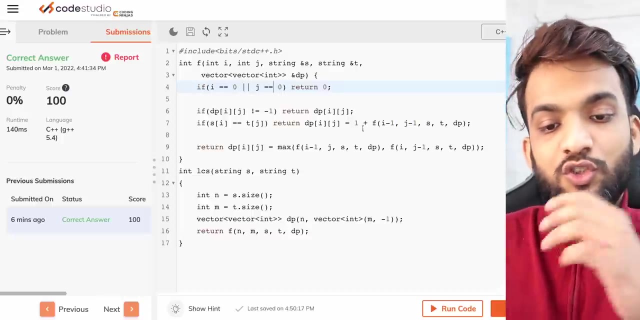 if i take you back to the code: over here, instead of n minus one, i can write n. m minus one i can write m, and over here i can write equal to equal to, and in the j also, i can write equal to equal to. but what's the other changes? everything stays same, states being called same. you're doing a. 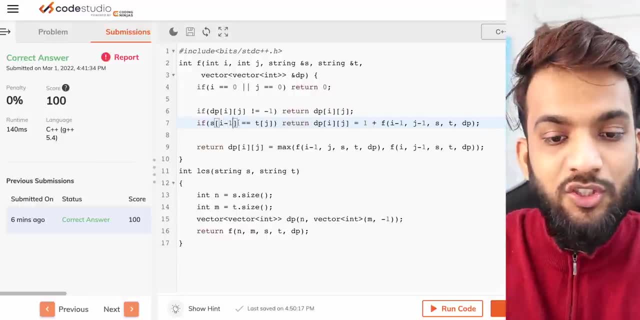 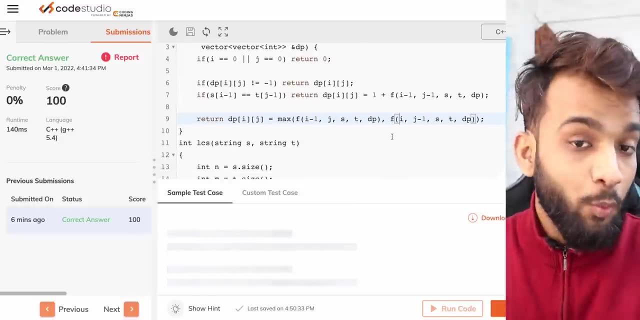 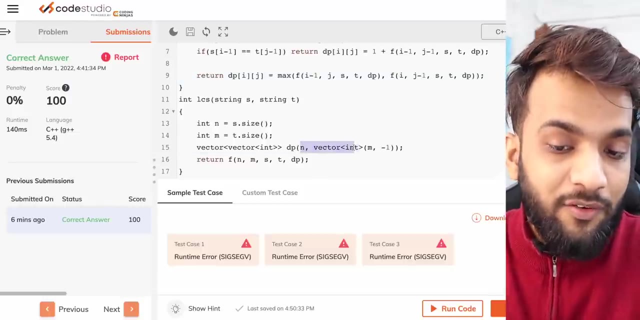 string comparison. but i means i minus one, j means j minus one changed. and now if i run this code, does this run same? it will. why will it? because you've just shifted it, okay, it's giving runtime error. Why give runtime error? because the dp that you've declared is of n- m and you are now using the. 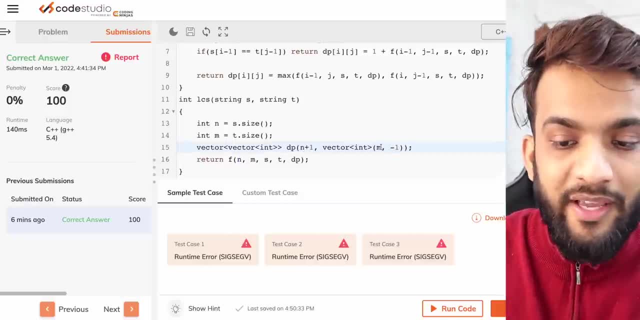 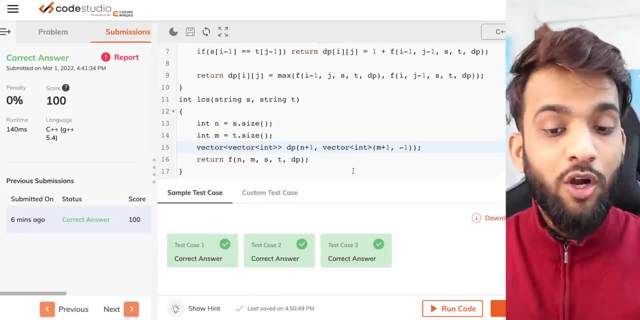 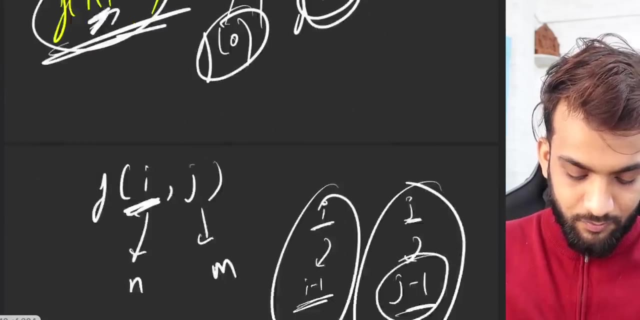 states of nm. so just make sure you declare a dp of extra size, m plus one. and now you've done a shifting of index, one right, and it does work fine. so okay, so the base case has been, now the base case has changed. what's the base case now? the base case is now very simple. it states: if i is equal, 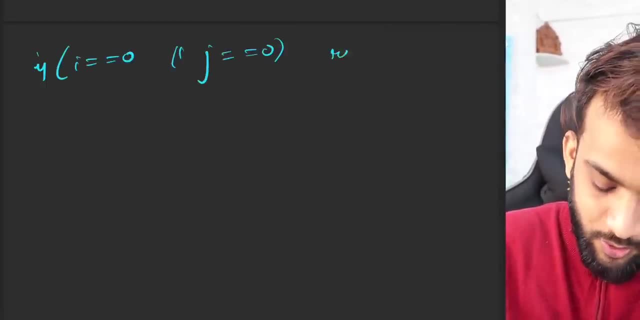 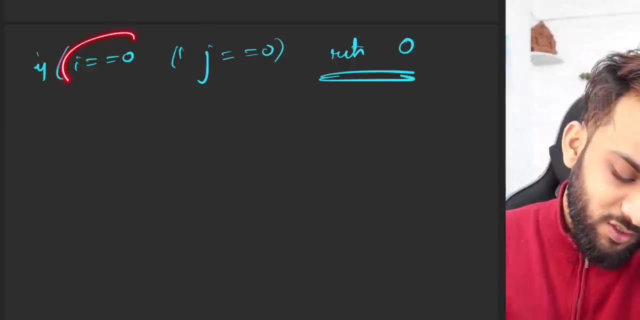 to equal to 0, or j is equal to equal to 0, we are returning 0.. how can i write this in simple, layman terms? okay, what does i? equal to 0 means? it means any dp of 0, and this guy can be anything. 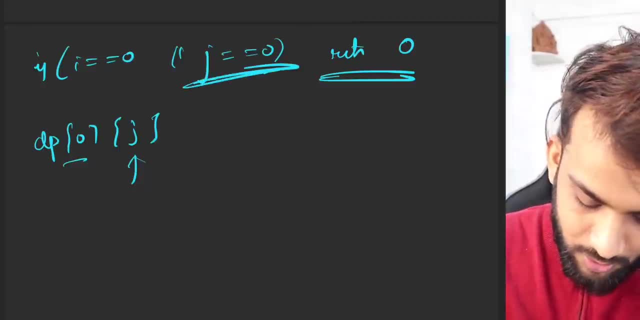 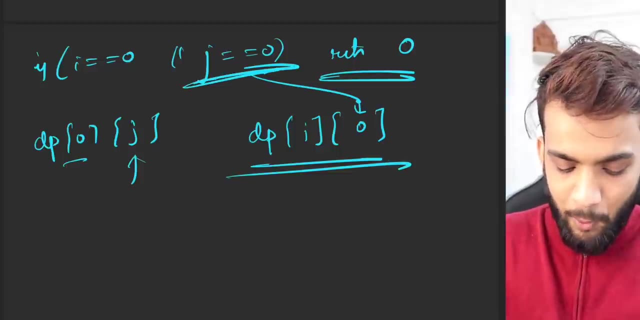 because this is j. j can be anything. and what does this mean? i can be anything, but this guy has to be 0 right. and what can be the possible values of j? anything from 0 to m minus 1. what? What can be the possible values of i? 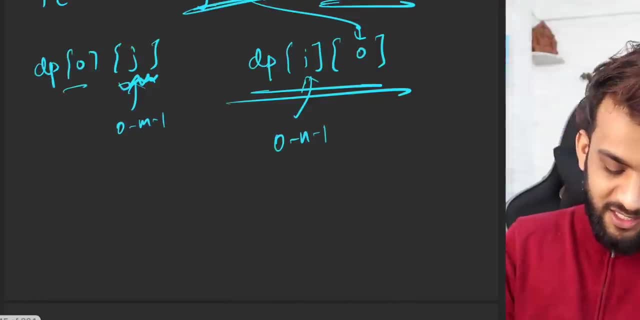 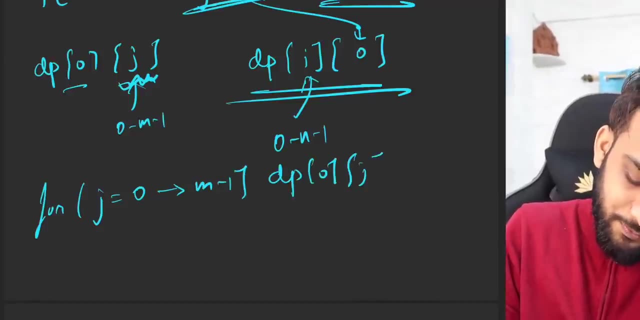 Anything from 0 to n minus 1.. Loop it. The base case are very simple. j can be anything from 0 to n minus 1.. And dp of 0 and j will be 0. This is for this one. 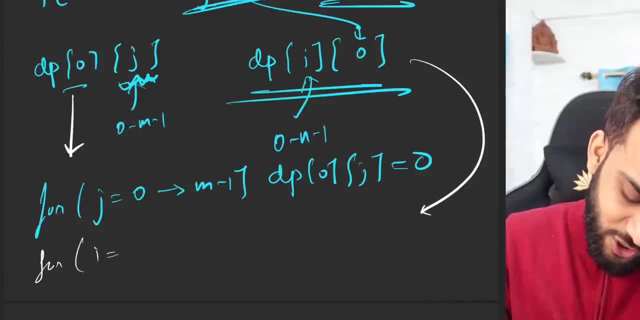 And for this one is this: i can be anything from 0 to n minus 1. And dp of i comma 0 is equal to 0. Base case written by shifting indexes by 1. And base case has been written Perfect. 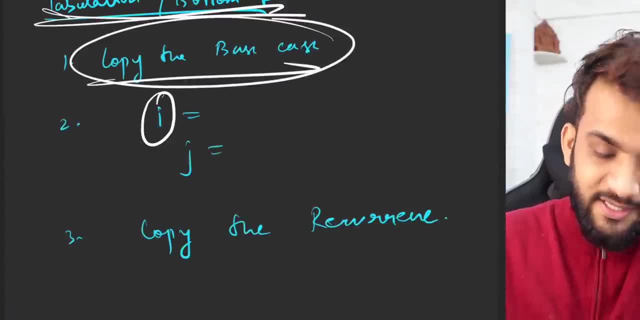 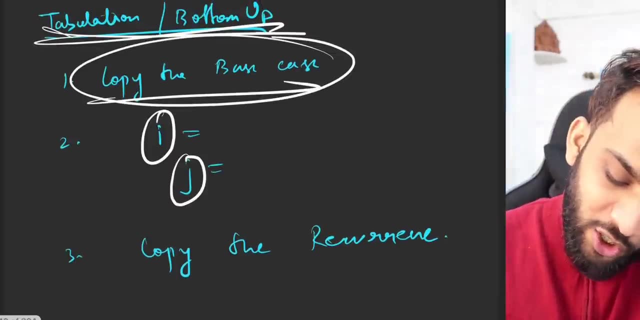 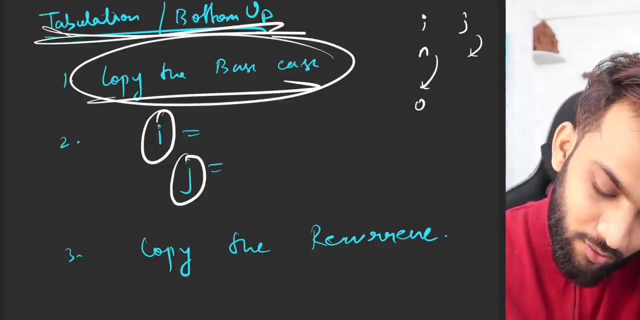 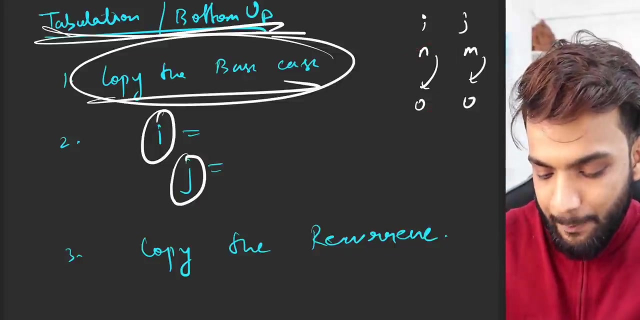 What's next? Write down both these guys in opposite fashion. In opposite fashion. So the moment I shifted it, The recursion was taking i from n to 0. And j from m to 0.. Top down, Top down. These are the base cases. 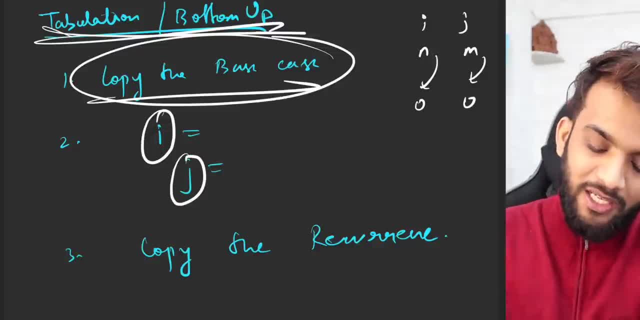 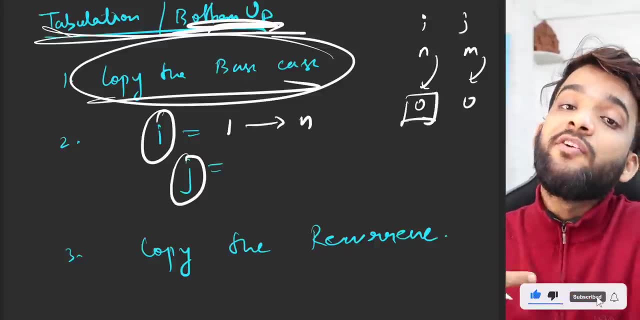 What is tabulation? bottom up You go up. So 1 to n. Why not 0 to n? Because 0 is the base case which has already been written. So 1 to n. What about j Opposite? 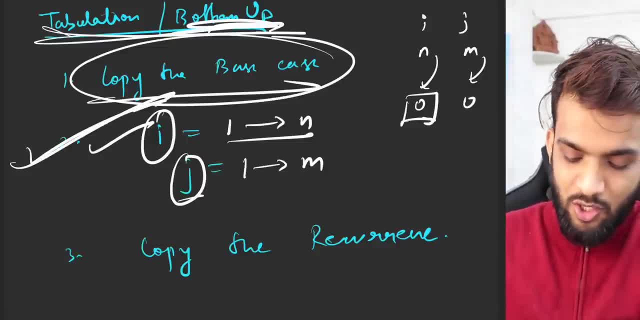 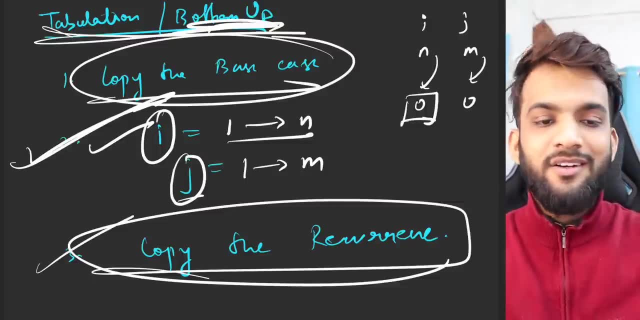 Done, Next Copy the recurrence. What are you waiting for? Just go back and copy the recurrence And you'll be able to easily write the tabulation format of LCS easily. So what I'll do is I'll go back and try to write the tabulation format. 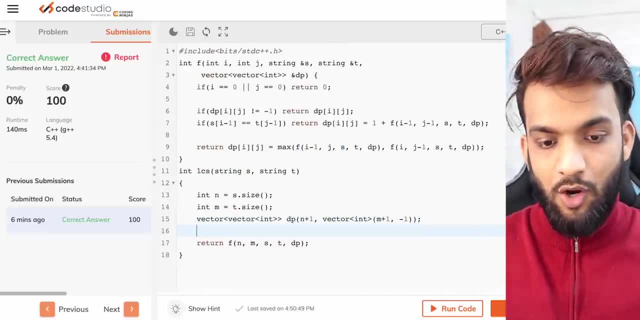 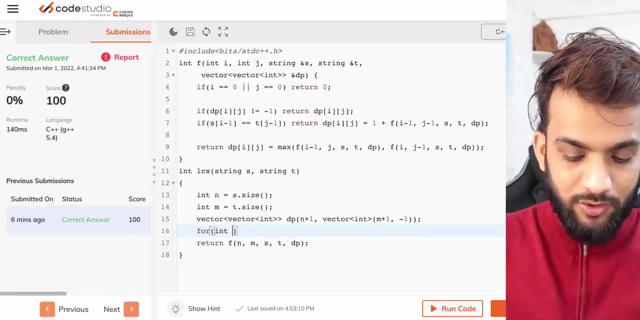 Okay, So we have this guy. That's perfect. Let's just omit this and try to write this. So, if you remember, it was i equal to 0.. Or rather, yeah, j equal to 0 was the first one. 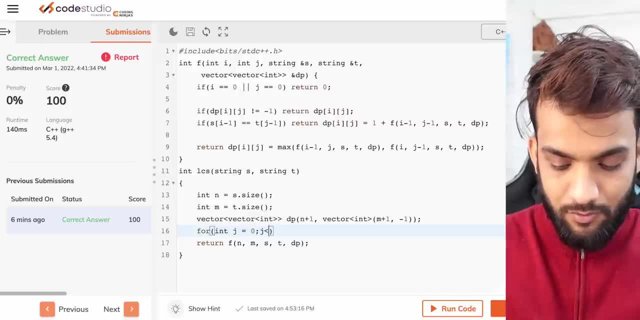 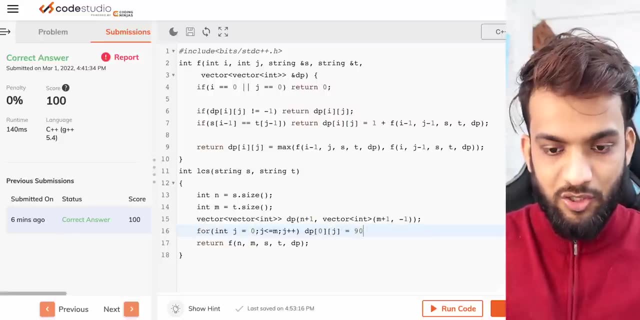 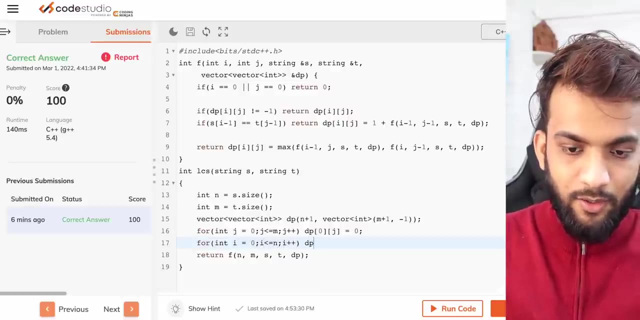 j equal to 0 and j lesser than m, But then now it will go j, this dp of 0. And j is 0. Perfect. And similarly i can go as 0 till n And it can go as dp of i. 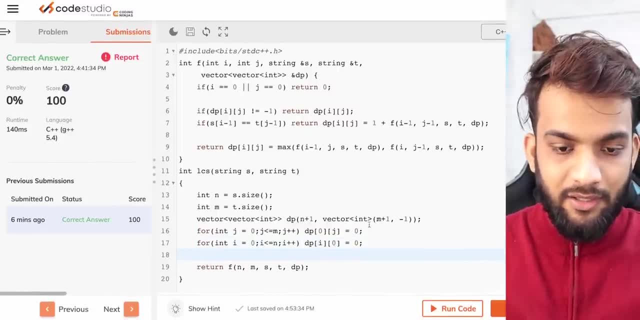 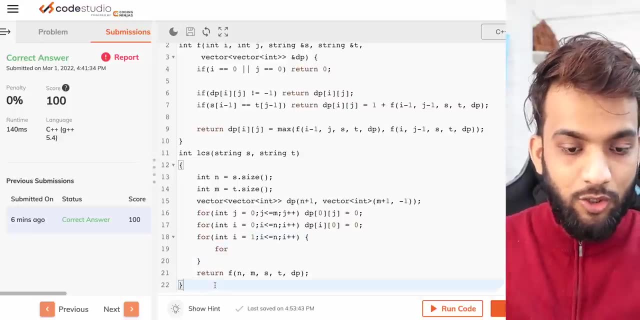 And 0 as 0. Perfect. And similarly for loops can go as: int. i equal to 1, i lesser than or equal to n. i plus plus. Similarly, the j loop can also go on in a similar fashion of int. j equal to 1, j lesser than or equal to m, j plus plus. 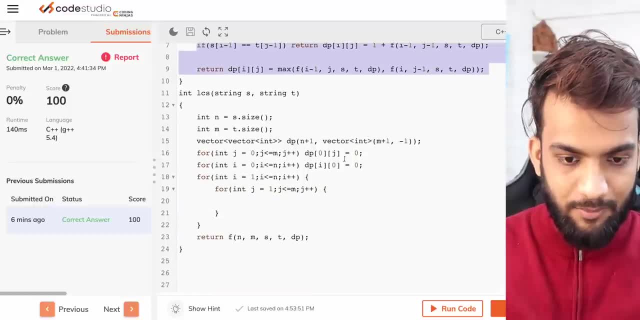 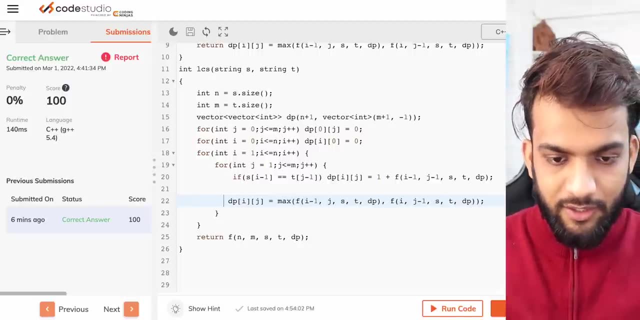 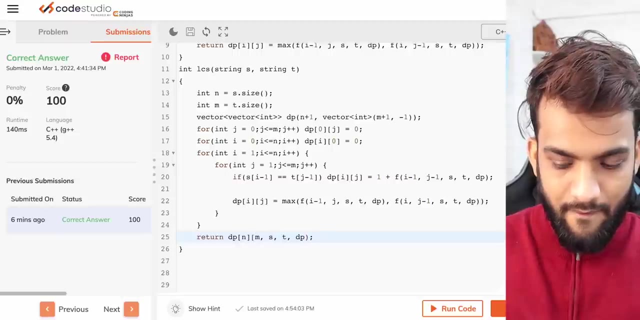 And you can just copy paste. Yes, Just make sure you copy paste the same thing, Just instead of written. just remove written. Yeah, Just remove written And just copy paste the same thing, Exactly same, And over here, just return. dp of n and m. 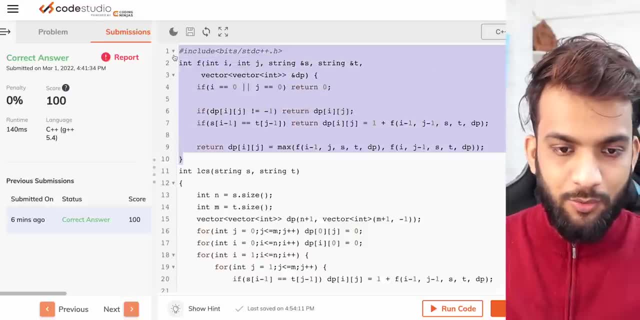 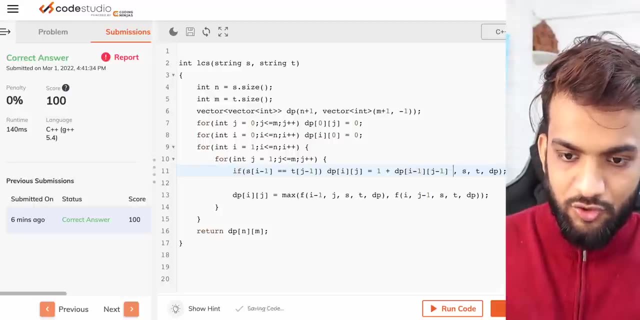 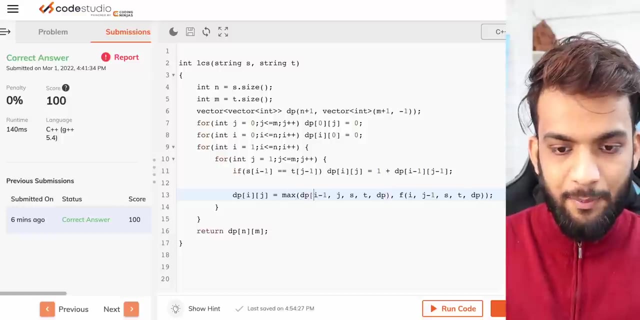 And remove this. And what you can do is you can also remove this portion And instead of f, just make sure you write dp of i minus 1, j. Perfect, And over here you can write max of dp of i minus 1, j. 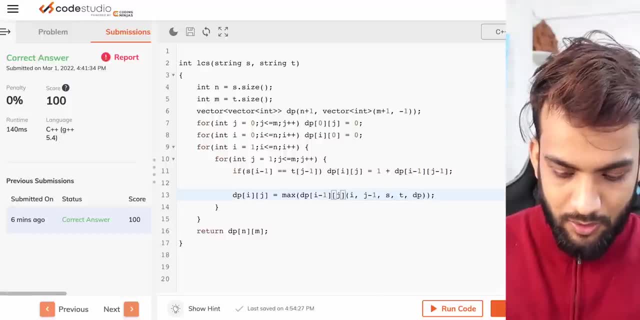 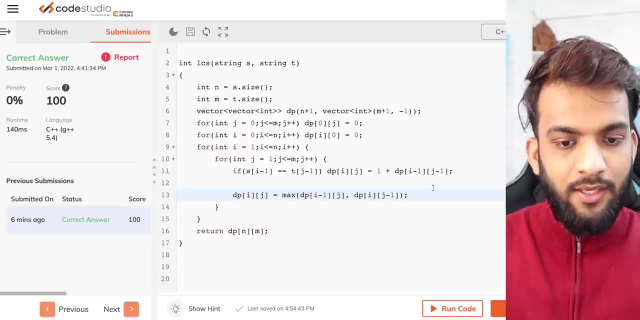 And again, you can just remove this, So you can remove this portion and the comma of dp of i and j minus 1.. And again, please make sure you remove this. Yeah, That's what it will be. So if I now try to run, this probably should run. 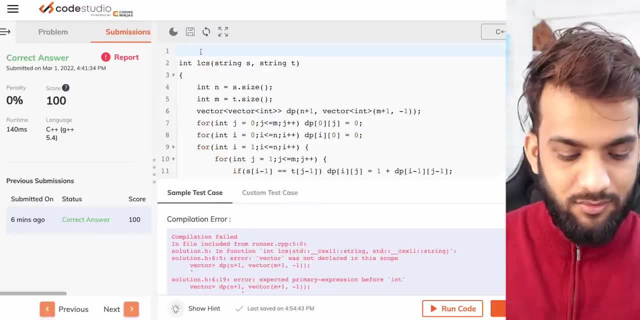 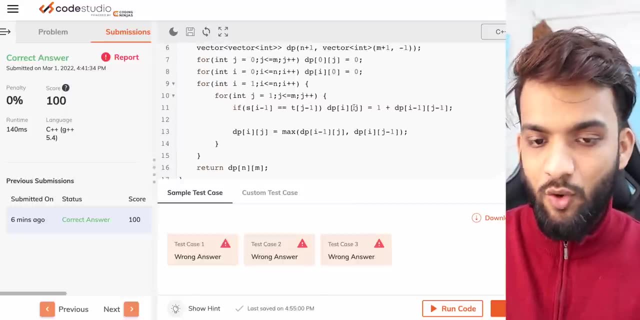 If I've not done syntax mistakes. again the hashing load missing. Again it's giving us a wrong answer. Why is that? So you can check out. why is this giving us a wrong answer and then we'll get started. So why did this give us a wrong answer? 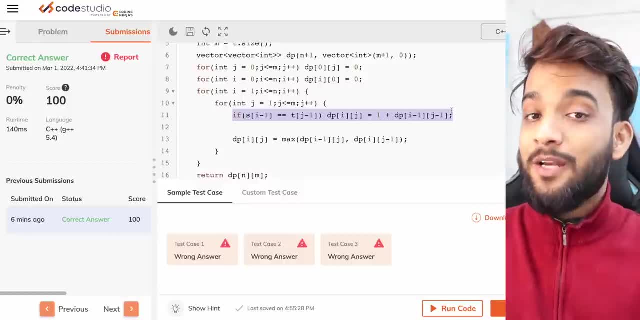 Why did this give us a wrong answer? Why did this give us a wrong answer? Because in the recursion, if this, if executed, it went back from there Over here, you have to just make sure you write an else. Okay, Just make sure you write an else, because it will not return. 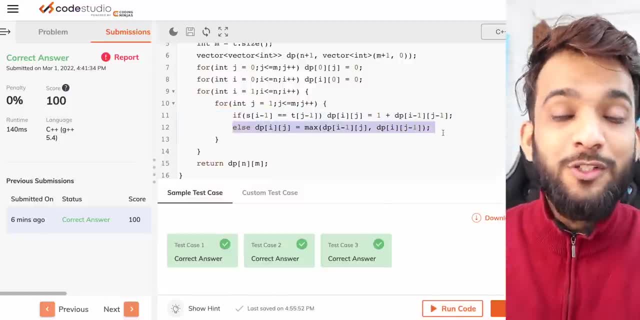 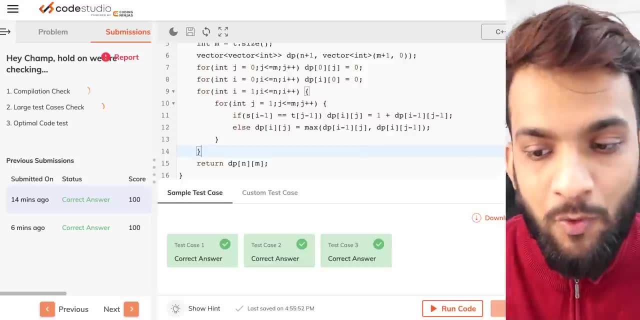 In recursion. this line was not executed In for loops. it will be so Just make sure either it is matching or not matching. It is running fine Now you can just go across and submit. So can we do a space optimizations? 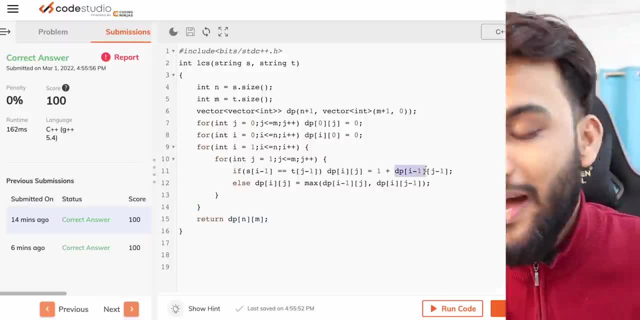 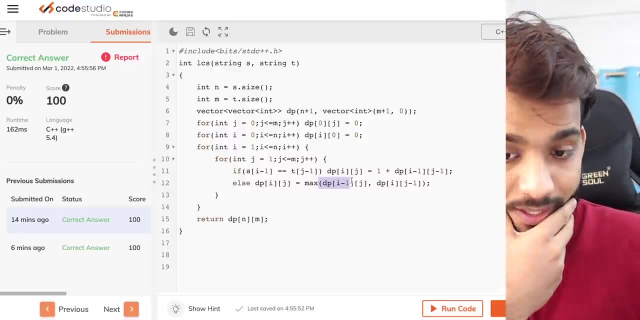 Yes, I have always told you, if there is a scope of i minus 1,, which means previous row, Okay, i minus 1,, which means previous row, You can always- I repeat, you can always space optimize the same portion. 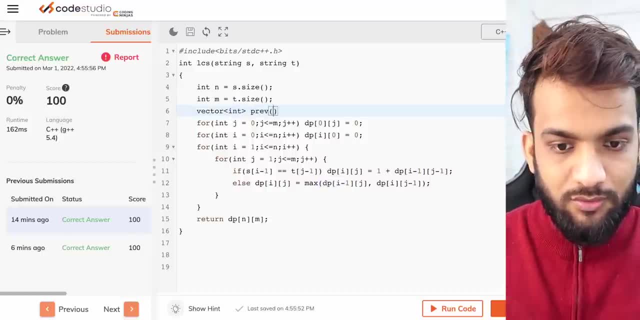 So what you'll do is, instead of this, just make sure you have a previous of m plus 1 comma 0 and a curve of m plus 1 comma 0. Perfect, And over here this will go, as this is the 0th guy. 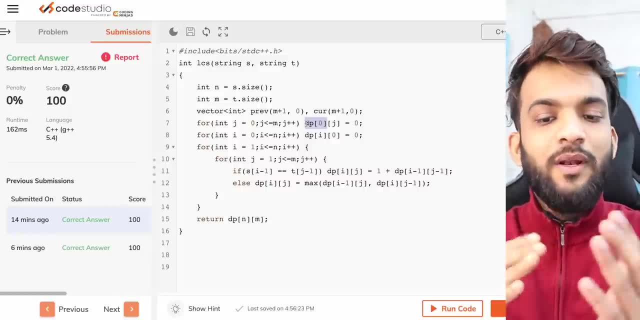 So what I'm basically saying is: okay for any 0,. what will happen? So this is dp of 0, right, So you can say previous: And will this be there? Will the column be there? No, there's no need of column. 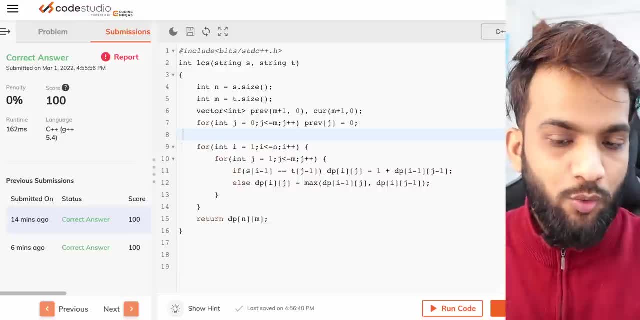 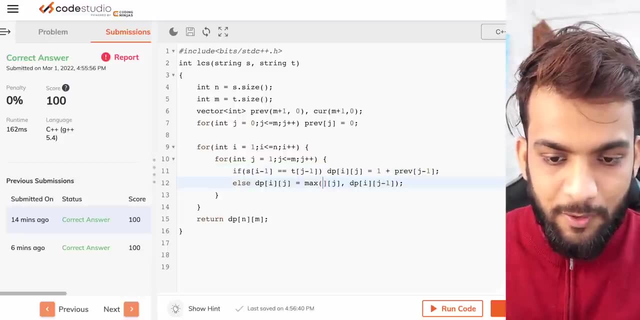 So you can just omit this. For the first row, every 1 is 0, right, So that's what you have done Over here. just make sure: instead of dp of i minus 1, that's previous Over here. just make sure: instead of dp of i minus 1, it's previous. 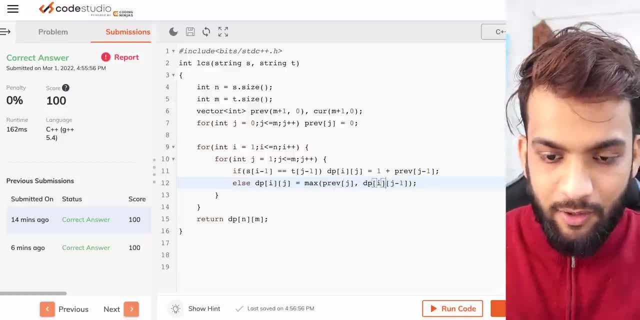 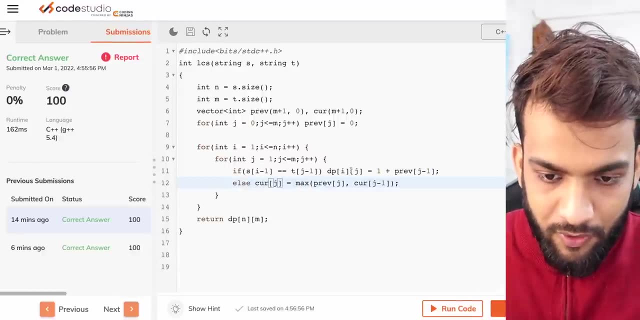 Over here, this is fine. Instead of dp, it will be curve. dp of i, it will be curve. Just make sure it is curve. And over here, instead of dp of i, this will be curve. Instead of dp of i, this will be curve. 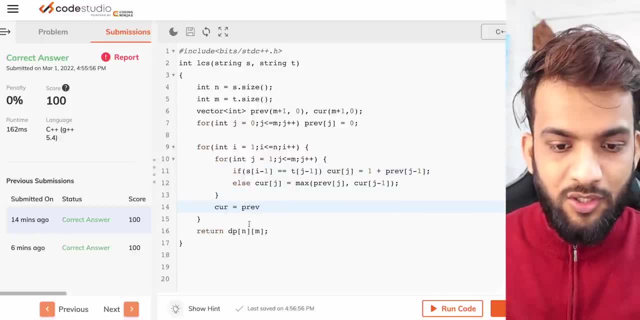 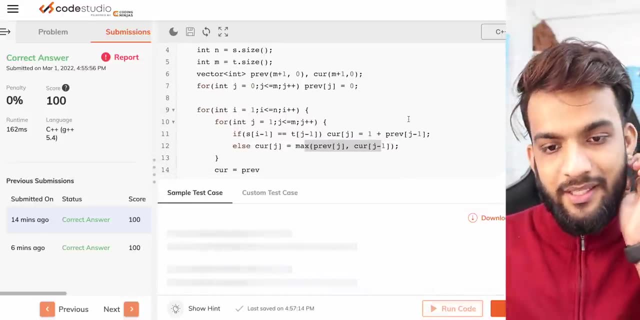 Perfect And just right. after this you will do curve equal to previous And over here you will just return the previous guy Or curve, whatever you wish to. Is this fine? Yeah, this should look fine. So now you can try submitting this. 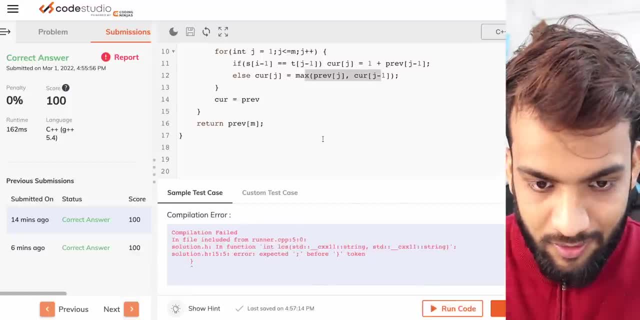 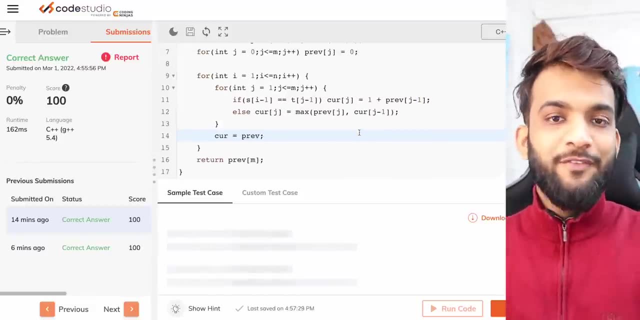 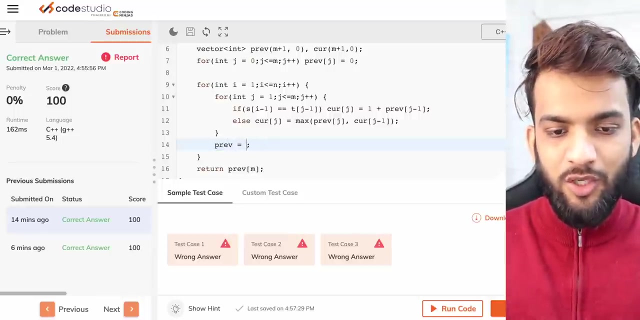 And you will see that this is also not running fine. Why, Okay, forgot to have a colon. So if I give a colon, just previous column, previous curve concept And okay, okay, Okay, so the issue was previous equal to curve will be here, not curve equal to previous. 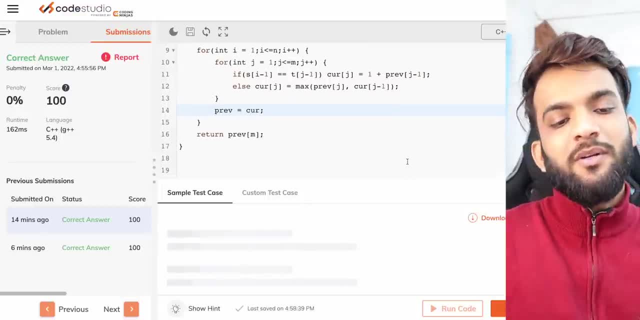 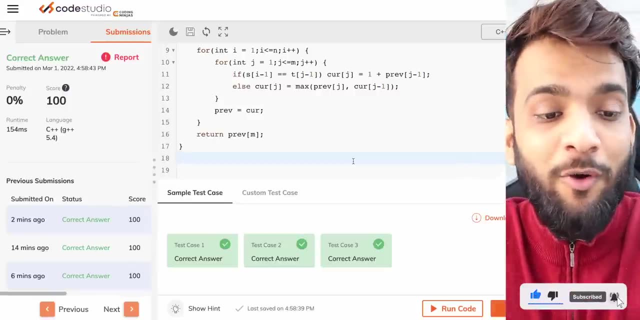 My bad. Okay, so if I just give it a submit, it should be running. fine, now, Yeah, it should run. If I give it a submit, this will definitely run. So, guys, I hope you have understood how I took a memoization solution. 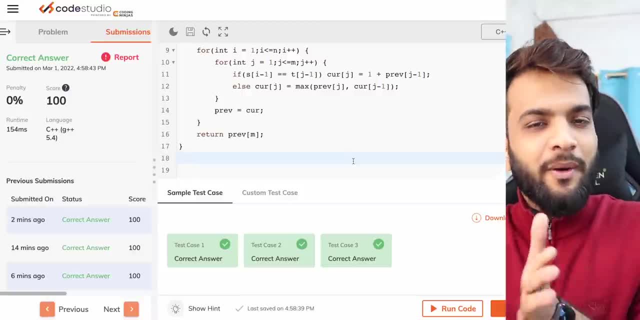 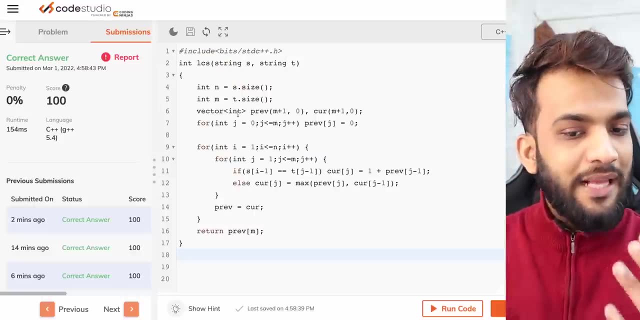 And since we were having problem in tabulation, I shifted it by right so that we do not have negative integers or negative indexes in base cases, And after that I just simply converted that into a tabulated. Once I converted that into tabulated, the space optimization is an extension of whatever I have taught in the previous dp lectures.